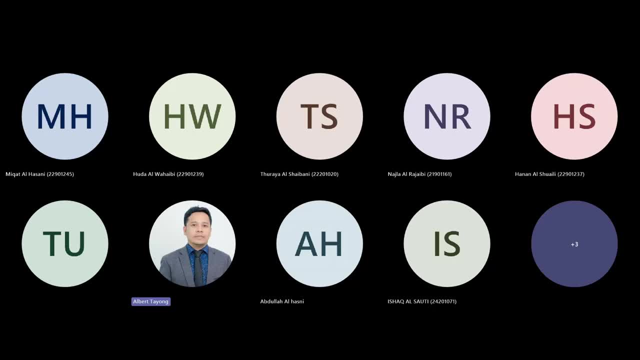 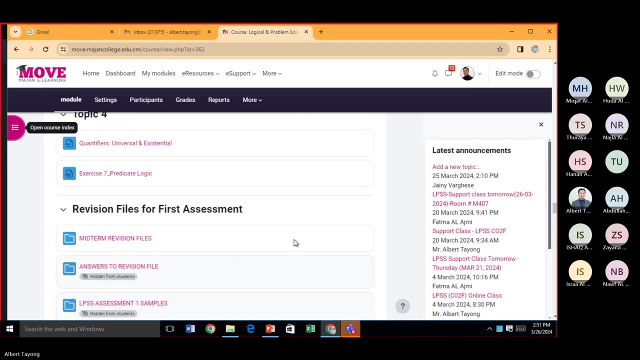 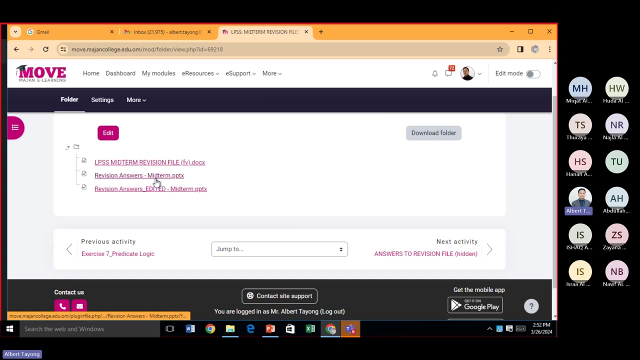 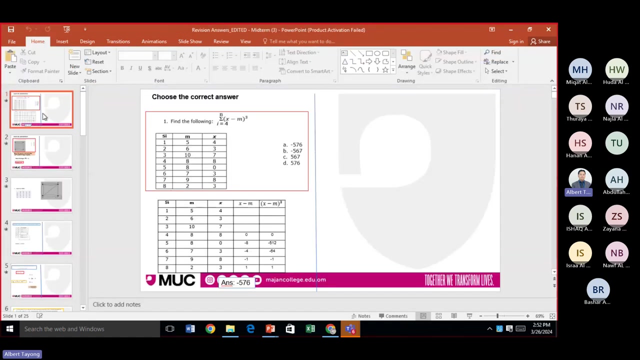 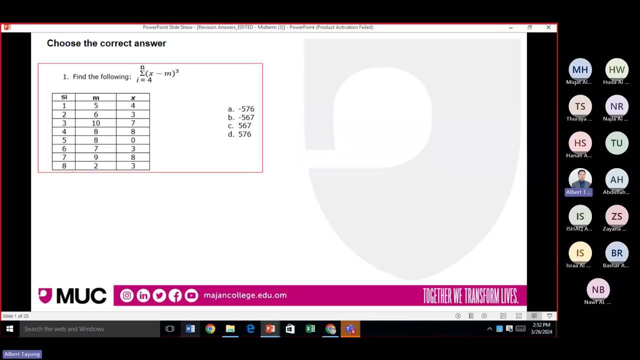 Okay, so the revision file is, of course, in the move page here, The first file. you can see the midterm revision files. This is what we're going to use. The answers are there already. These are the questions. Okay, so let me answer this one by one. Thursday we're going to have a support class again, From 245 to 515.. That will be our last class before your exam, Because next week, next week, No, this Thursday, Okay, Next week is your exam. 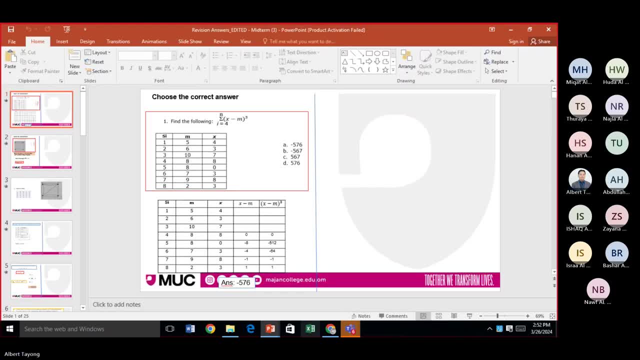 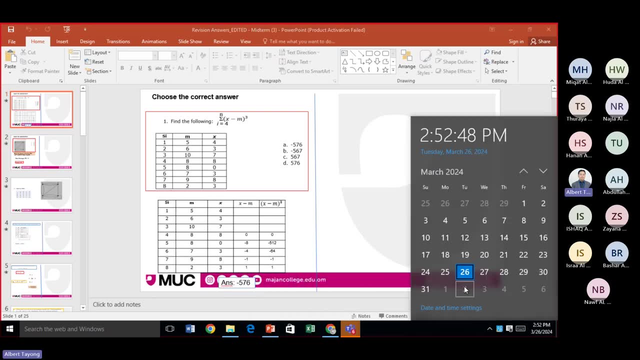 Right, So next week we don't have a class Because this is assessment week. April two: no class. So our last class will be on Thursday, March 28.. After tomorrow, So the same time, 245 to 515.. That will be our last class. 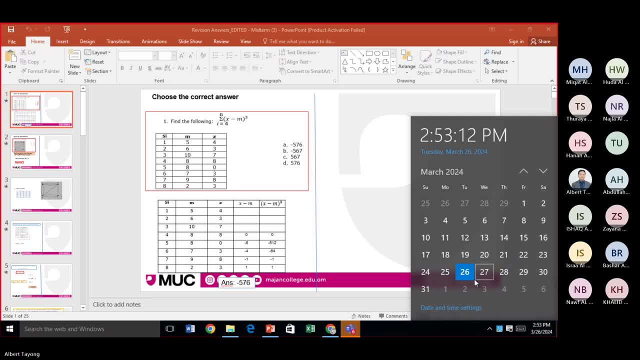 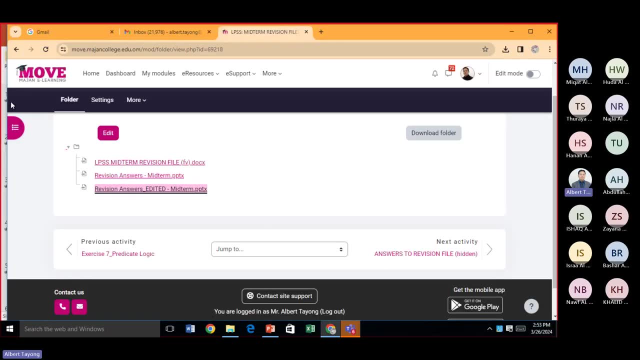 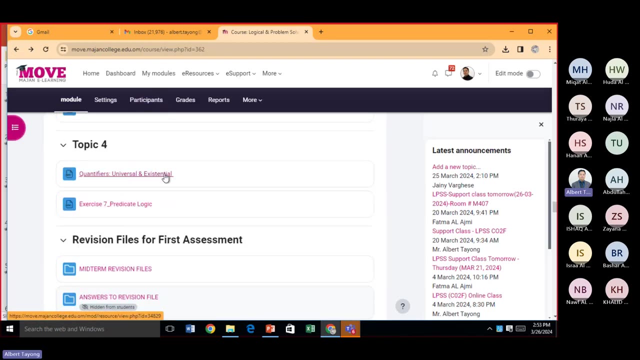 So for this I'm going to focus on the remaining of the revision Plus, I'm going to discuss the again. the last topic 25,, universal and existential, Although I sent you the recording of this already last time, but I will again rediscuss this on Thursday. 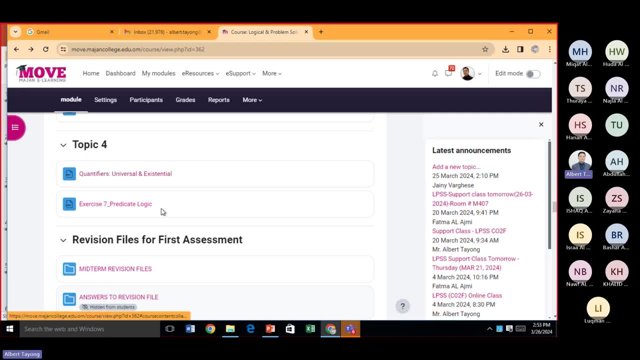 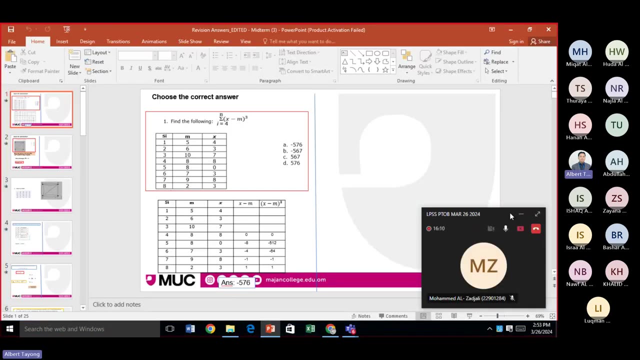 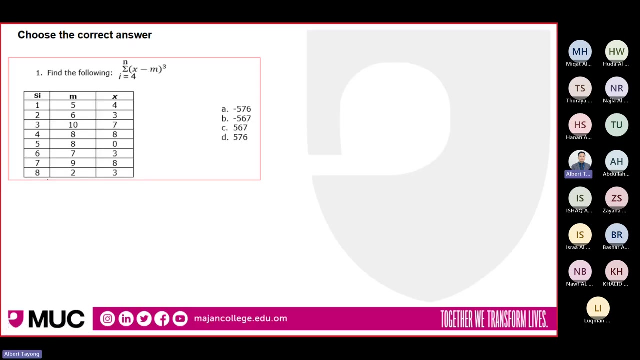 Plus the remaining of the revision. meaning of the revision: okay, so please attend a support class on Thursday. that will be our last class before your exam, so let's do this one by one. number one is all about the summation, so please look at where is the starting. 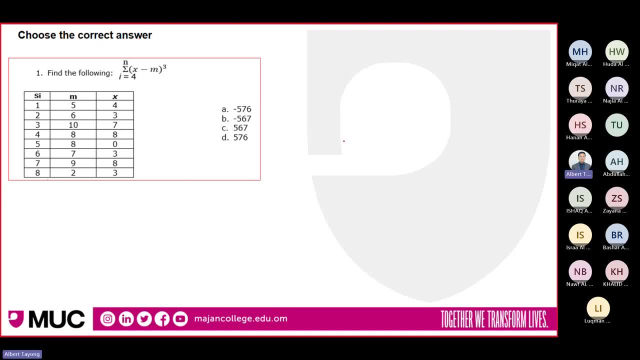 point. the starting point is the fourth and the ending point is the stopping point. n means the last. okay, all right, so it means we are going to start from here until eight. okay, we will not be including one, two and three. we will start with a fourth and you're going to get the sum of the quantity of X minus m raised to the. 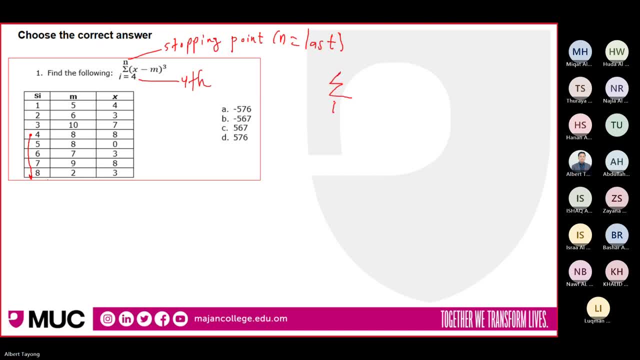 power of three. so I equals four until n where we have the course. so that means we have to put the sum of the quantity of x minus X minus m cube. so this means we're going to add cubes here. be careful, we're going to start from X, not from M. 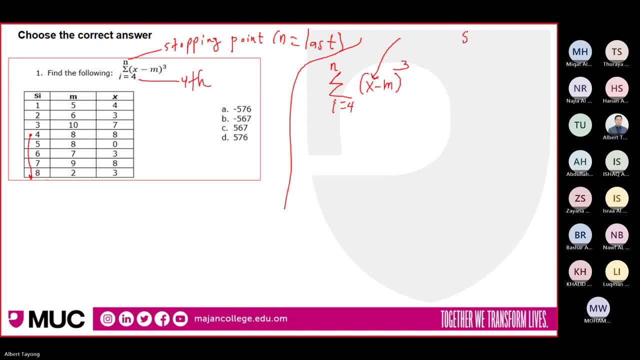 because subtraction is not commutative. five minus two is not equal to two minus five. okay, so in subtraction we have to be careful. in addition, there is no problem, we can change the order. it will have the same answer. so this will be equals 8 minus 8 cube. 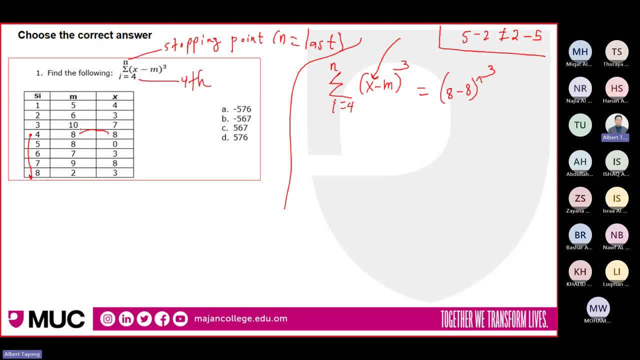 we start with 8 x minus m, then 0 minus 8, so plus 0 minus 8 cube. okay, plus. we keep on adding because of the summation: okay plus 3 minus 7 q. plus 8 minus 9 cube. plus 3 minus 2 cube. 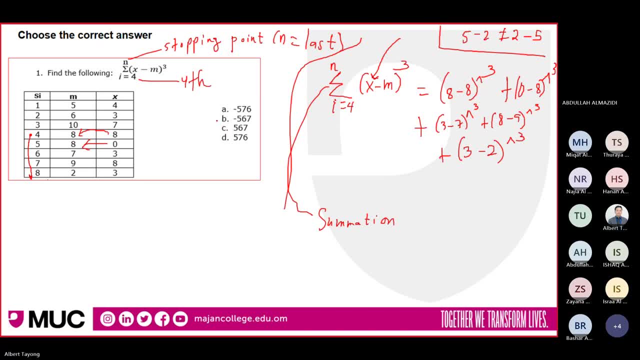 okay. so what is the answer? this is a multiple choice question. you have to encircle only the correct answer in your exam. so what is the answer here? negative 500, 76. so you have to encircle a guys. do you have any question here? no, mister, so easy, was so easy, mashallah okay. 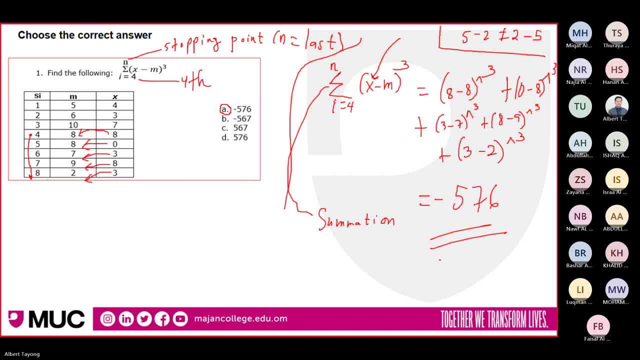 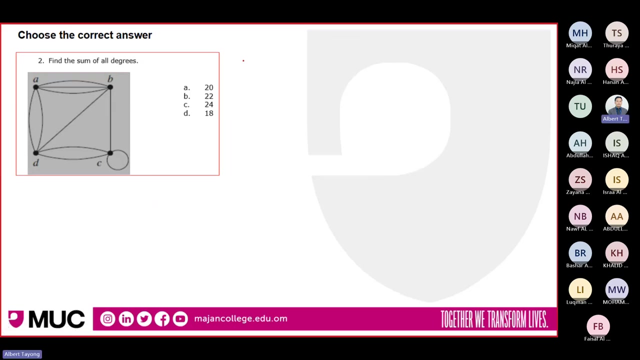 yeah, face now. yes, yeah, F F T Z F F F F Z Z 500 1 1, 2, 1 9. 1 2 3. 1 1 6, 4, 5, 3, 5, 6, 5. 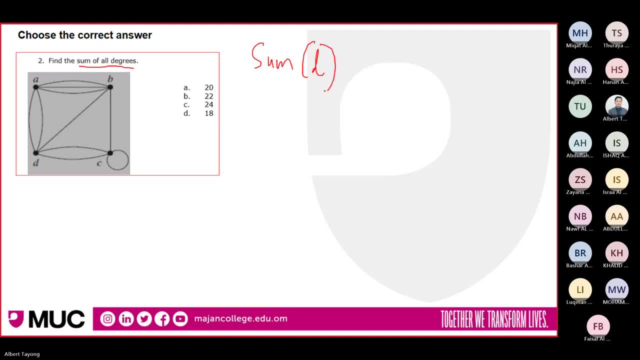 The sum of all degrees is equal to 2m, where m equals number of edges. So you have to count. You can label in the exam to avoid confusion. You can have this as E1, E2,, E3,, E4,, E5,, E6,, E7,, E8,, E9, and the loop is E10., 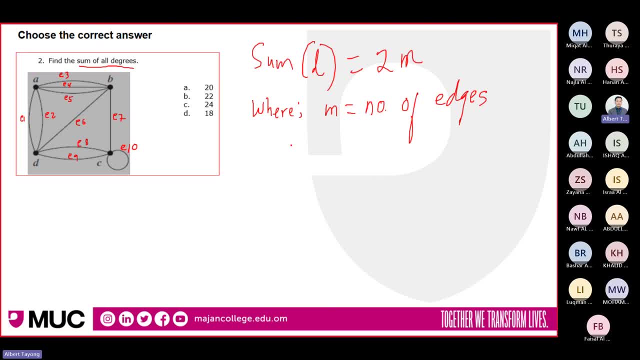 So there are 10 edges. So we have 2 times 10 equals 20.. So the answer is letter, Letter A. Okay, Of course you can do it manually. You can find the degree of A is 5. Because we have 1,, 2,, 3,, 4,, 5.. 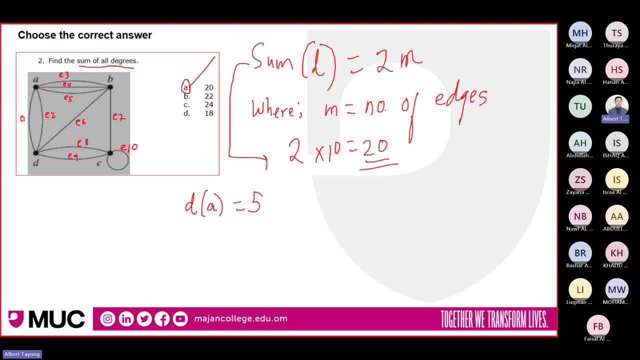 Okay, A is intersected 5 times, 2 times from D, 3 times from B, So total: 5.. Degree of B is also 5.. We have 1,, 2,, 3,, 4, 5.. 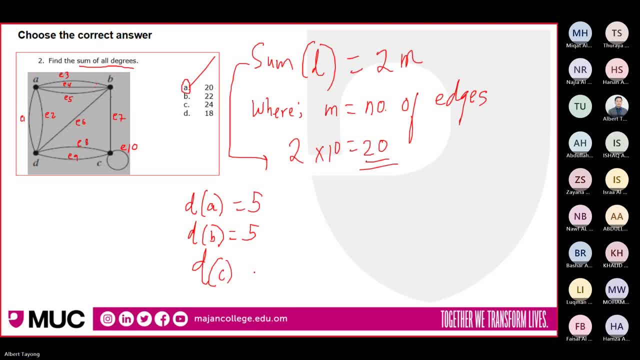 Degree of C is 5.. 1,, 2,, 3, and the loop is degree 2.. So total: 5.. And degree of D is also 5.. We have 1,, 2,, 3,, 4,, 5.. 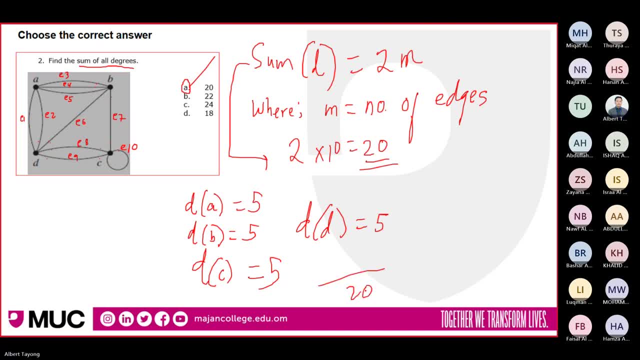 So the total is 20.. Okay, It's up to you, But the best method is to use the formula, which is 2M, 2 times the number of edges. It will never make a mistake. Okay, so let's proceed to number 3.. 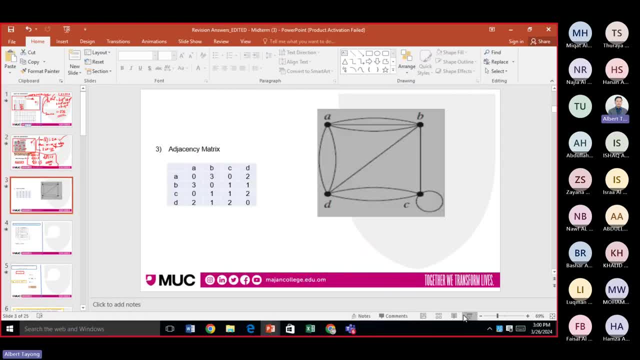 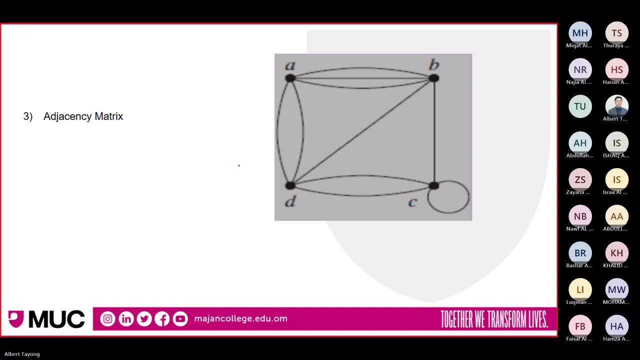 I think this one is very easy. Number 3, you're asked to create an adjacency matrix. For adjacency matrix, you need to create a table. The matrix is never made in Linux. That's how you remember nothing but a table. it has rows and columns, does it? 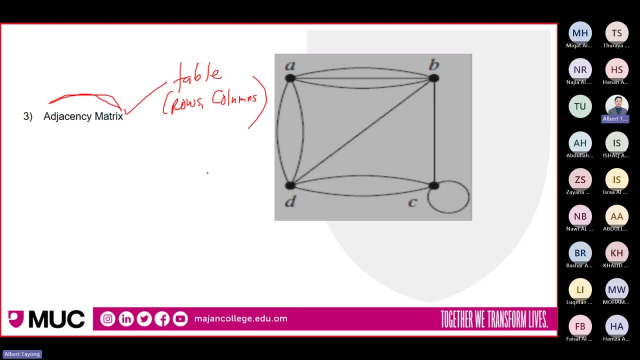 so adjacency means the direct or immediate connection. okay, it comes from the word adjacent. adjacent means there is a direct connection from one point to the other point. so basically you have to label your rows. okay, so we have ABCD. that will be your row ABCD. okay, so it's better to follow the alphabet. if the points or the vertices 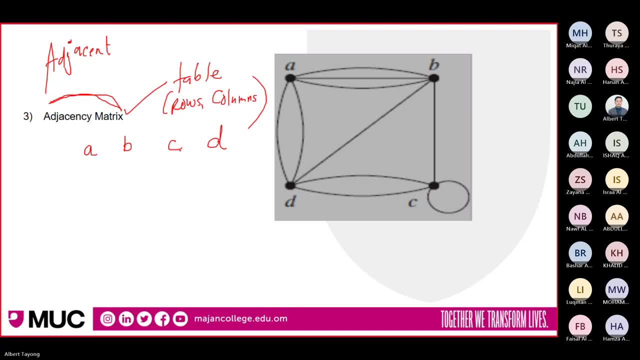 are given in letters to avoid confusion. so whatever you put on the row, you have to do the same for the column. this is left to right, top to bottom of a space here, so you have to put your a here. then you have B, C and D- here's space. don't put your a here. you. 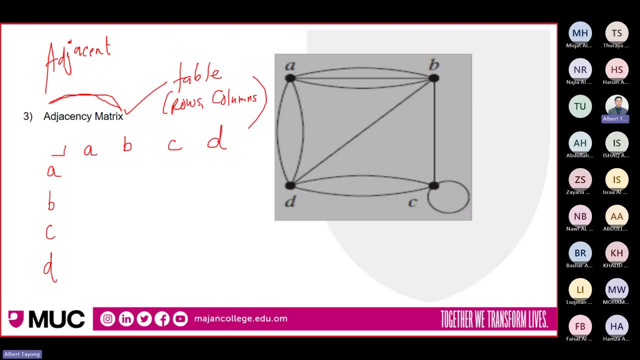 below the a. this one should be empty here. okay now, whatever you write in your row, you have to follow the same order. your ABC D: our column should be ABCD as well, but of course, if you're going to change it, it'll be correct, but it is easier to. 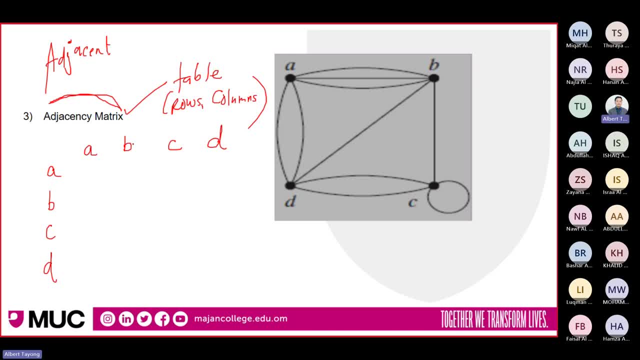 do it like that, so you are going to avoid confusions. okay, now, if there is no loop like a, there is no loop here, so a is not adjacent to itself, it's not connected to itself. so a to a will be zero, because a is not connected to itself, so it is zero there. 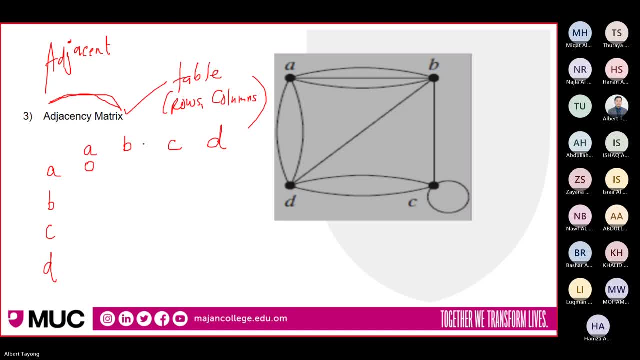 how about a to b? how many edges from a to b? three, three. so you're going to pull three here. do we have an edge from a to c? do we have a line from a to c? no, no, no, zero. how about from a to d? two, two. there are two edges from a to d. very easy, right. 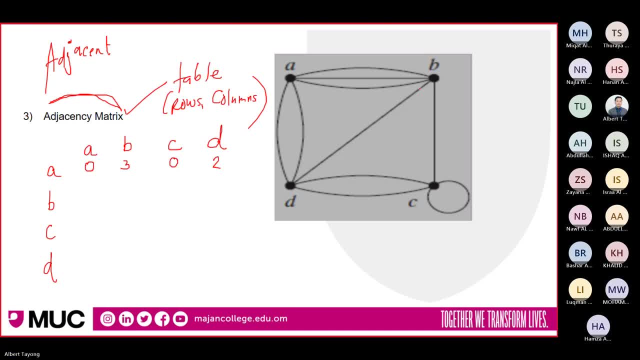 okay, let's look at our b. from b to a there are three edges, so this will be three. from b to b: there is no loop here. if there is a loop here, we have to put here one. but there is no loop zero. so b to b is zero. how about b to c? 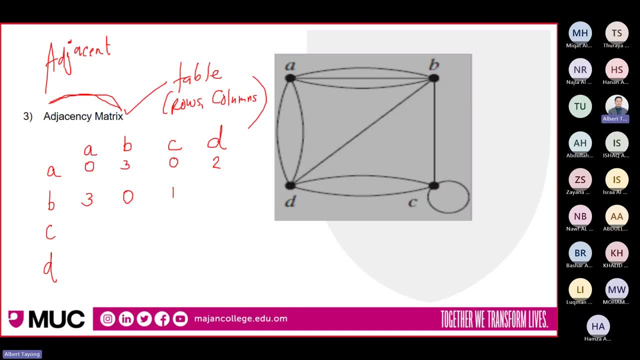 one one because there's one edge from b to c and b to d one. okay, so here the total is five. here the total is five is correct, because a- the degree is five, b- the degree is five in c, C to A. we don't have a line from C to A. 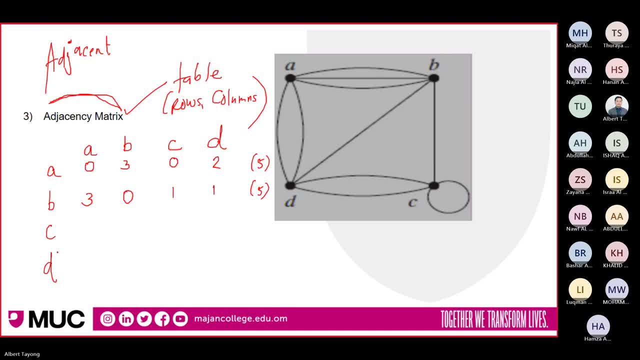 It will be zero. C to B. we have one line there, So one C to C: One One, Because we have one loop. If there are two loops, you're going to put two. C to D, Two. 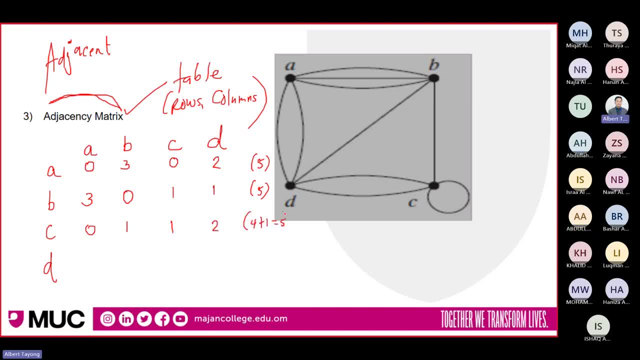 Two, So we have four plus one. five Because this one is times two here, This one Because we have loop. Okay, So this is a multiple choice question. What? This is a multiple choice question. No, this is not multiple choice. 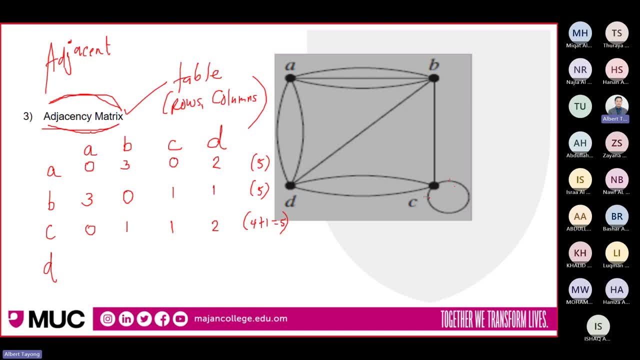 You are asked to create agency matrix here. Okay, Agency matrix table. If it is multiple choice, there is a, A, B, C, D answer. Okay, fair enough. Yeah, we don't have Here. we are asked to create a matrix, a table. 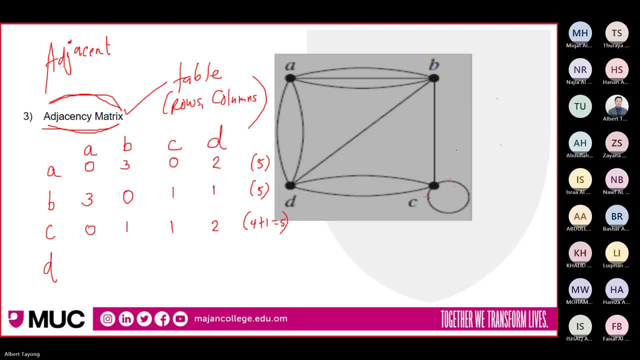 Okay, Number two, of course, multiple choice. Okay, D, It's connected to A. Two times Two, B One Two. Do we have a loop Zero? No, No, so d to d is zero, d to c is two, d to b is one, d to a is two. okay, so that's our. 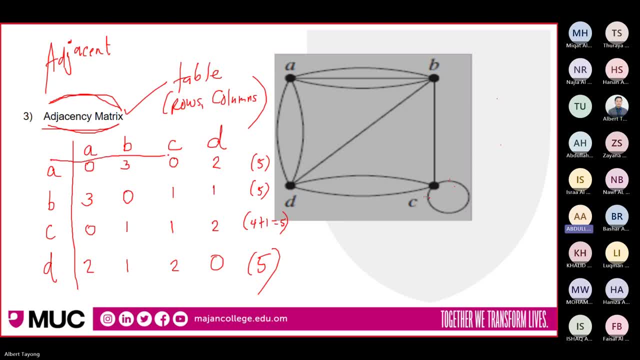 adjacency matrix doctor. yes, how about c? how come five? why no four? yes, because of the loop two. loop here degree two if loop two. yes, okay, okay. so this one will be, uh, times two here. basically this will be times two, but we put one because only one loop. 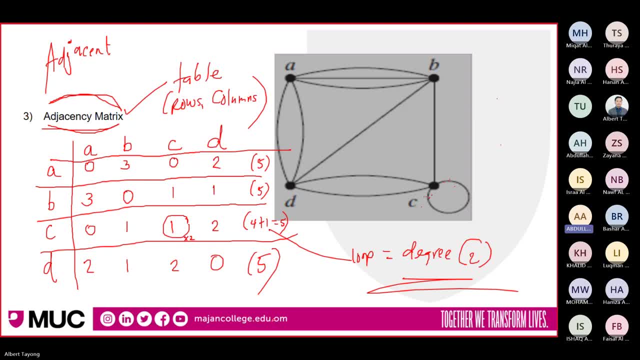 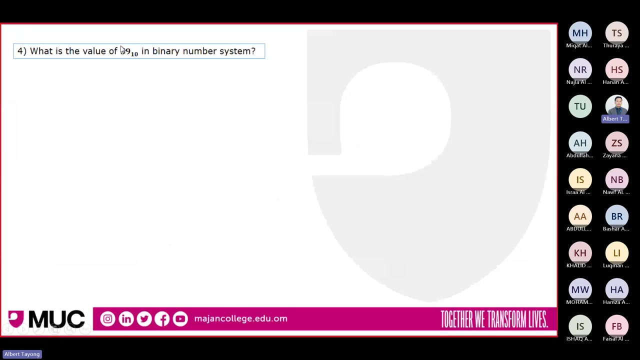 you understand? yes, yes, yes, okay. so let's proceed to number four. now i think this one is very easy, right? okay, this is our table, all right, so let's proceed to number four. number four: you are asked to change from uh decimal to binary, so you are converting from. 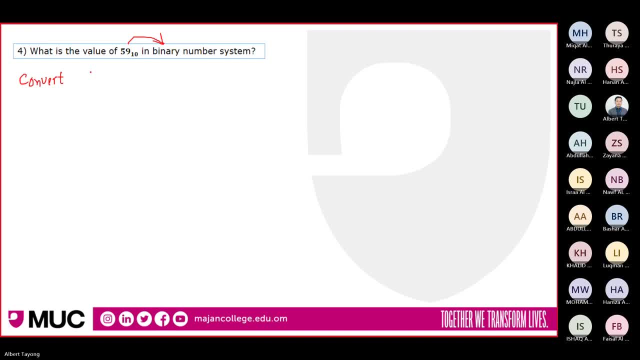 so let's put it on the right 59, base 10. so let's put it on the right 59, going to base 2.. why base 2? because binary. so please be careful on your exam. i might be saying octal here, so this will become 8 here. 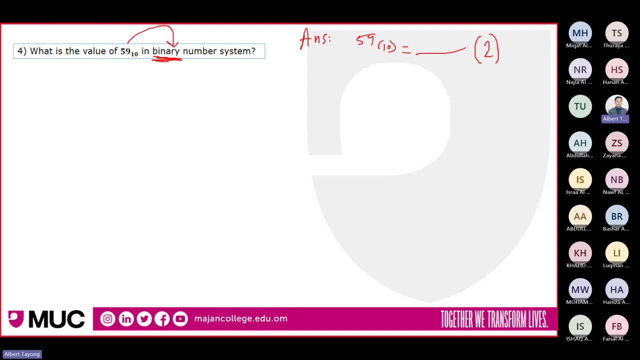 so 10 is on the left. we have two 59. create a table. please remember, if 10 is on the left table, so 59 and division here and remainder you can put r? e. so 59 divided by this number: 29.5, yes, 29.5. write only 29. 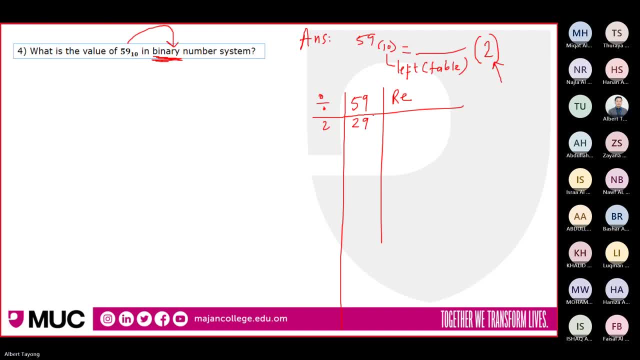 we don't need to write the decimal part here, so we have to bring this one down. so this will be: 59 minus 2 times 29 equals 1. a yes, this is always minus here. and these two you have to multiply. and now, if 29 divided by 2, 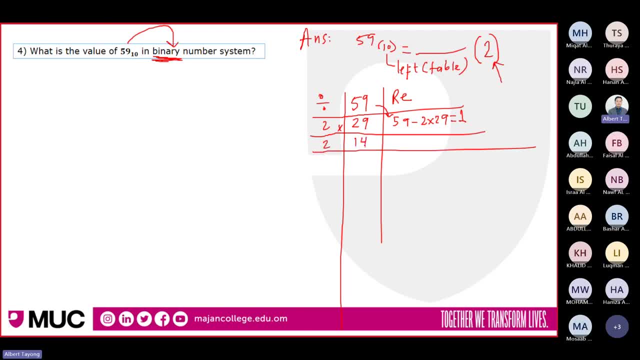 14.5 is 14.5, so 14. so bring down: 29 minus 2 times 14 equals 1: 1. okay, then 14 divided by 2 is 7.. bring down 14: 0 2 times 7, so 0. 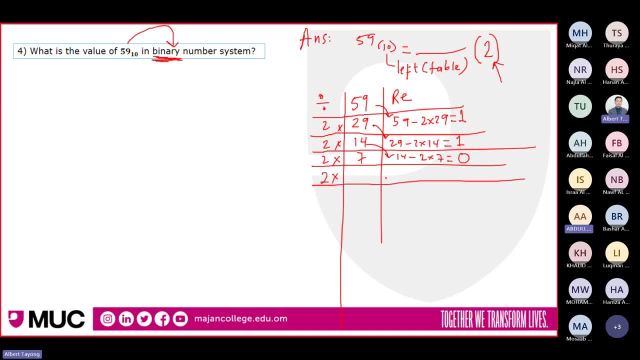 and 7 divided by 2, 3.5 it is 3.5. so we put 3, bring down 7 minus 2 times 3 equals 1, 1 and are we going to stop here? 0.5, no, no, 1. 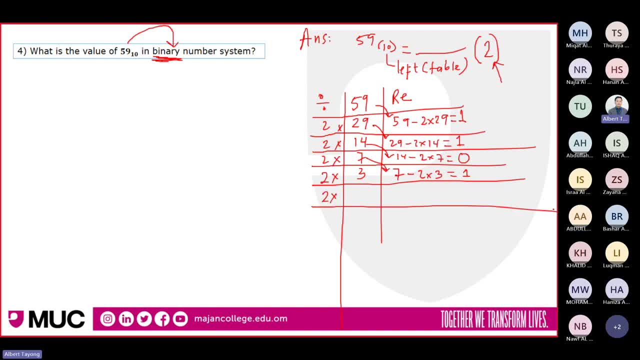 we continue. why we have to continue? because bigger than 2, right, yes, 1.5, so 1, bring down 3 equals 1, so we stop here. yes, why did we stop here? because coming zero, i think, or what? because smaller than two. okay, so we have to go up. 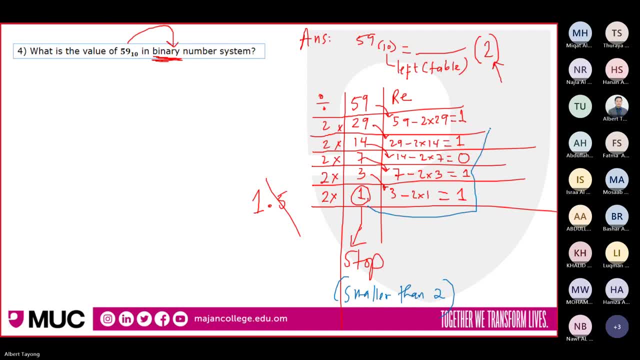 our answer. so we have to go up one one. start from where you stop, we stop at one, so start from there. one one, one, one, zero one, zero one, one base two. so the answer is one one, one, zero one, one base two. answer is 111011. 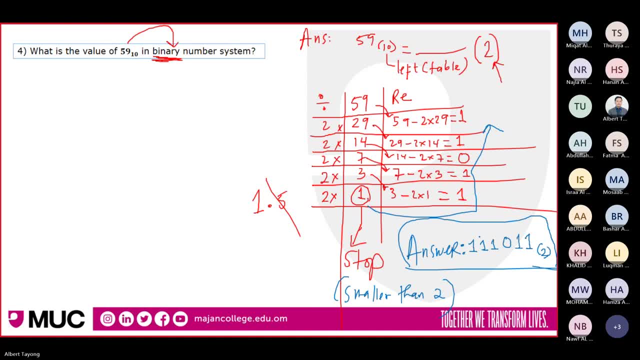 zero one one base two. any question here, guys? do you have a question here? no, so the answer is one one one. zero one, one base two one. can i ask a question? yeah, i, i'm a bit confused about when i used two, four, eight and division it. 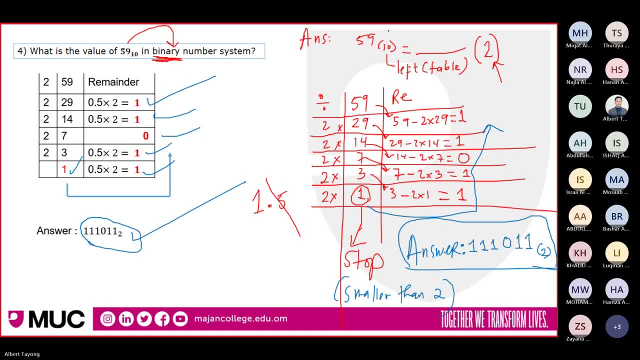 division. if 10 is on the left, yes, then here is on the left, okay, yes. now, for example, if i say in octal number system, here this 2 will become 8, understand, yes. if i say, hexadecimal, 2 will become 16.. is this clear? yeah, i see. 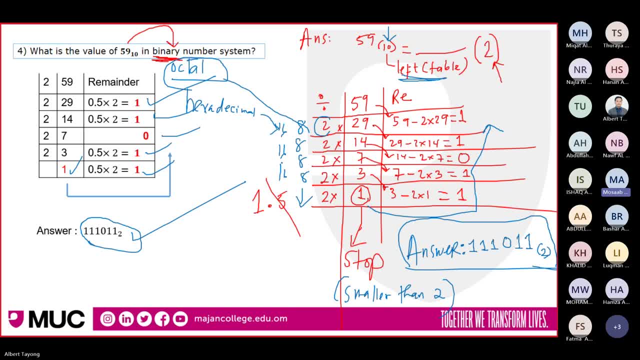 okay, but sorry, but i'm ask. you told us we can use the way we wrote: two and four and eight and both, one only or zero. that is only if you have 16 to 2, 2 to 16, 2 to 8, 8 to 2, only this, okay. 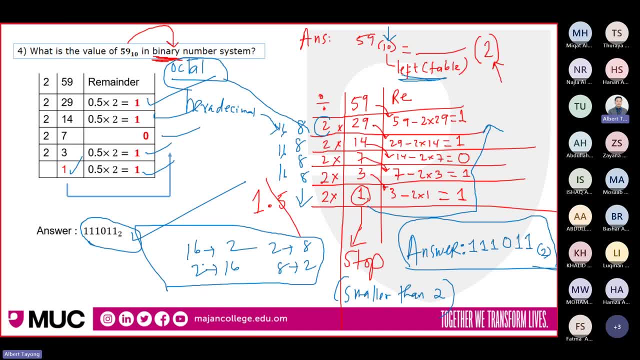 okay. okay, thank you for 16 and 2. you're going to use 8 4, 2 1 for 2 and 8, 8, 2, 4, 2, 1. only for this. thank you, okay. so, only for this. you're going to use 4 2 1 or 8, 4, 2, 1. 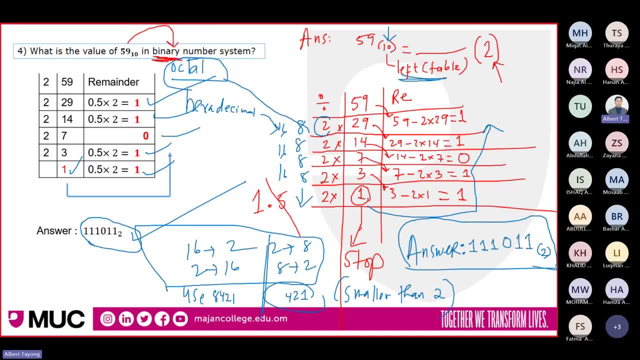 for example, see here there is no 10. you're going to use a table and you're going to use 8, 4, 2, 1. going to use a table if 10 on the left decimal- but here we have 2, 8, 8, 2, 16, 2, 2, 16. we don't have 10. 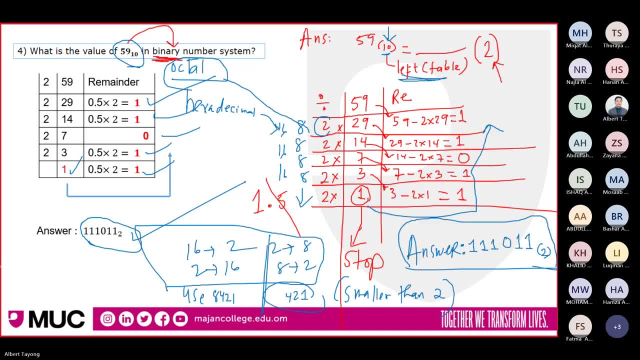 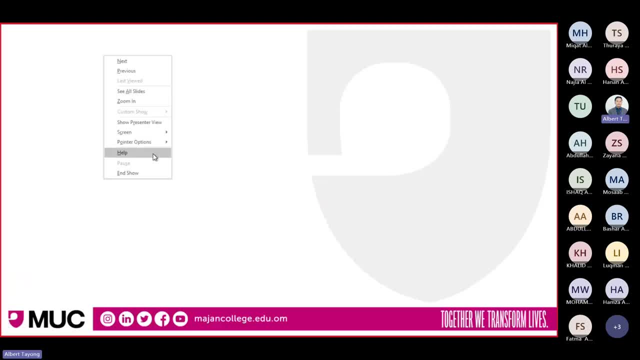 there. but, for example, if you have, like this, seven, four, then eight, going to base two. So this is the time you're going to use 4, 2, 1, Because you have 8 and 8 and 2. So 7 equals 4, 2, 1. 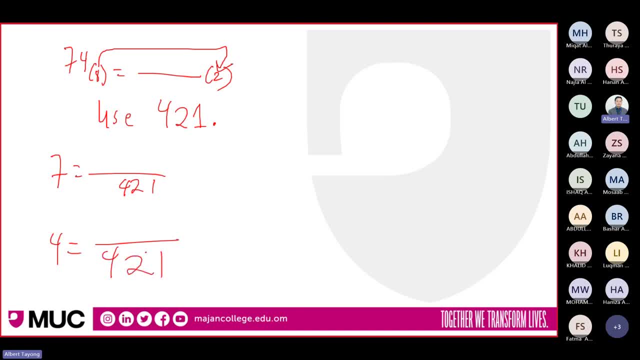 And 4 equals 4,, 2, 1. So for 7 you need 4,, 2, and 1, Because 4 plus 2 plus 1 equals 7. So you have to turn on All the digits Here. you need only this. 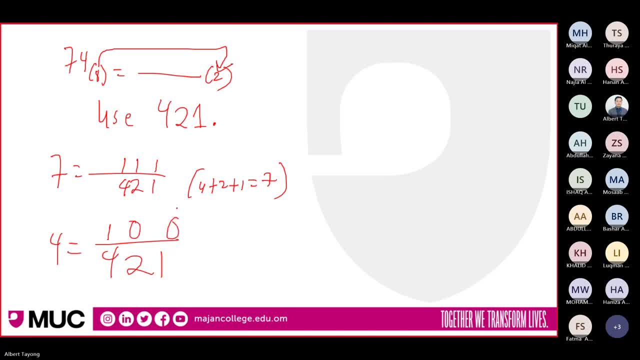 This will be 0, 0, Right, Okay, Is that clear? Yes, thank you. So the answer will be 1, 1, 1, 1, 0, 0. Base 2: Okay, And the other one is 16. 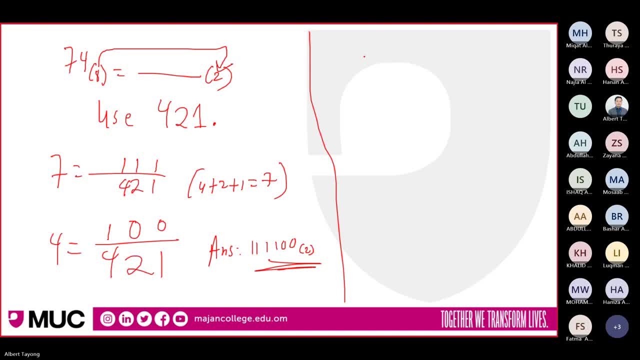 For example, you have, Like this, Going to 16, Assuming you have 1, 0, 1, 0, 1, 0, 1, 1, 1. Base 2, Going to base 16: Okay, So You have 1, 0, 1, 0. 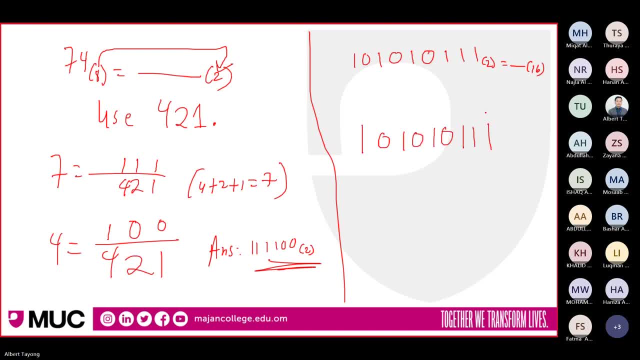 From right to left, So 2 to 16: 8, 4, 2, 1. So here You will have 4 digits: 1, 2, 3, 4, So 1, 2, 3, 4. 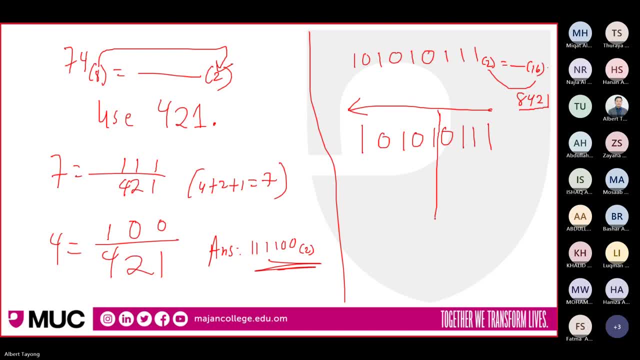 1, 2,, 3, 4, And then 1, 2,, 3, 4, So this will be 8, 4, 2, 1- Here Equal to 7, Here 8, 4, 2, 1. 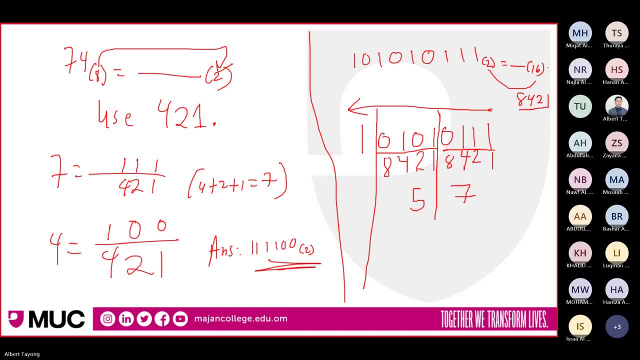 8, 4, 2, 1, 8, 4, 2, 3, 4 Equal to 5, Because we count only 4 and 1 And here we have 1 directly. So the answer will be 1, 5, 7. 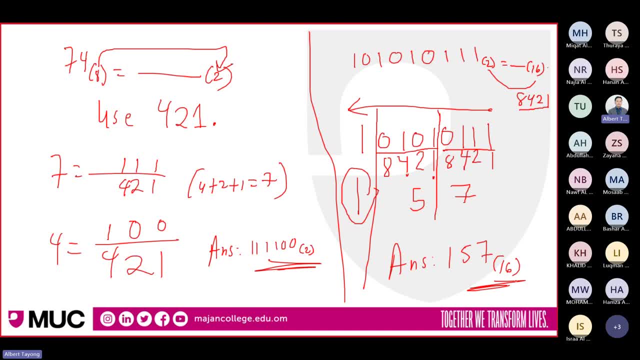 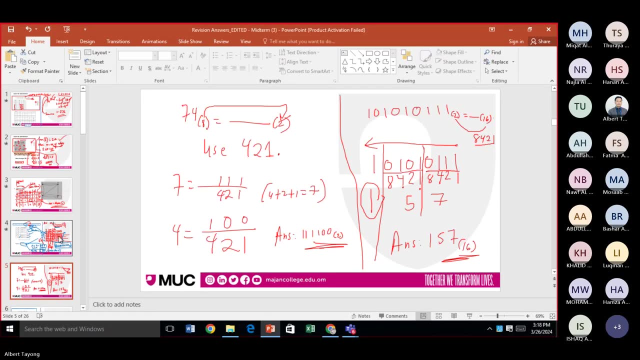 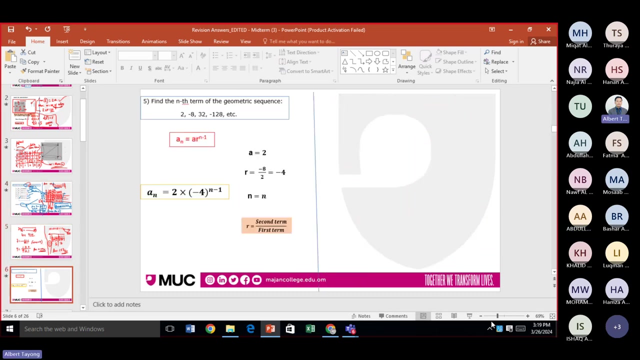 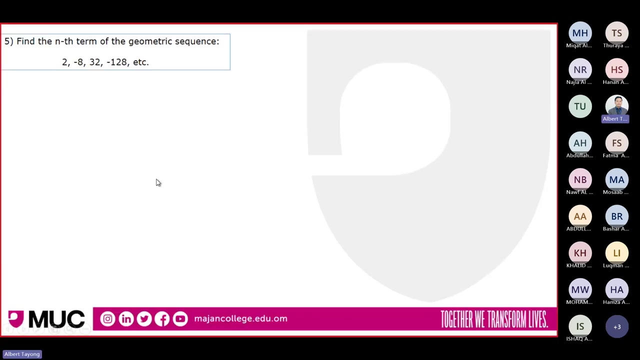 Base 16. Okay, Is that clear now? Yes, Alright, so So let's proceed to the next Number four. Let's go to number five. Number five: you're asked to find the nth term of the geometric sequence, Geometric sequence. you know the formula. 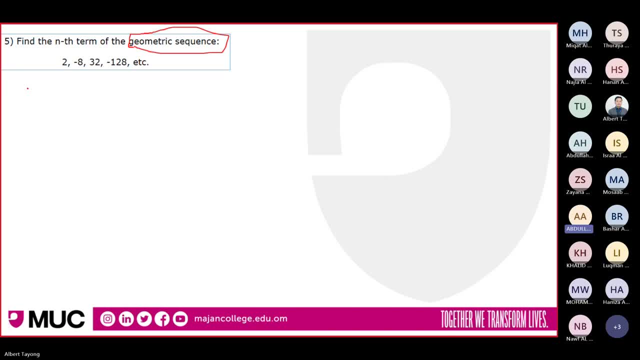 A sub n equals a times r raised to the power of n minus one. So please remember this always. So you have to use the given. What is the given Geometric sequence and this sequence here: two negative eight: 32, negative one: two eight. 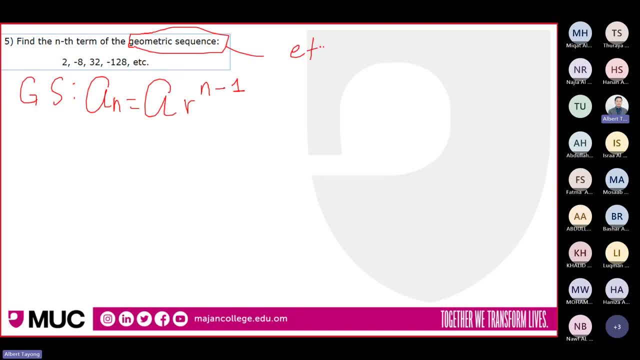 et cetera. Et cetera means that that that Here, That means it will continue. Okay, so we have our first term Two. This is the first step. Our first term is two. Two A is equal to a sub one. 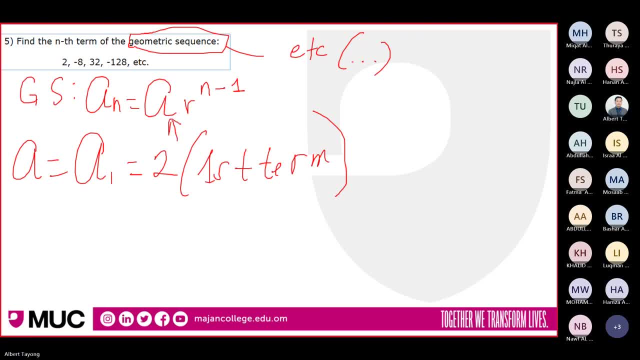 This one And then your r equals a sub two. divide a sub one. Negative eight. divide two negative four. So these are the steps to find the n term here. okay, so let's solve for the n term. it means you are not going to change your a sub n. 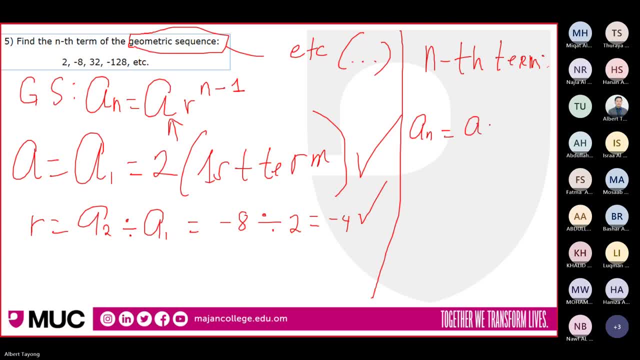 okay, your a sub n will be the same. okay, so a sub n equals 2. that is your a times r negative 4 raised to the power of n minus 1. okay, we don't need to simplify this because you have negative 4 here and 2. 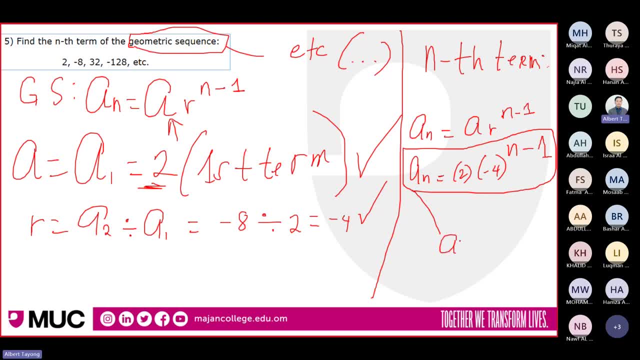 this is the answer. 2 times negative, 4, raised to the power of n minus 1. okay, is that clear? a a first number, doctor, yeah, a is the first number first and r second. no, r, is this one a sub 2 divided a sub 1? yes, yes, 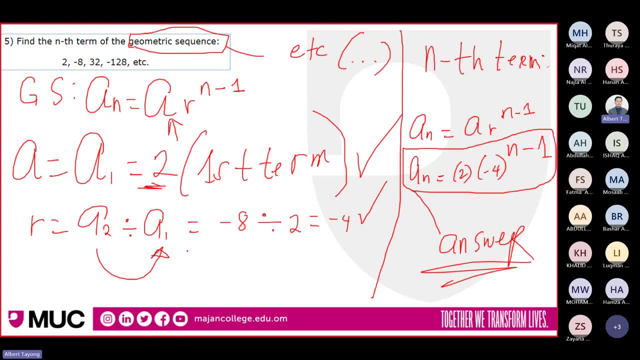 it's not the second one. it is a sub 2 divided by a someone. yes, so negative 8. this is your. a sub 2 divide a sub 1. it's negative 4. right, yes, okay. so i think that's very clear. okay, let's go to number six now. 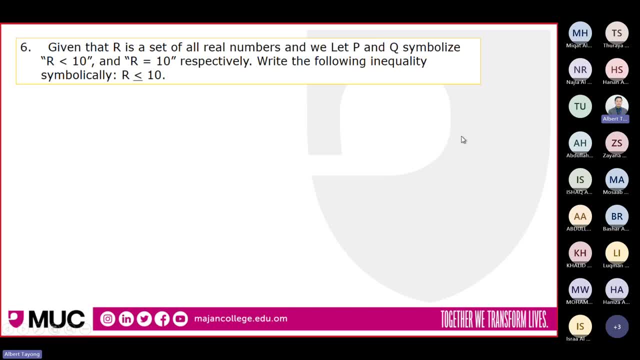 okay, this one. i had an example of this during the support class last week. okay, so i hope that you remember. still mention here: r is real numbers, of course. real numbers any number that can be represented on the number line, anything that can be represented here is what we called as a real number. 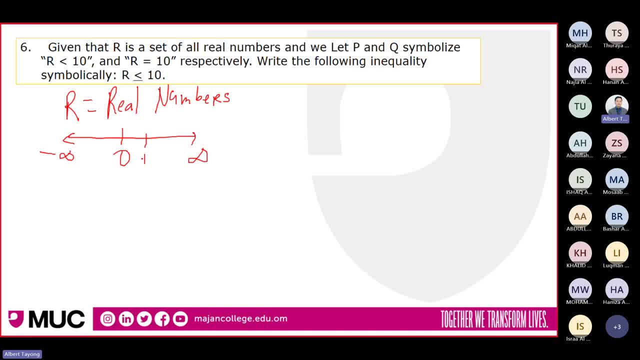 so 0.5 is a real number. This one Square root of 2 Is a real number. after 1, 1 point, something Okay. so any number is called as a real number. Now, as long as it has a value, We let P and Q. 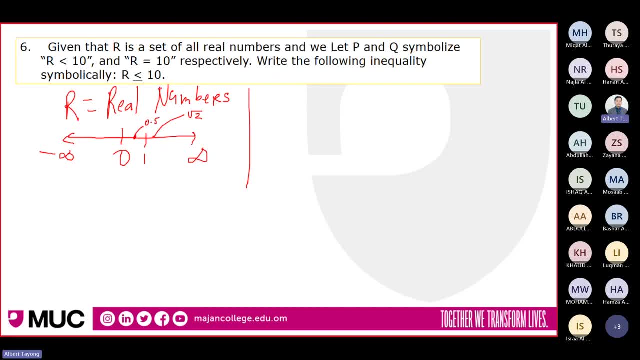 Symbolize R less than 10 And R equals 10 respectively. The word respectively is there. It means we have to follow the order. The first is P, So P will take the first value. R is less than 10. The second is Q. It will take the second value. 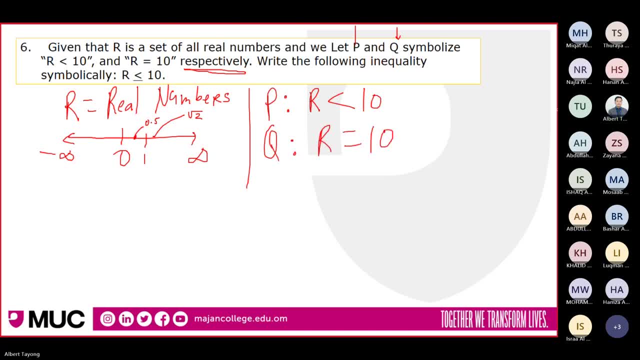 R equals 10. Okay, that's the meaning of respectively. Let P and Q symbolize R less than 10 And R equals 10 respectively. So it means P is R less than 10 And Q is R equals 10. So when I say Ahmed. 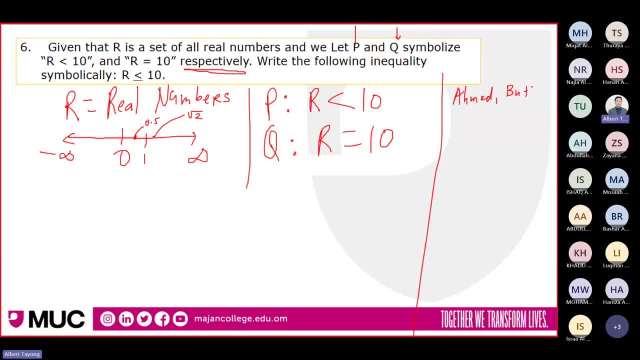 Hussainah And Faisal. Okay, This equals right here: R5, 10 And 6 years old Respectively. What's the meaning of this? What's the meaning of this? Ahmed is 5 years old. Hussainah is 10 years old. Faisal is. 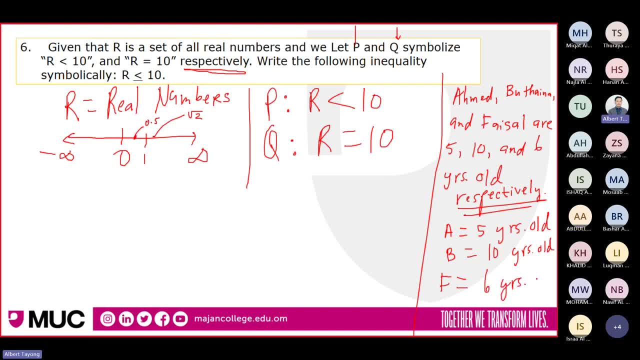 6. Did you understand the meaning of respectively now? No, It follows the meaning of respectively now. It follows the meaning of respectively now. It follows the order. This is the first, Second and third. So this will be for the first, Second and third. That's the meaning of respectively. 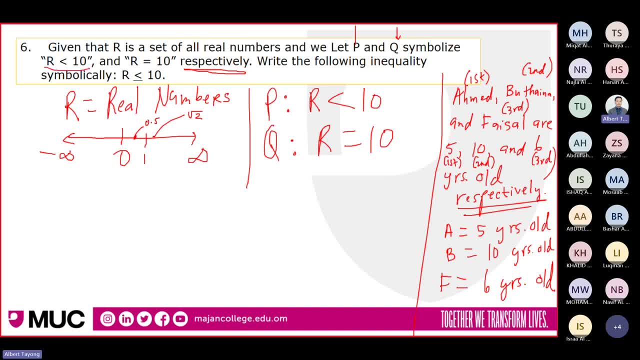 So here, P and Q. So P is this And this is for Q. Write the following: inequality symbolically. So P is this And this is for Q. Write the following: inequality symbolically. The result of the first infinity project, Say P, is this: 0. What is the quality symbolically? 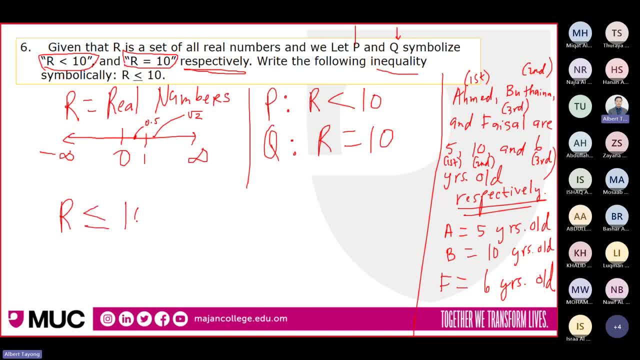 R is less than or equal to 10. So this is the given: higher is less than or equal to 10. So what's the meaning of higher is less than equal to 10? What does it mean? It means we have R is less than 10. 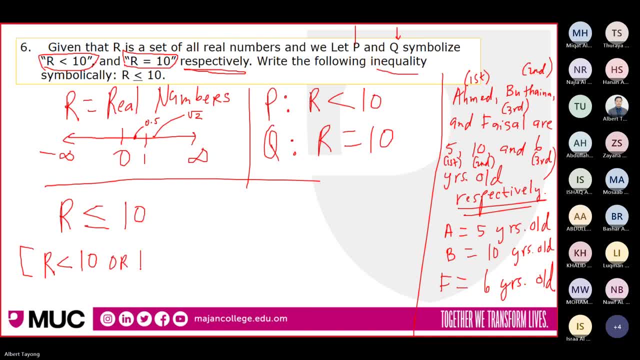 It has视لان Beings C or r equals 10. if we have simple inequality with an equal sign, we use or okay. so the answer will be: are less than 10. that is P, change to P, or this is or like V or seven in Arabic. on r equals 10 is Q. 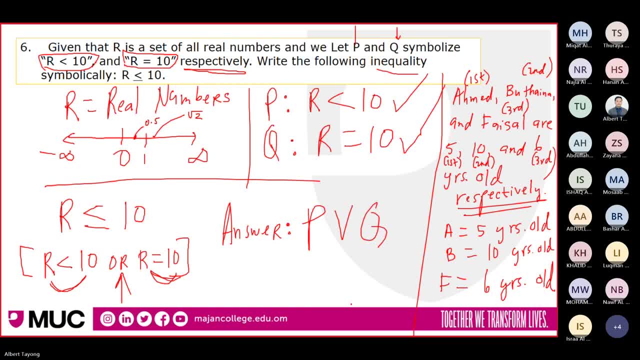 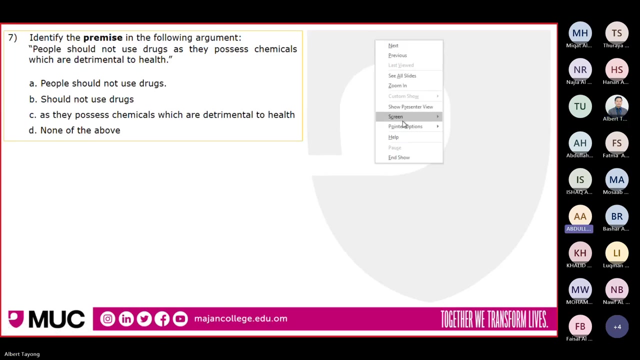 so the answer is P or Q. okay, any question here? is this clear? yes, okay, let's go to number seven. you, you number seven. you are asked to identify the premise. so, as mentioned before, premise is the evidence or evidences. this is the reason, the reason why we are claiming something. 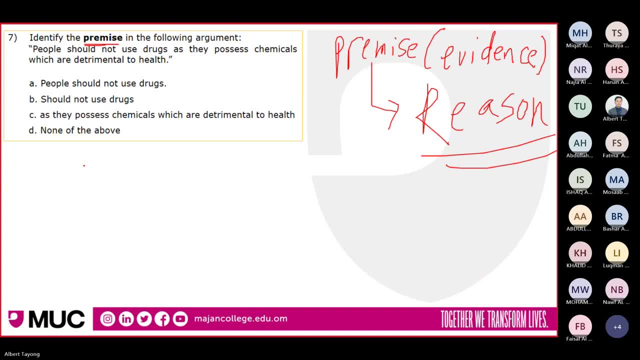 okay. so this is the argument: people should not use drugs as they possess chemicals which are detrimental to health. detrimental means harmful, okay. so what is the premise here, as they positions chemicals. so what is the premise here? yes, the ass, there is like, because as they possess chemicals. yes, the ass, there is like because. 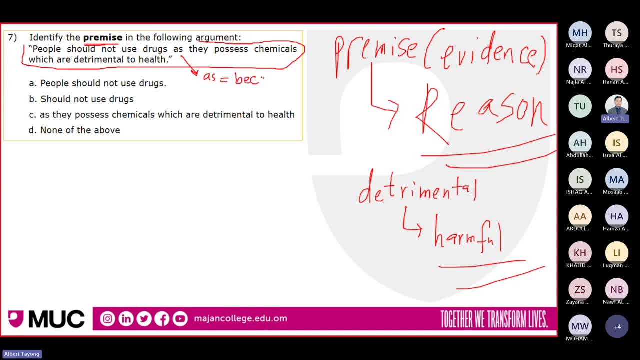 us. there is like: because us, us is equal to because a us, since these are the common ones, common indicators of premise or premises, so let us see the answer. so because or as they possess chemicals which are not good for health is detrimental to health. so what is your conclusion here? 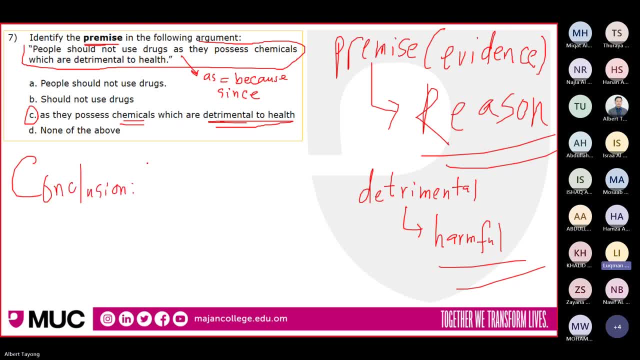 i might be asking you to give. people should not use drugs. yes, people should not use drugs. should not use drugs. we're talking about the illegal ones. illegal because some drugs are legal, like coffee. coffee is a drug- actually, coffee is actually a type of a drug, but it is legal. we're allowed to drink coffee. 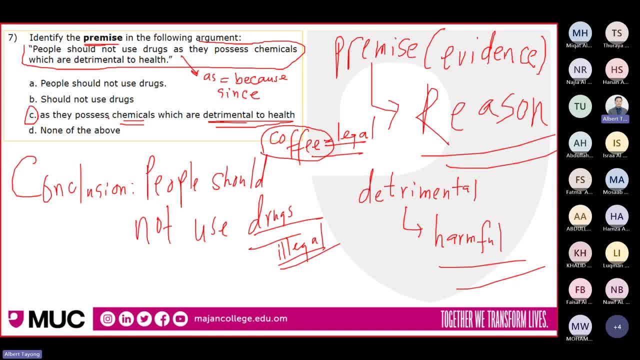 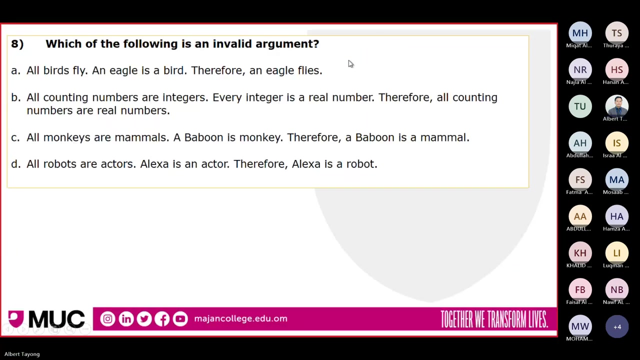 okay, but now you are fasting, you're not allowed to drink coffee, okay, so we talk about legal drugs here. that is the premise. that's the reason. it has some chemicals which can harm your health. number eight now in number eight you're going to. this is also part of the support class last meeting, last thursday. 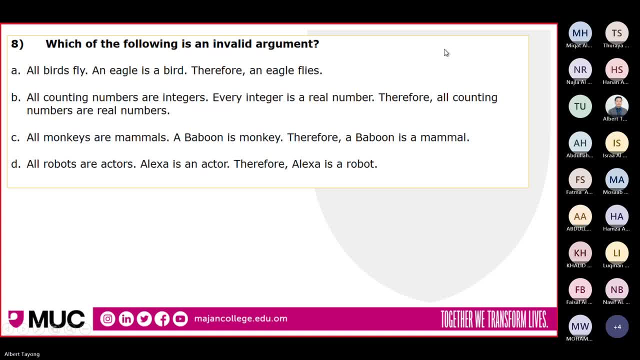 about valid and invalid argument. now, as i mentioned during the support class, there are two valid arguments. one is a, b, c, a, c b, where this is general. so please try to take note of this. this is the first valid form. the second one: a b, b, c, a c. 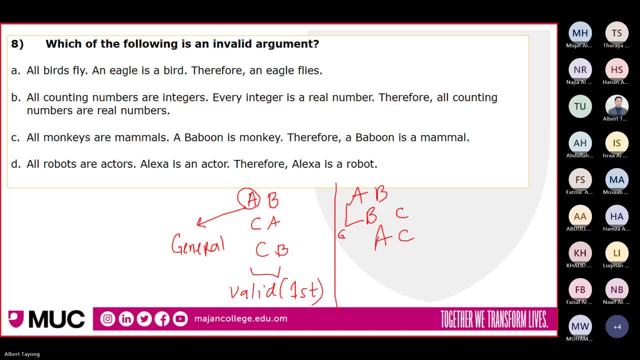 where a and b should be general. when i say general, it's universal, like every, everything, any, anything, okay, all everything. these are the keywords, but usually the most common one is all. it's actually universal, like the first one here. all birds, so all birds. this is your a. a means the subject and b is the predicate. 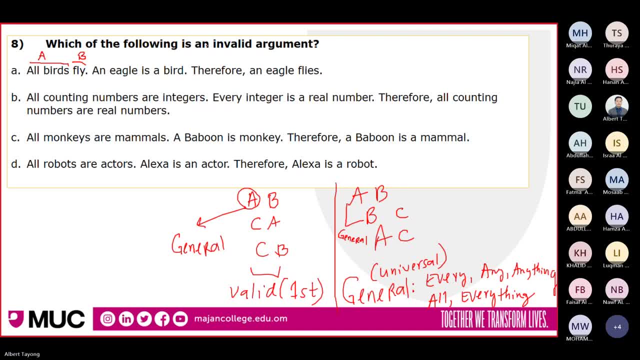 there is only one word in the predicate: fly, okay. so a is the subject and b is the predicate. this is the predicate, for example, when i say: for example, when i say so, is a student is a student at muc. so here, where is the subject? what is our subject? 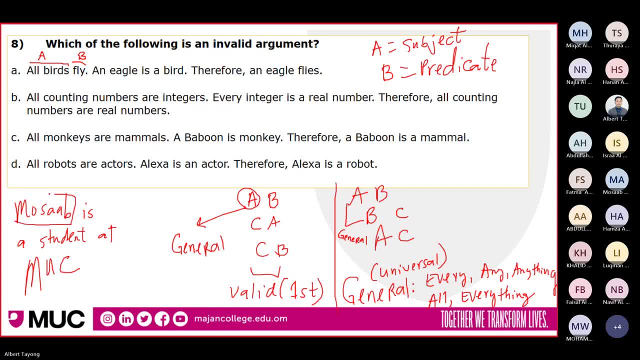 how is our subject? This one, and is a student at MUC, is the predicate. predicate is the, the phrase that describes the subject. So, is a student at Madan University College is describing our subject, But the whole phrase that describes the subject is called as predicate in grammar and in logic. 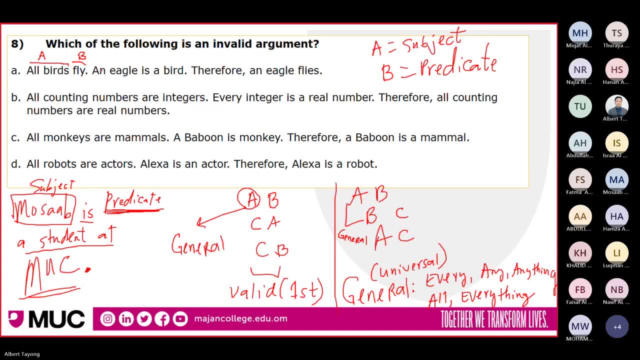 Now in the second one, an eagle. So here an eagle is not mentioned in the first sentence, so this will become C Because it's not mentioned here. we have A and B in first. We don't have eagle here, So is a bird. 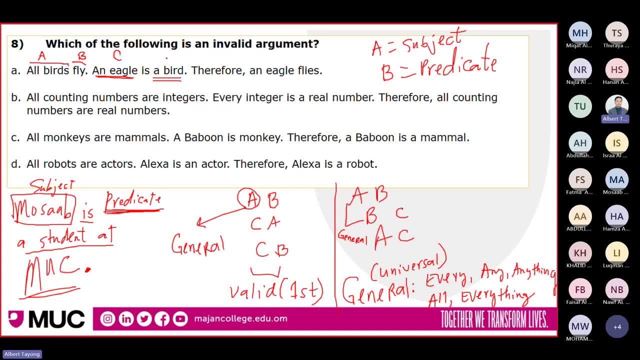 A bird. here is A, A, Very good, Very good, Because it's part of all birds. So it follows A, B And C, A. Therefore an eagle C flies, B is same here B, So this is a valid argument. 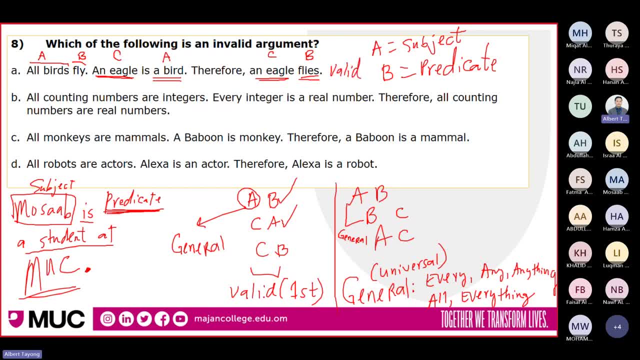 A, B, C, A, C, B, where A is general, all birds, Of course. if we say all birds fly, an eagle is a bird. therefore an eagle flies. Okay, In general we don't care whether it is true or false, but if the first two statements 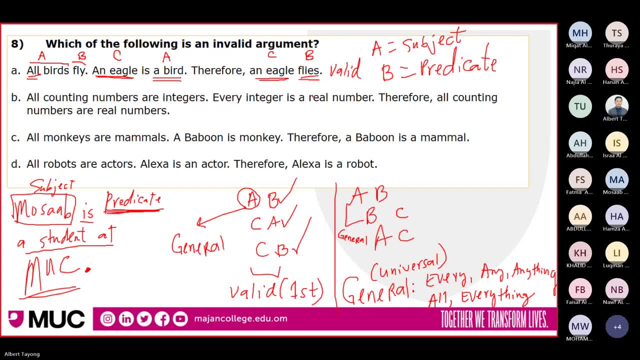 are true, the conclusion cannot be false. Okay, Let's try to look at letter B. All counting numbers are integers. So this is our A, A And integers B. This is our B. Every integer is again B, B. 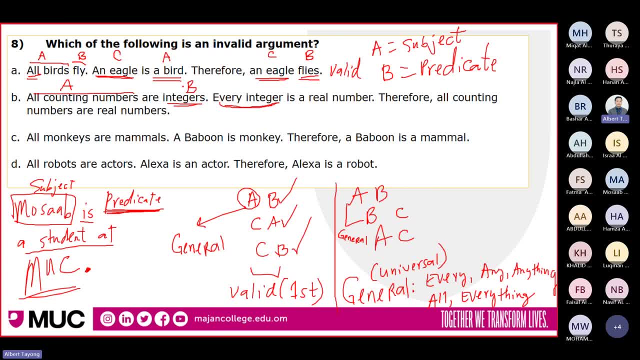 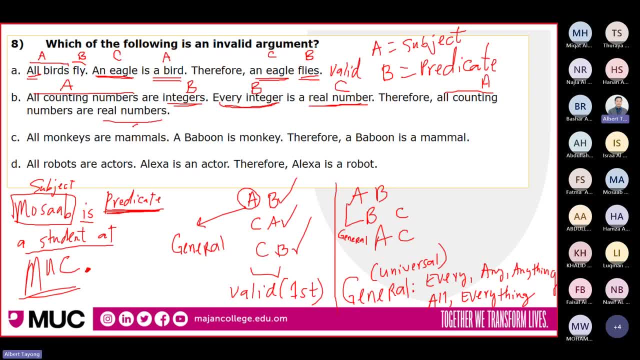 Real numbers B, C, B. Real numbers A, C. Real numbers C. Real numbers A, B are general. you have all and every, so the second one is valid. okay, so this is the second valid form here now. here let us see all monkeys: a, mammals, b, baboon, c monkey. a baboon is c, c, mama, mama is. 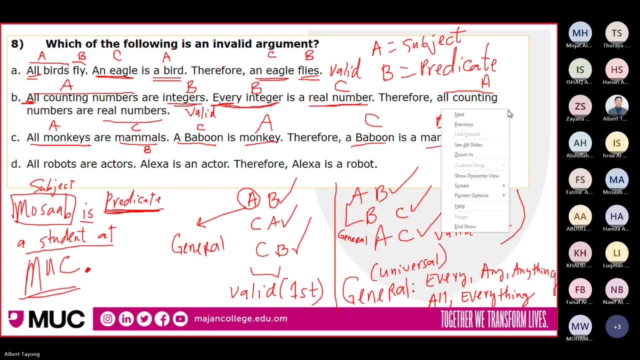 this follows the first one right first valid form: a, b, a, b, c, a, c b is valid, so that means the last will be invalid. yes, this is invalid, why all robots: a are act, actors, b, alexa is c, c, actor is b. so immediately invalid because it violates. it should be a, b, c, a. 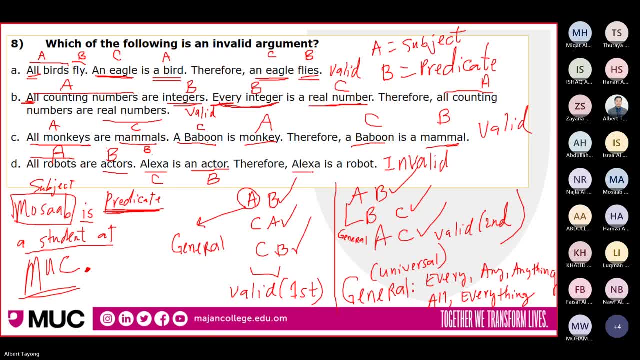 but here a, b, c, b. alexa is c, robot is a, so it does not follow. it violates this rule here. okay, so letter d is invalid. so, guys, in validity of argument we don't care whether the statements are true or false, because if it follows the structure- the first and the second structures here- then automatic the. 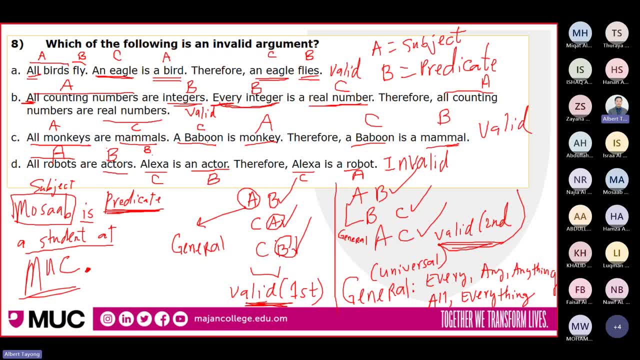 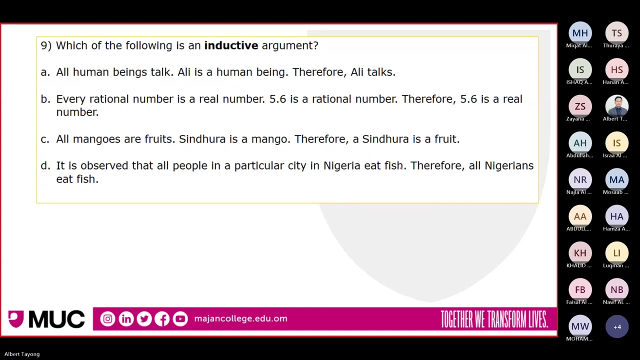 conclusion will be true if the premises are true, means the first sentence and the second statement. if these first two are true, then the conclusion will be true if it follows these structures. okay, this is your prayer time now. okay, number nine. okay, number nine. we will discuss number. what's the time now? 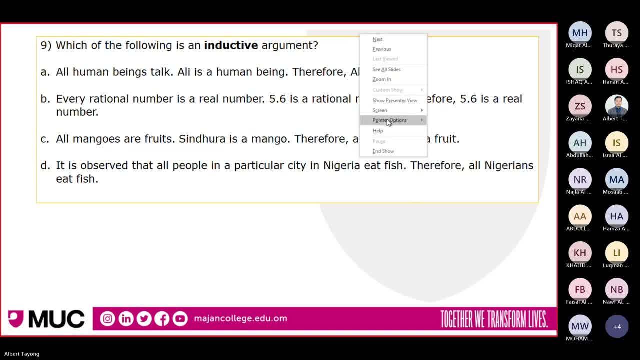 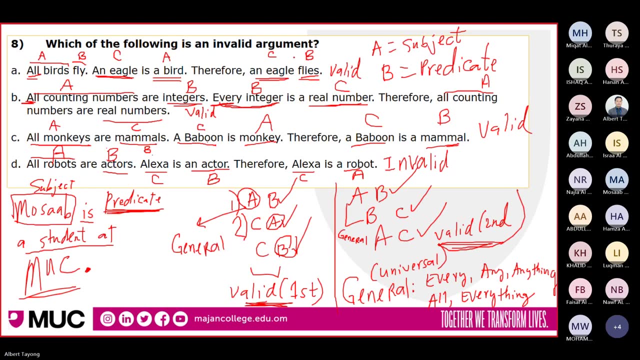 this is your prayer time, okay here. inductive argument: this one was discussed also last meeting. inductive and deductive. deductive are all of this. all of these arguments- i gave you a number eight- a, b, c, d are deductive. deductive usually follows three sentences, three statements. okay, like a, b, c, a, c, b. 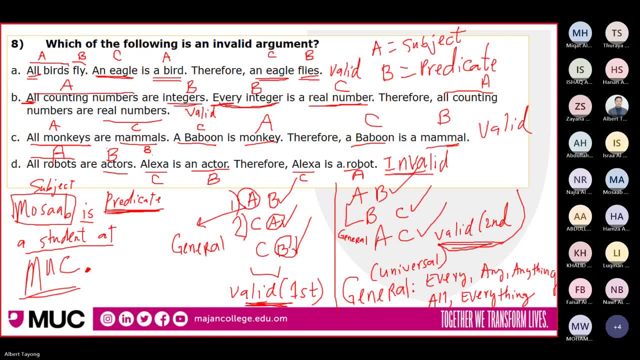 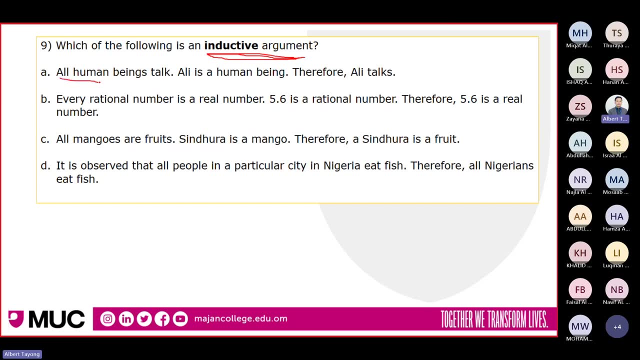 even if it is invalid, still it is deductive. so deductive argument will start with two premises and conclusion, always. so let's look at this. this one is deductive because we have a b, we have here c a, c b, so this deductive very easy to identify. 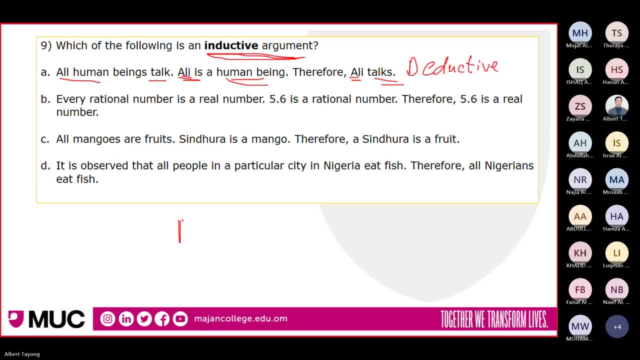 so in deductive you have premises one, premises two. conclusion: that's deductive. it will start with the general and then specific. see, so this is from general to specific. so this is from general to specific, like this is from general to general. right, this is general, all human beings talk- and then specific here specific. 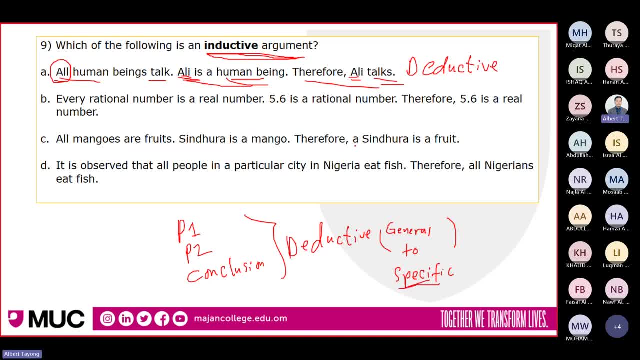 ali is an example of human being, therefore ali talks. so from general to specific example and a specific conclusion. We have A and B, another sentence and then conclusion. So again, this is deductive. Yes, this one. again, we have three sentences. 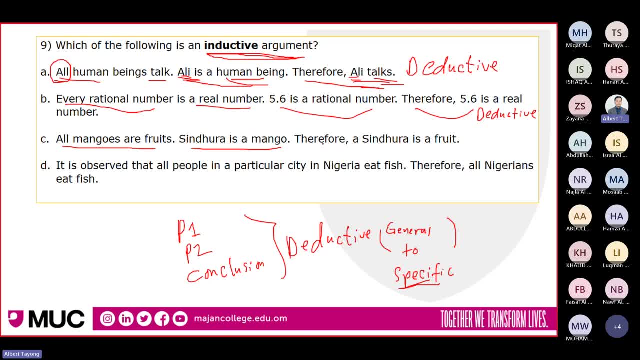 One. an example of a mango Deductive. also This is deductive, So the last will be Deductive. What is this? inductive Inductive means we start from specific to general Inductive: Usually we use observation. Okay, we use observation. 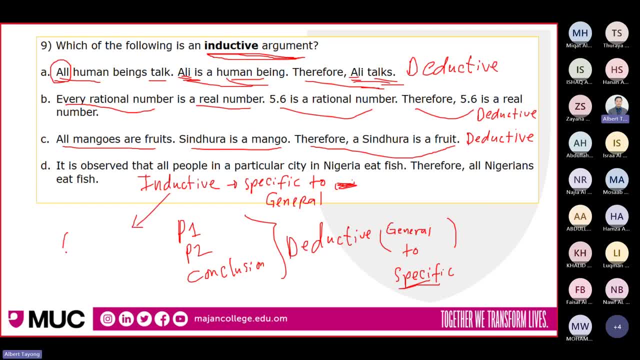 Not right here. Okay, so we use observation, We use some samples or experiment to conclude, or gathered facts, information, Like it is observed that all people in a particular city, so particular city in one city only in Nigeria, eat fish. 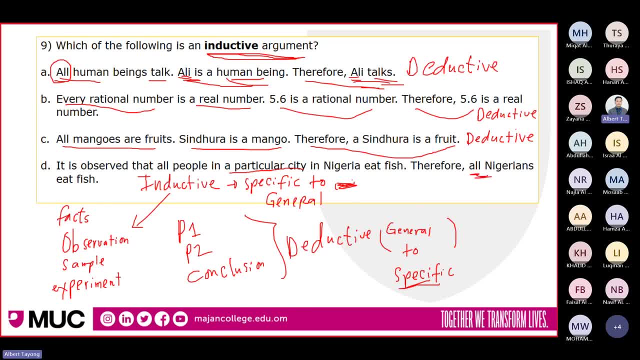 Therefore, all Nigerians eat fish. Are you sure that all Nigerians eat fish? No, Your conclusion is just based on your observation Using one city, So it means you conducted a survey, or maybe you interviewed all the people in this particular city in Nigeria. 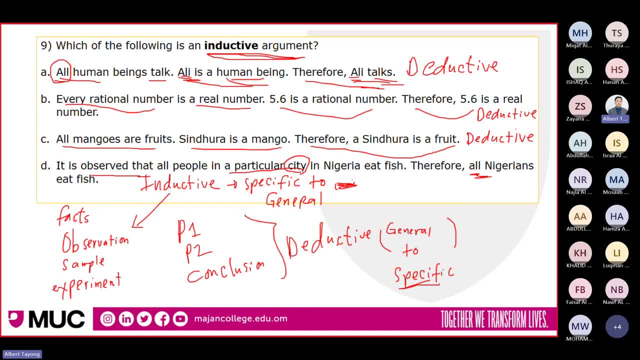 Asking them if they eat fish And they said yes, all of them. And now you are concluding that the whole people in the whole country, all Nigerians, eat fish. So the conclusion is uncertain. We call this a probable conclusion. That means we have to verify our conclusion. 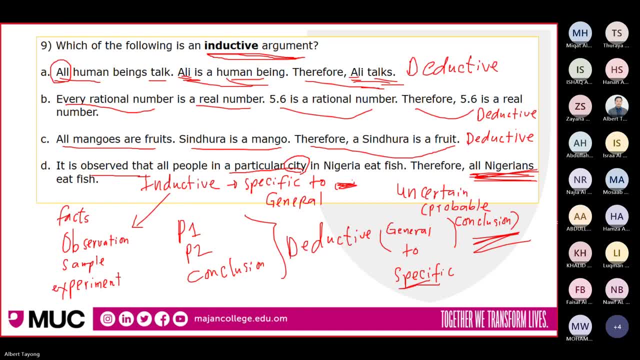 Maybe true, maybe not, Maybe Okay, because you have already observed that all people in one city in Nigeria eat fish And you are saying that everyone in this country eat fish. Nigerians are so many- I think there are more than 200 million. 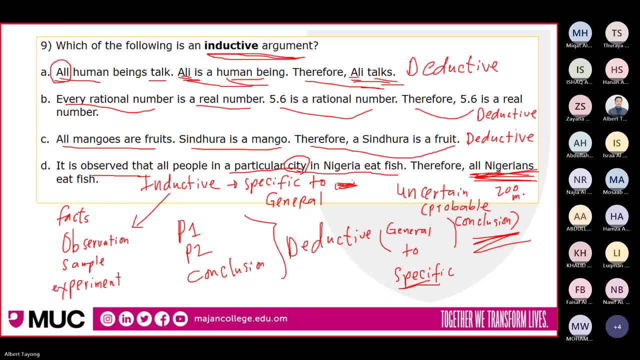 It's the biggest in Africa. Okay, So the letter D is inductive argument. From specific to general. This is general here. Specific is this one Particular city, One particular city. Your conclusion is all Okay, so maybe you take your break now. 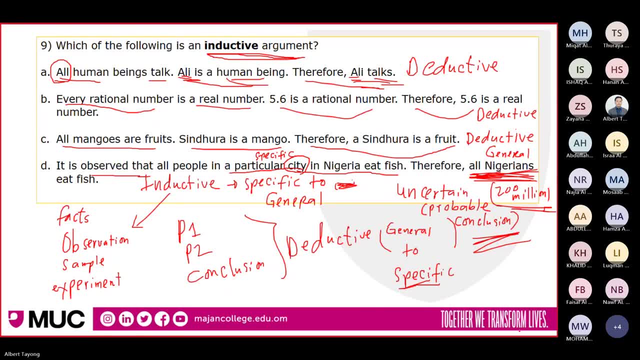 406,. you have to come back. Okay, guys, Don't worry, We will finish everything during the support class On Thursday. Okay, see you, We'll be back, All right, Thank you, Thank you, Thank you. 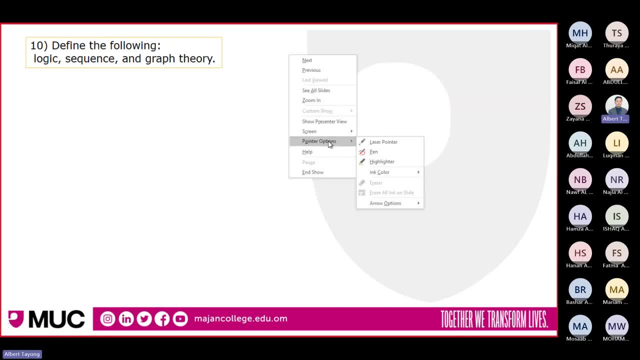 you have to know what is logic, what is a sequence, what is graph theory or what is number system. so usually this will be part of your multiple choice. okay, logic is the study of correct and incorrect reasoning. it is also the science of the necessary laws of thought without logic. 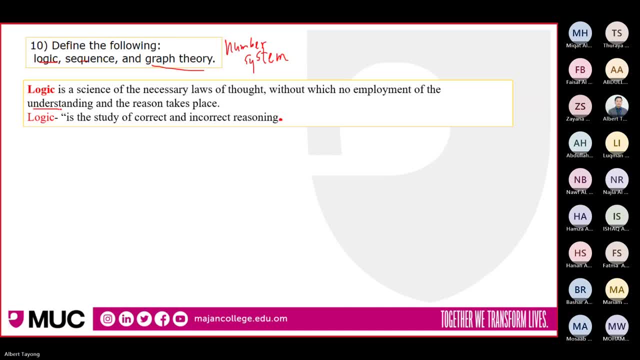 you will not be able to understand and reason out properly. so, without which no employment of the understanding and the reasoning takes place. this one here is reasoning. so in logic, actually, reasoning is equivalent to thinking. when you reason out, you are actually voicing out your thought. okay, what you think. 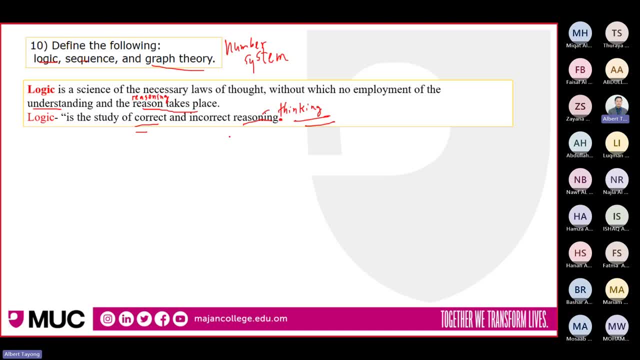 so it is the study of correct and incorrect reasoning or a very simple definition. it is the anatomy of thinking. anatomy is the structure of thinking. what else it is also called as the science of argumentation. why science of argumentation? because usually we look at arguments: whether it is valid. 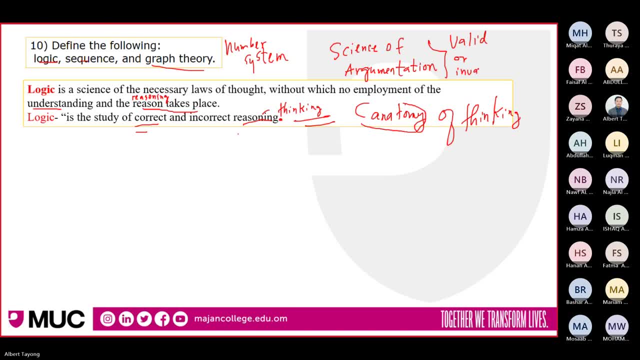 or incorrect argumentation, and we look at deductive argument, inductive argument. okay, that's why it is also called as the science of argumentation, because we look at the validity of the argument and types of argument, whether it is deductive or inductive. okay, sequence is an ordered list of things. 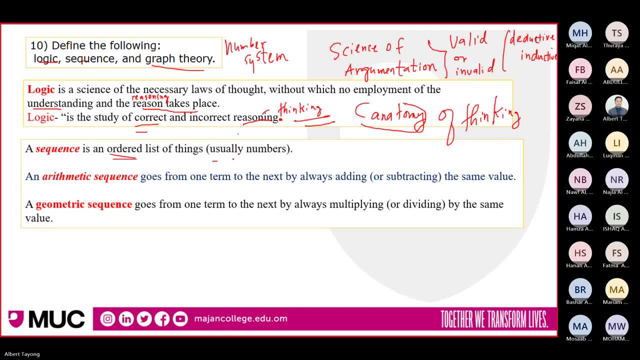 the keyword. there is ordered, usually numbers. not always. in most cases we deal with numbers, but of course a sequence can be anything. it could be a variable also arithmetic sequence. this is a sequence of numbers. this is a sequence of numbers. this is a sequence of numbers going from one term to the next. 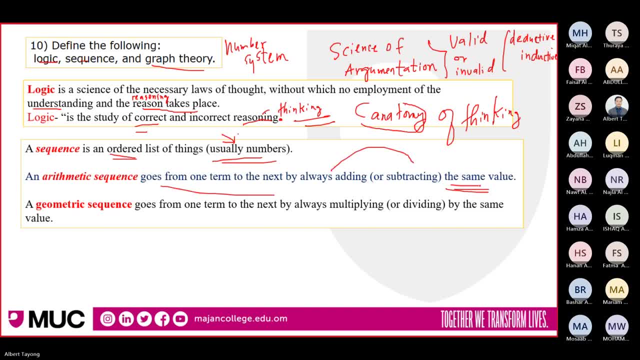 by adding or subtracting the same value. An example is eight, eight, 10,, 12,, 14 is arithmetic, Eight plus two, 10 plus two, 12 plus two, While a geometric sequence goes from one term to the next. 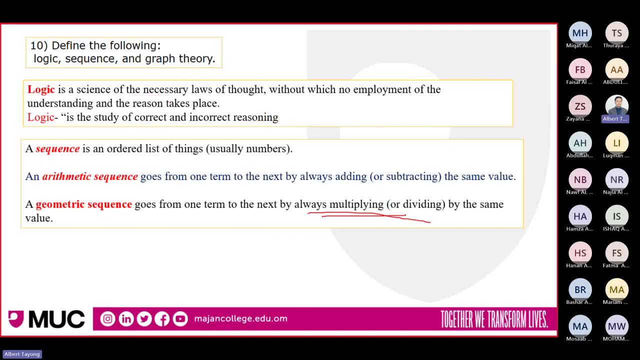 by always multiplying or dividing by the same value. Okay, same value. here is the D common difference, and for geometric sequence it is the R. Okay, here we have D the common difference, and here the same value in geometric sequence is the R. 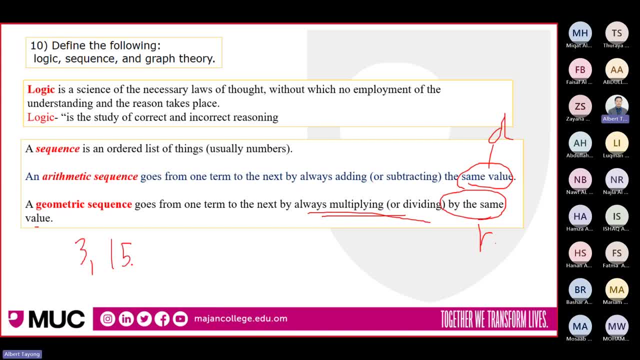 So it might be three, 15,. yeah, so multiplying by five. So three times five is 15,, 15 times five is 75. So this is an example of geometric sequence. It keeps on multiplying by five from one term to the next. 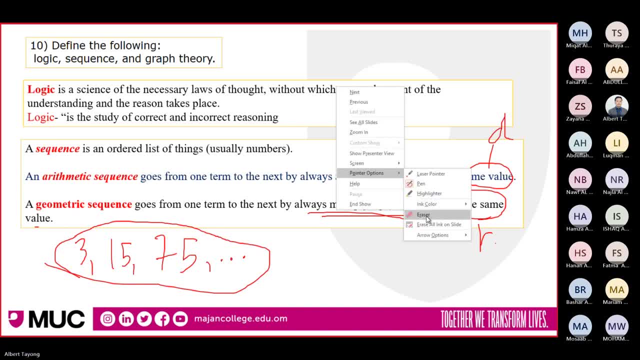 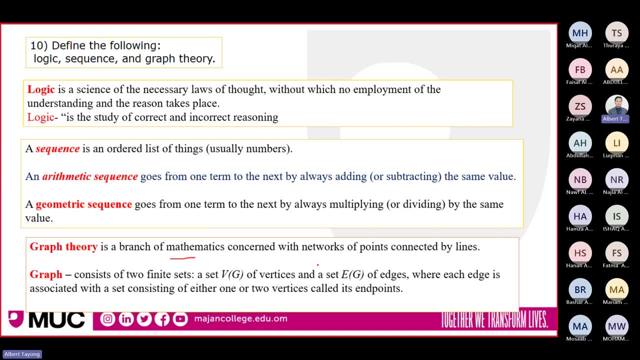 Back here. this is the R? U? 어�. In this caseenta to the left of three, we have a definite value. So you can see that this is the R? U and the C is perpendicular to this drugs. Now I'm going to stress both Halfs and Sim決ters. 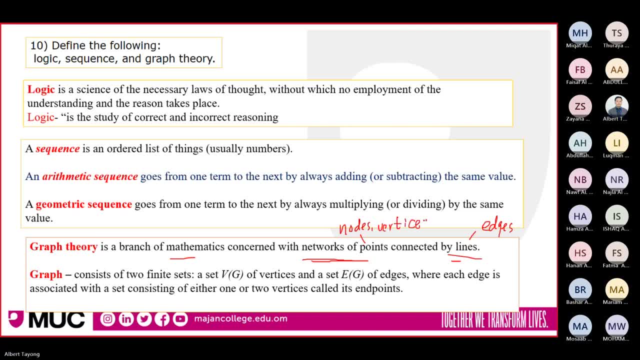 ности to be same, and I'll be using the model function because you have to have those functions come together. so, for example, the fruits are also called as vertices or nodes. a graph consists of two sets: set of vertices and set of edges. so these are the definitions you have to somehow familiarize for your multiple choice. 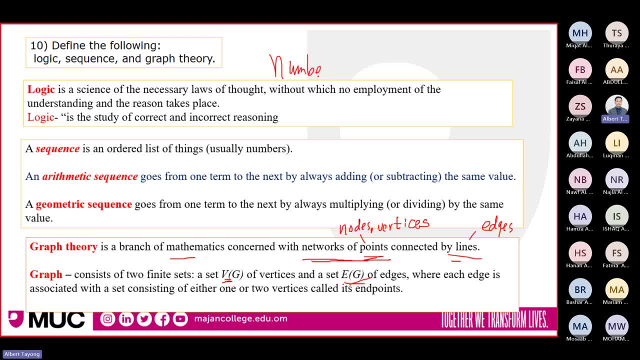 questions and try to search also the meaning of number system. of course you know number system. it is a writing system used to represent numbers using digits or symbols, or symbols, in a consistent manner. okay, so we use symbols or digits to represent our numbers. we use symbols because in some 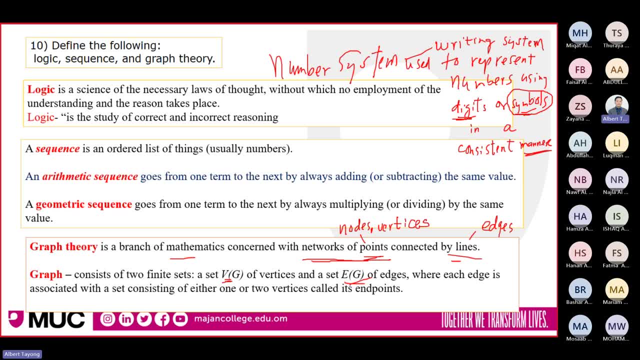 civilizations like the arab world. you have your own symbols to represent your digits and to represent your numbers consistent manner, because every digit has some meaning. nine has a place value, five has a place value, seven has a place value, so this is zero here. one and two, so there are seven hundreds. 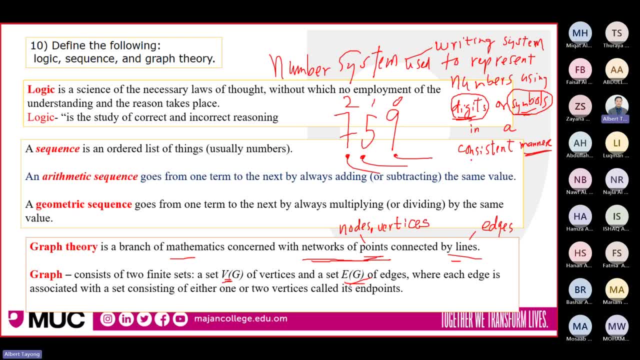 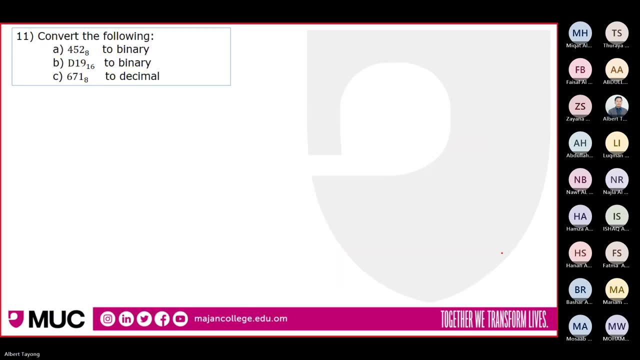 five tens nine ones. that's why we mention these words: consistent manner, because every digit has a place value. okay, so of course conversion will be there. for example, you're going to convert four, five, two base eight to binary. i gave this already a while ago an example of this. 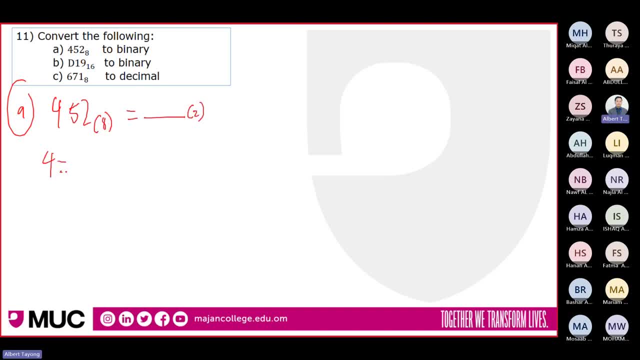 so four is four, two, one. five equals four, two, one and two equals four, two, one. whenever you see eight and two, use four, two, one, so this will be one. this will be zero and zero. we need only four, five. we need four and one, so this will be zero. four plus one is equal to five. 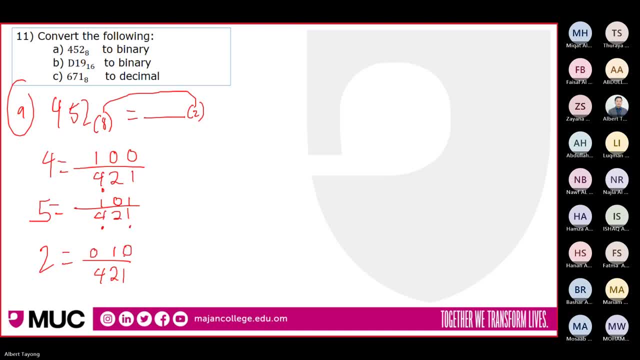 two. we need only the second digit: zero, one, zero. so the answer is: one zero, zero, one zero, one zero, one zero, base two. so this is the binary number for this octal number now. so this is the binary number for this octal number now. now, this one equals nine. 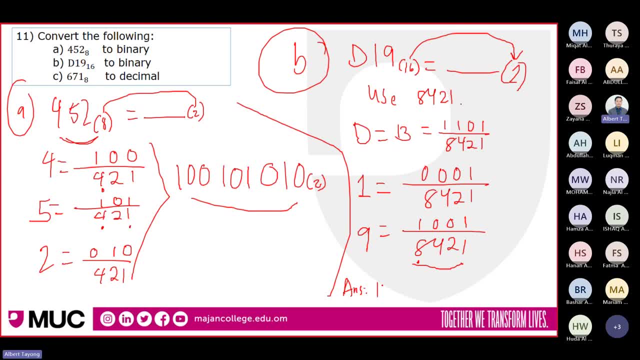 this one equals nine. so the answer is so. the answer is so. the answer is one one zero one zero zero, zero. one one one zero, one zero zero, one zero, zero. one one, one zero, one zero, zero, one, zero, zero, one one zero zero, one base two. one zero zero, one base two. 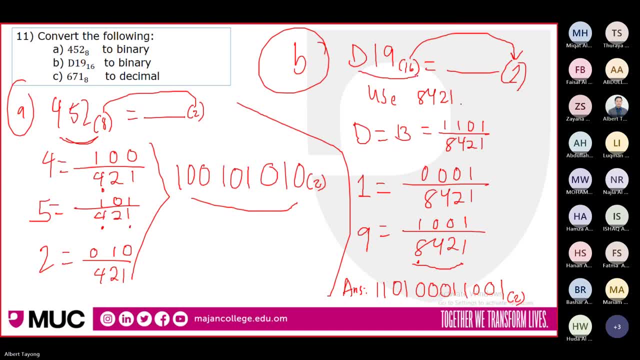 one zero, zero, one base two. so this is the binary number of this. so this is the binary number of this. so this is the binary number of this hexadecimal number. so please memorize, so, please memorize, so please memorize this, this, this, the highest is 15 f. 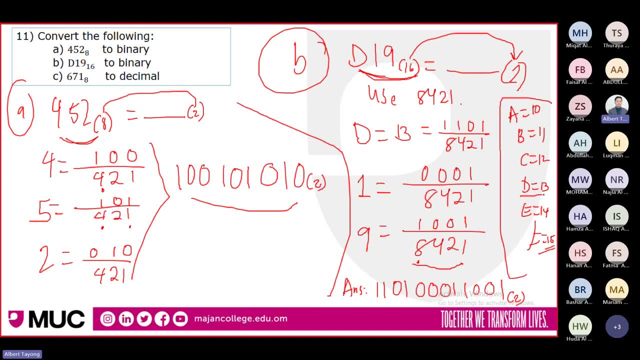 the highest is 15 f. the highest is 15 f, starting from 10 a, so d is 13.. the last one there is the last one. there is the last one. there is six, seven, one base, eight, two decimal. six, seven, one base, eight, two decimal. 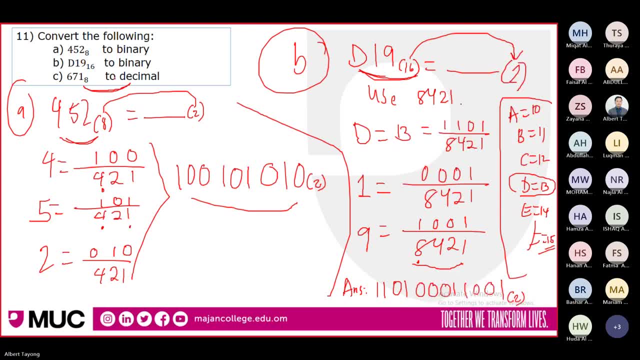 six, seven, one base eight, two decimal. so what are we going to do so? what are we going to do so? what are we going to do? six seven, one base eight. six, seven, one base eight. six, seven, one base eight. going to decimal 10. going to decimal 10. 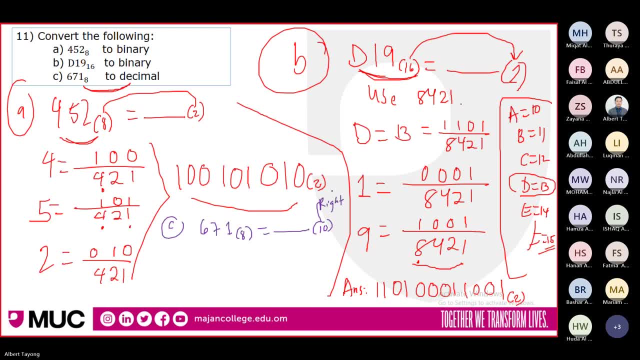 going to decimal 10. 10 is on the right, 10 is on the right, 10 is on the right. so what you will do, you will have. so what you will do, you will have. so what you will do, you will have zero, one, two going to the left. 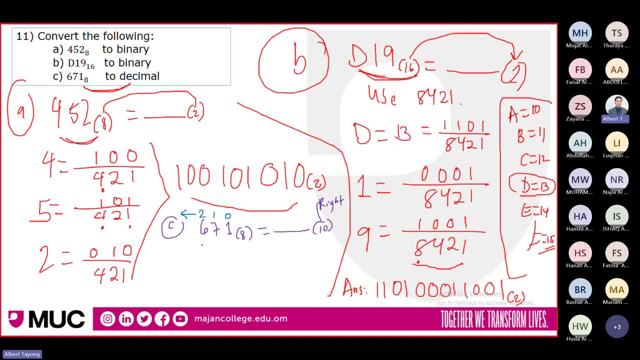 zero one, two going to the left. zero one, two going to the left. you can continue if there are more digits. you can continue if there are more digits. you can continue if there are more digits. zero one, two, three and so on. zero one, two, three and so on. 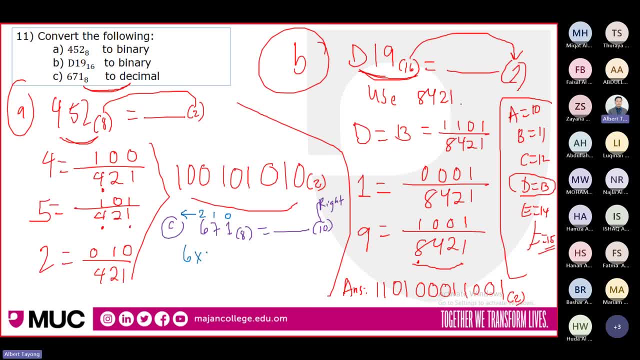 zero, one, two, three and so on. so six times, so six times. so, six times eight squared because you have eight here. eight squared because you have eight here. eight squared because you have eight here, plus seven times eight raised to the, plus seven times eight raised to the. 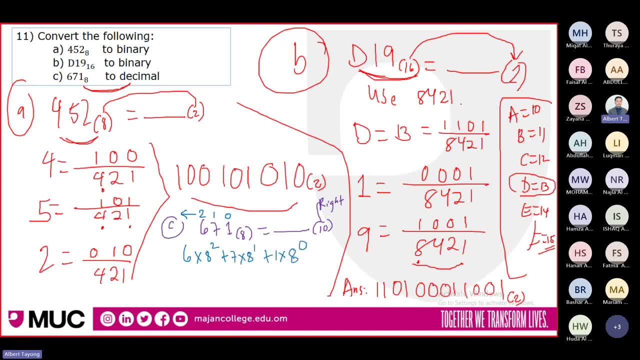 plus seven times eight, raised to the power of one, power of one, power of one plus one times eight raised to the power plus one times eight, raised to the power plus one times eight, raised to the power of zero of zero of zero, equals 441. okay, okay. 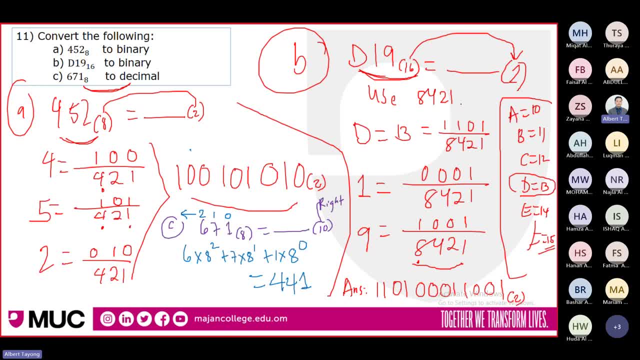 okay, so that is the answer for letter c. this is so. that is the answer for letter c. this is so. that is the answer for letter c. this is the answer for a. this is the answer for b. this is the answer for b. this is the answer for b and this is for c. 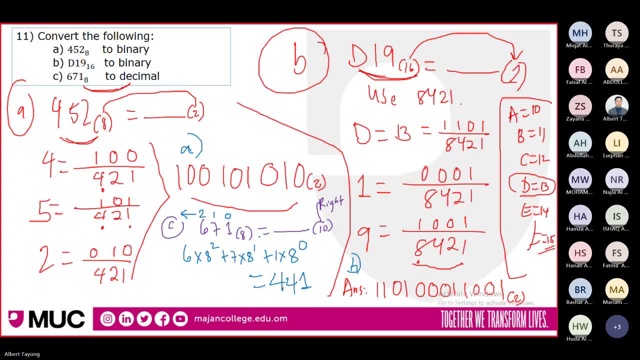 so be careful: here we have to use eight, we use eight. here we use eight here. we use eight here, because the base is eight octal, because the base is eight octal, because the base is eight octal. ten in the right, then on the right, you. 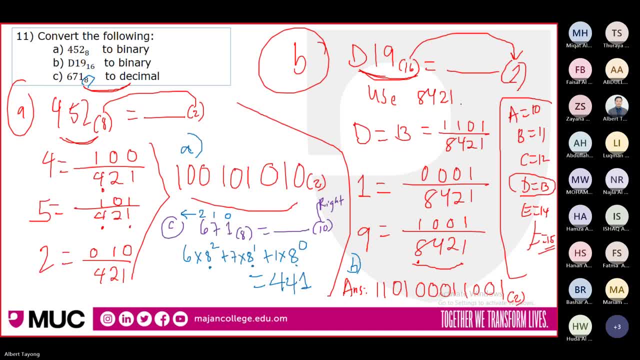 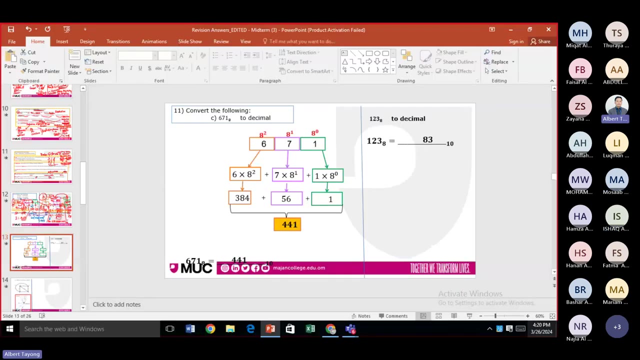 ten in the right, then on the right. you ten in the right, then on the right. you have to use this method. any question here. is this clear? is this clear? is this clear guys? no, thank you. yes, mr. okay, let's go to number 12.. okay, let's go to number 12.. 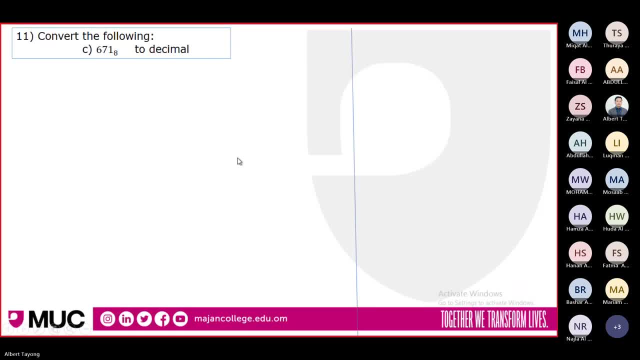 this one finished already. answer here is 441. yes, 11 c. i answered already. let's now have number 12. number 12: you are asked to short circuit three points: w, z and x- x. so we have here our w z- x, so maybe you can put it here. 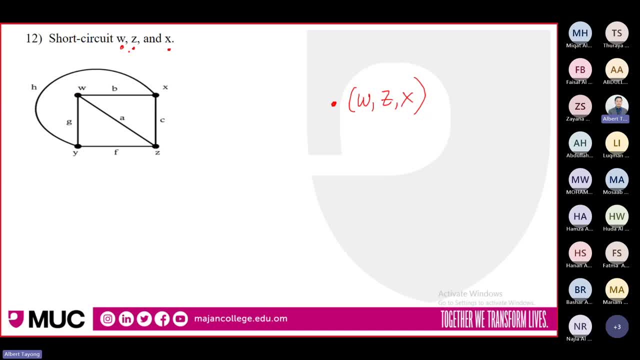 so w, z and x will be now one point, and your y, so you can put your y here. so now we have only two points. originally we have four points: w, y, z, x, but we are going to short circuit these three, so now it will, it will become one. 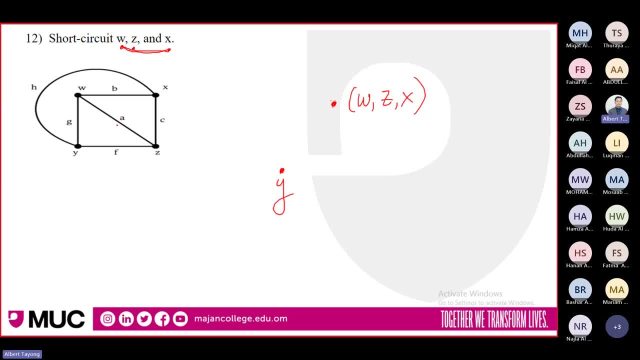 so let's start with a so we will not be confused. a is from w to z, so w and z are together. so what will happen? loop? yes, will become a loop. this is your a. okay, fix this all right. so let's go to our b. b is w to x. 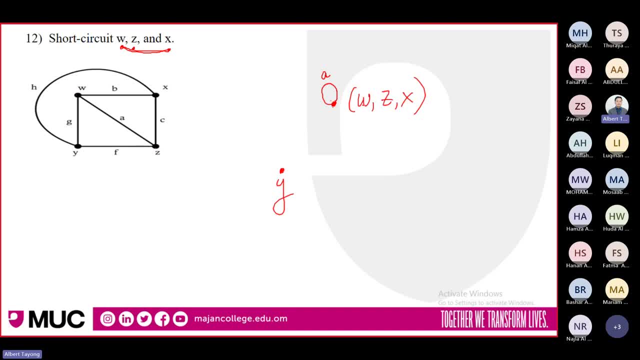 again, w and x are together, so it will be a loop again. this is our b. our c is x to x to z. again x and z are together, so it will be another loop. this is our c. now we have here also g and f, g and f. 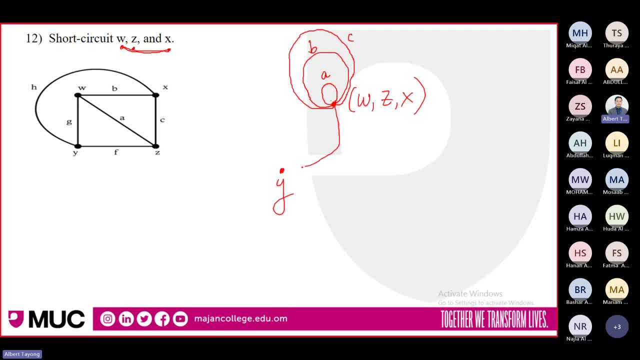 from W to Y. so W to Y is your G and F is Y to Z. okay, this is our F, and we have here H. H is from Y to X, so this is our H. so all in all we have six edges, three loops and three multiple. 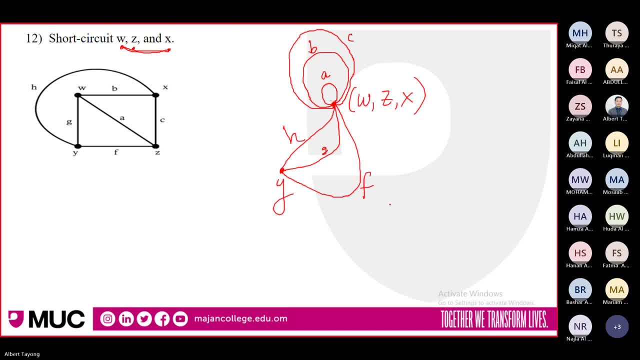 edges. so this is our answer. okay, is this clear? any question here? I think no question here. okay, number 13. number 13: you're going to draw the complement. we have one, two, three, four, five: the complement will have the same point. we have one, two, three, four, five: the complement will have the same point. 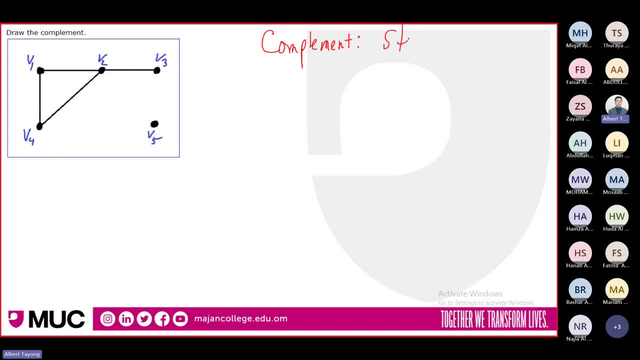 so please take note that step one is to label all the points. that's your step one. so V1, V2, v3, this is v4 and this is your v5. okay, so we are done with step one. v1 is connected to two and four. 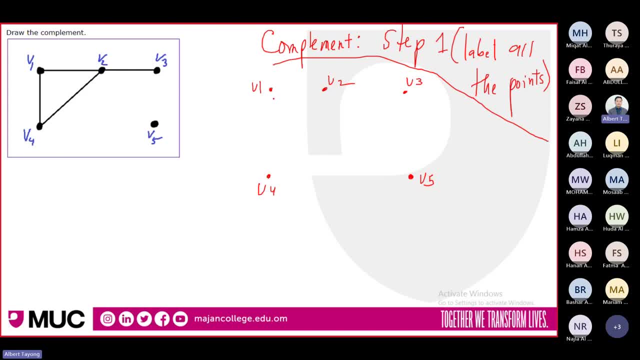 so the opposite is three and three and five. we deleted from v1 to v4. that edge is deleted, then v1 to v2- deleted. v2 is connected to one, four, three. the opposite is only five. five v3 is connected only to two. the opposite is one, four, five, right, yeah, but already is connected to one. 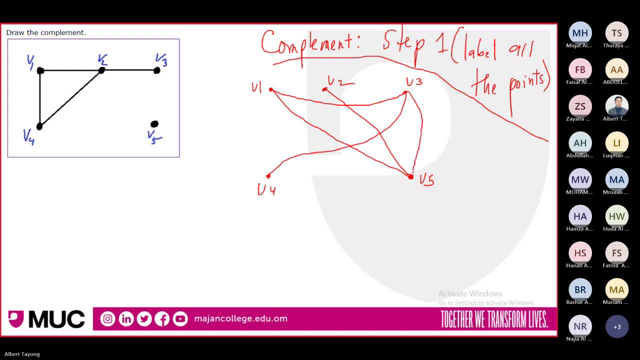 so connect to four and five. v4 is connected to two and one. it should be connected to three and five. yes, yes, yes, v5 is not connected to anything now it should be connected to all. so this is the answer already, because five is connected to all. 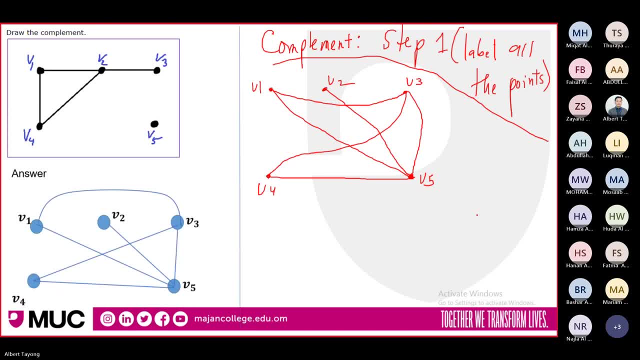 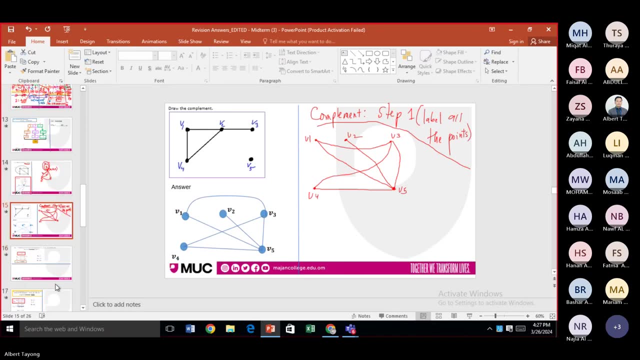 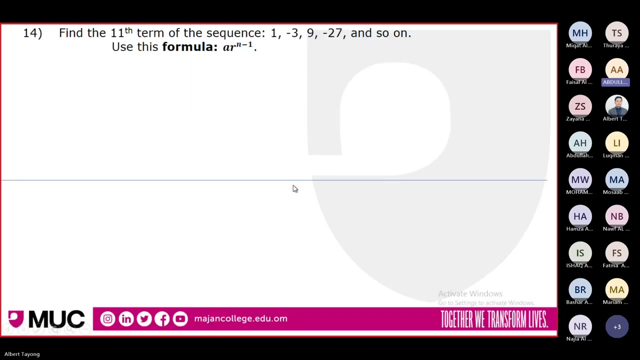 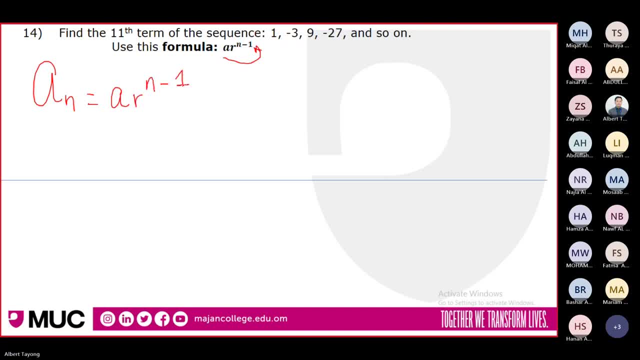 raised to the power of n minus one. so we have to start with a. our a is one equal to the first term, r. you know the formula: a sub 2 divide a sub 1. so a sub 2 is negative 3. divide 1 equals negative 3. 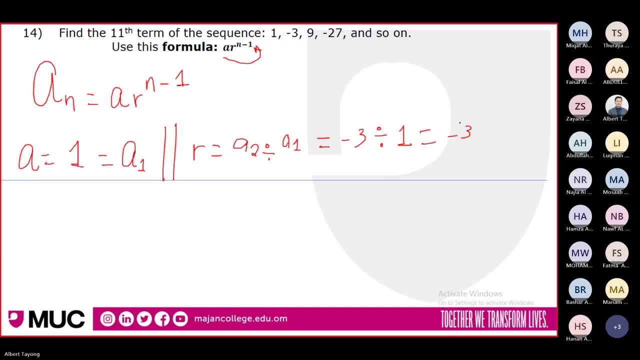 okay. so the question is: find the 11th term. so it means we have to find a sub, a sub 11. so our a is one, r is negative, 3 raised to the power of 11 minus 1. so we have to find a sub. 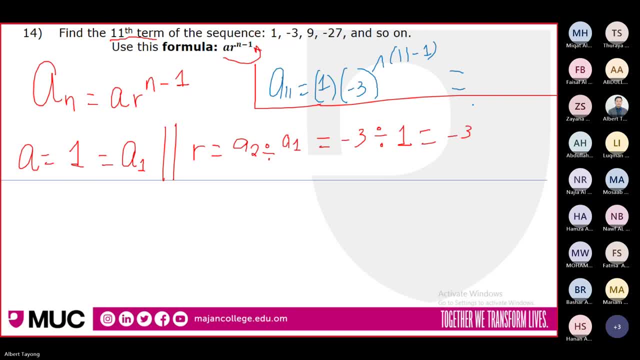 n equals a sub 2. okay, so our a is one, our r is negative 3, our n is 11, 11 minus 1. so the answer is 59049 59,049. can you please check this out in the calculator? yes, correct, there's a minus. 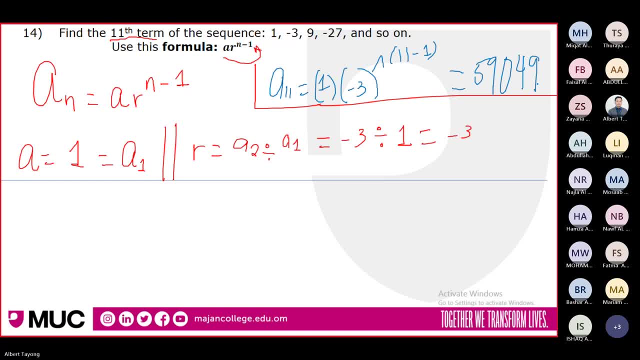 where? and minus 590. no, this one is positive. yes, positive because negative 3 raised to the power of 10 will be positive. yes, yes, because even number, even number, any exponential expression with an even, any exponential expression with an even number, will give you a positive answer. 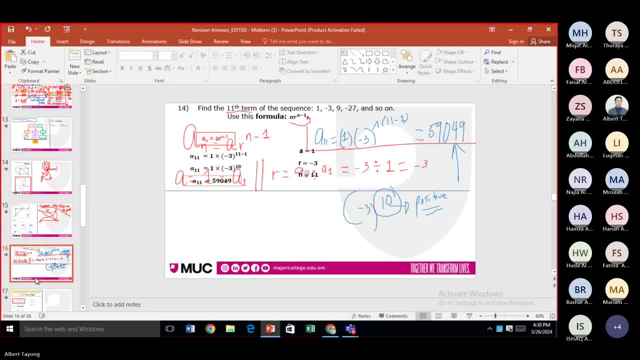 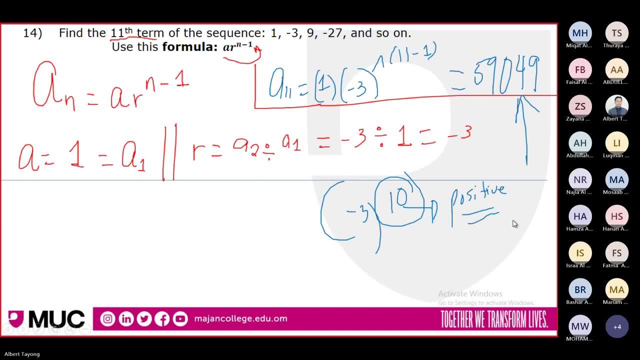 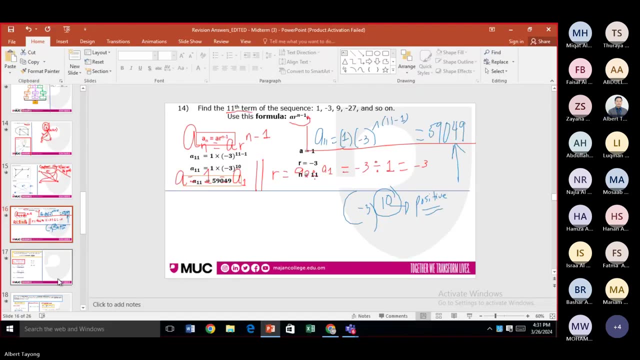 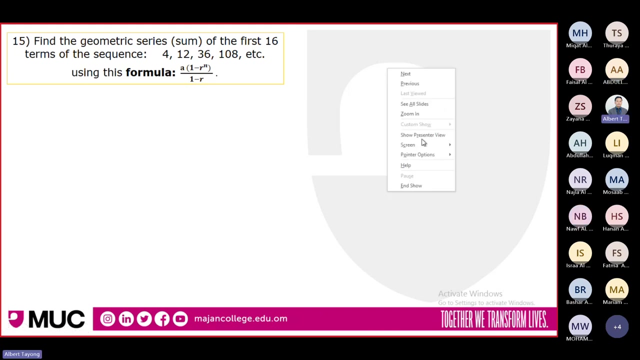 answer: okay. so this one is clear. so this one is clear. it's easy, right? it's easy, right. okay, so this one is clear, it's easy, right. okay, here you're going to find the geometric series. whenever you see the word series in arithmetic or geometric sequence, you are finding the sum. 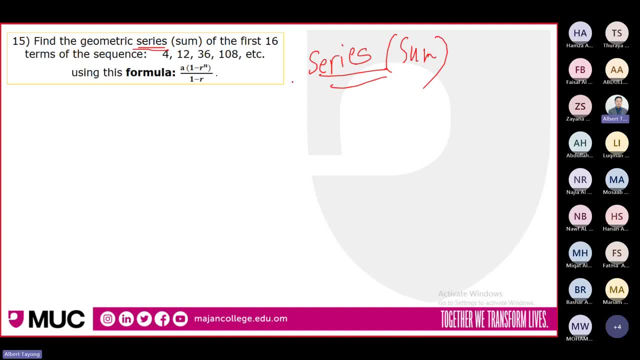 the geometric series of what first, 16. so the question is: s sub 16? the first is 4, followed by 12, 36, 108, dot, dot, dot, etc. so get your a. a is 4. this is the first, or a sub 1. our R is a sub 2 divided by a sub 1. well, divide 4, yes, very good. 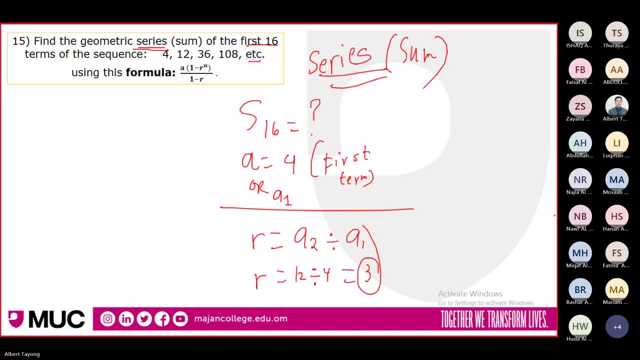 3, so we can immediately plug these values using the formula. the formula is given, so we have s sub n, because we talk about series, or sum equals a times 1 minus R raised to the power of n here. don't forget open and close here, although the formula has no open and close. 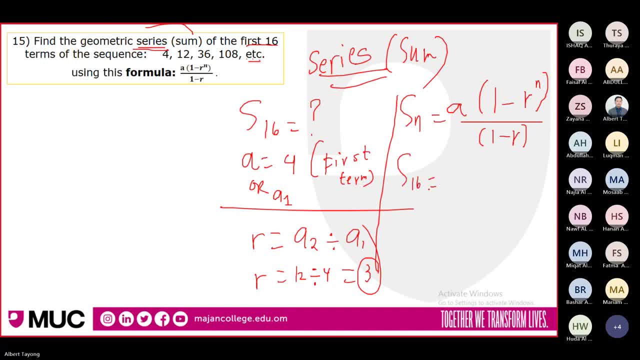 so the question is s sub 16, because geometric series of the first 16, our a is 4 times 1 minus 3, 3 raised to the power of what 16 a. what's the answer? Abdullah, what's the answer? hmm, well, what's the answer? 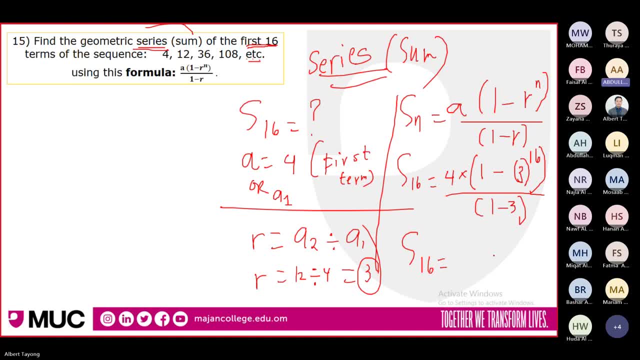 yeah, this is a very good answer. second: 2: ok, one 2. total: 86093440. very good, so the answer is 86 million ninety 3440. ok, so later. very simple. your exam is very simple piece of cake. yes, can i proceed to the next? 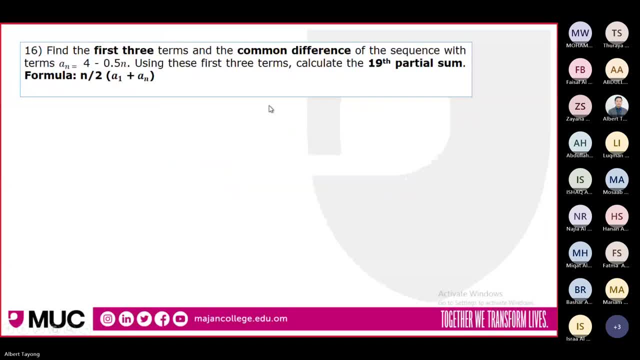 look man, look man, is there? okay, number 16: find the first three terms and the common difference of the sequence with a sub n equals 4 minus 0.5 n, so the n term is given already. this is our n term is given. we have 4 minus 0.5 times n, so find the first three terms. so that means you have to find a1. 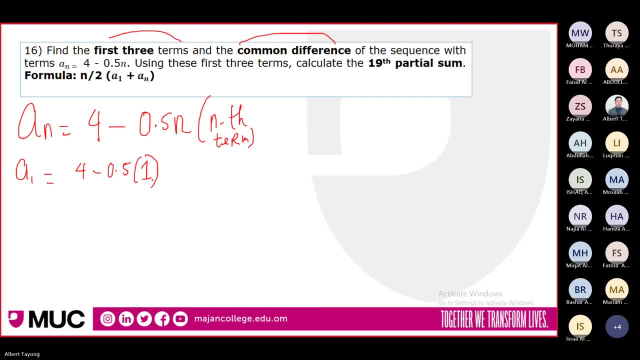 4 minus 0.5 times 1.. okay, so the answer will be 3.5. then a sub 2 equals 4 minus 0.5 times 2 equals 3. okay, then a sub 3: 4 minus 0.5 times 3, so basically we just change our n. 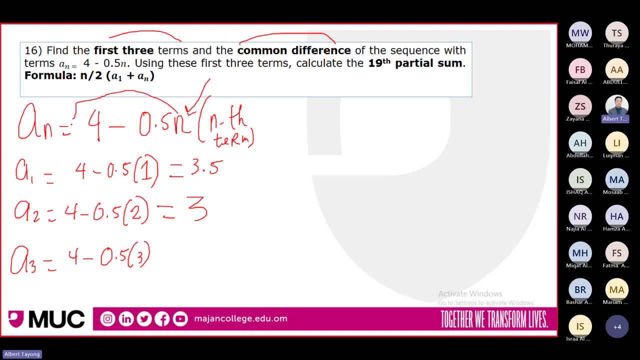 our n, we have to change one and two and three. now, here was the answer. did you get 2.5? so the first three terms are 3.5, 3, 2.5. right now, what is the common difference, guys? what's the common difference? 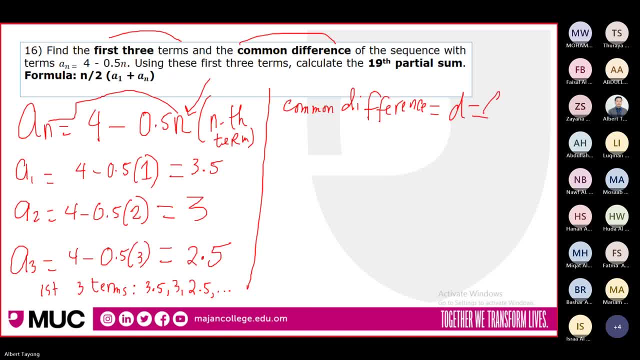 0.5. very good, a sub 2 minus a sub 1. so our d equals 3 minus 3.5. so negative 0.5. what the negative? what's up? negative 0.5, yeah, yes, yes, okay, okay. now calculate the 19th partial sum. 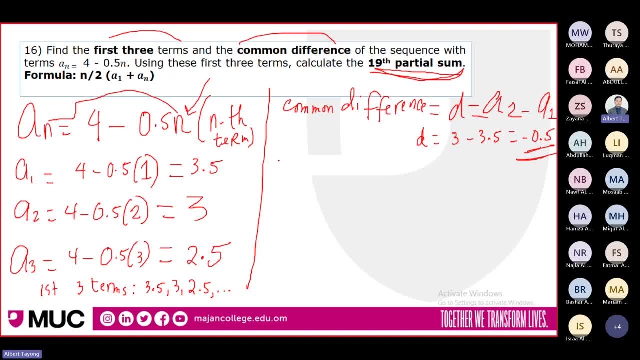 okay, now calculate the 19th partial sum. so it means we have to find s sub 19.. that's the question: 19th partial sum. every time we are only having partial sum, because this will keep on going, a sub one, a sub two, until infinity. 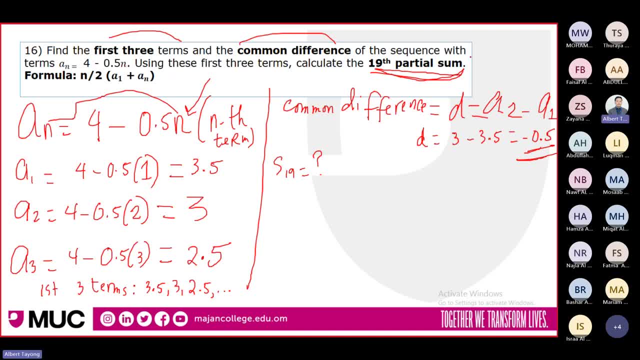 so most of the series values are only partial. you cannot add all formula is there and over 2. this is the formula for arithmetic, series arithmetic because you have common difference. so it means we have to find a sub-19 first. this one, a sub-19, is 4 minus 0.5 times 19. so what is the answer? 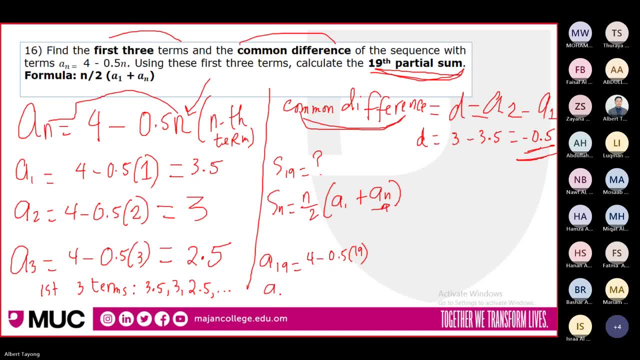 minus 5.5, yes, negative 5.5. okay, so now we can solve s19: 19 over 2. a sub 1 is 3.5 plus negative 5.5. okay, so now we can solve table. so what's the question? 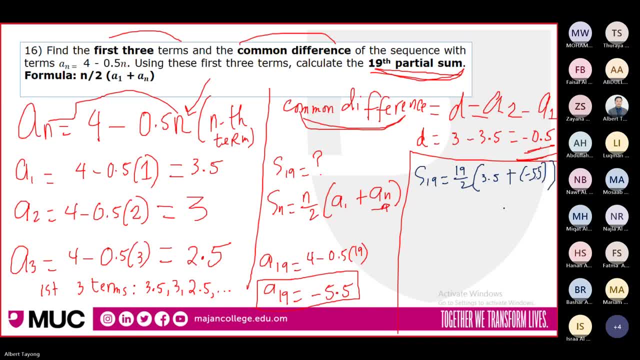 table. how do we fit the sum? so yes, alright. so what's the value? the side of the formula quotes. so what's the value? side of the formula? negative 1. so 19 times negative 1 equals negative 19. so the answer is negative 19.. 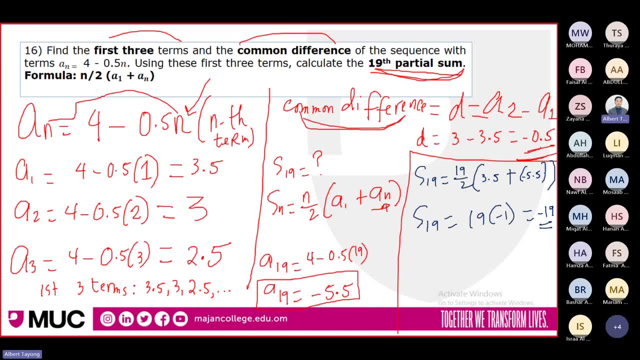 okay, is that clear guys? 19, i think 9.5. the answer is negative, 19.. no, before i said: how come nine? what is nine? there is no nine here. this is 19 here. yeah, why i'm? i'm use this uh 4 minus 0.5 to get 19th number. 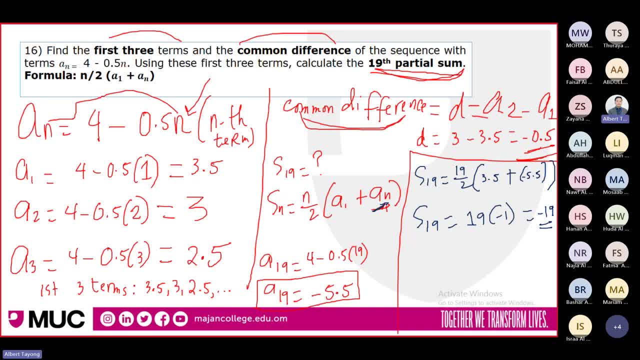 because we have a sub n here, this one, this is negative 1. what is our n? what is our n? what is the question? 19? yes, 19 partial sum. so we have to find a sub 19 first. put it here: a sub n, the a sub n. what is our n here in s sub 19? 19, right? 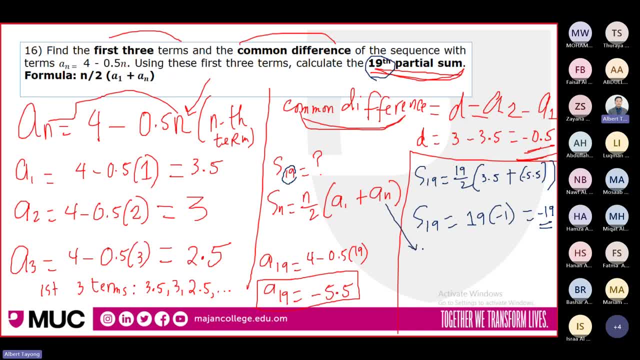 yes, so a sub n is a sub 19. that's why we need to find that value. okay, I'm asking this, yeah, I'm asking this step, why I use this specific thing and why I'm not use a for 3.5 minus. oh wait, see, we have a sub 1 here, right, yes, a sub 1 already. we know what. 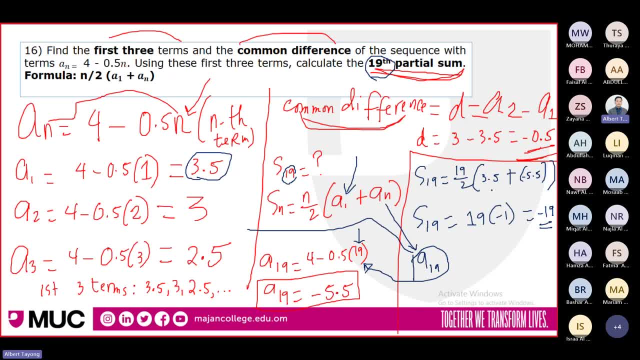 is the value save and slide. so we have here: this is a sub 1, a sub 1, this one, this one is a sub n, is a sub n. the aja n is not this sub 1. a sub n is the ace of 19.. 19, because you have 19 partial sum. okay, so this n here will be 19. 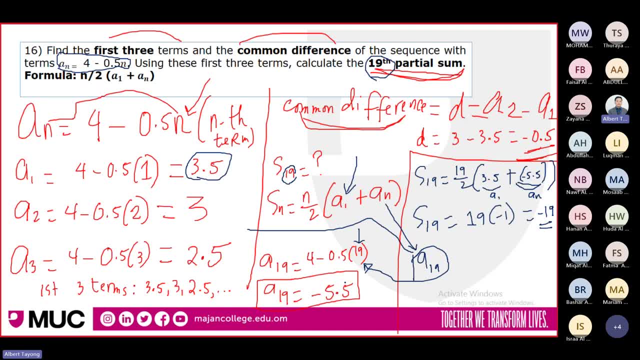 so the value is negative 5.5. using the formula: the formula is given 4 minus 0.5, n. change n to 19, so the value is negative 5.5. that is your a sub n. a sub 1 is 3.5. 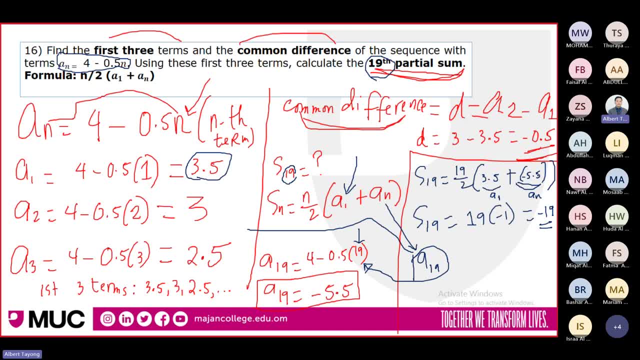 plus a sub n is negative. 5.5. n over 2 is 19 over 2, so 19 over 2, 19 will be at 2 will be cancelled. yes, so the remaining is negative 1, or you can use your calculator directly. you're going to get negative 19.. 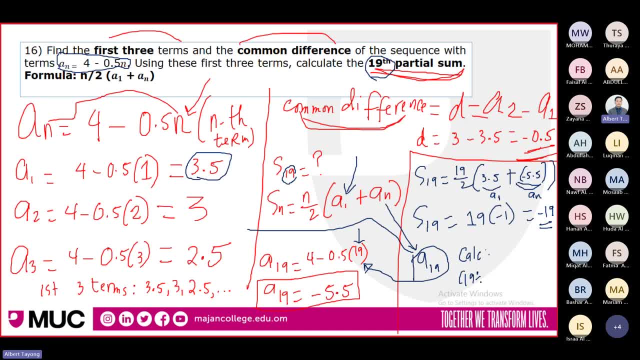 the calculator, you will have 19 divided by 2 times 3.5. minus 5.5, because this is plus, negative will become minus here. okay, immediately you're going to get negative 19.. did you understand, musab? yes, so basically for the arithmetic series. first you find a sub n- this one. the n here is this one, 19. 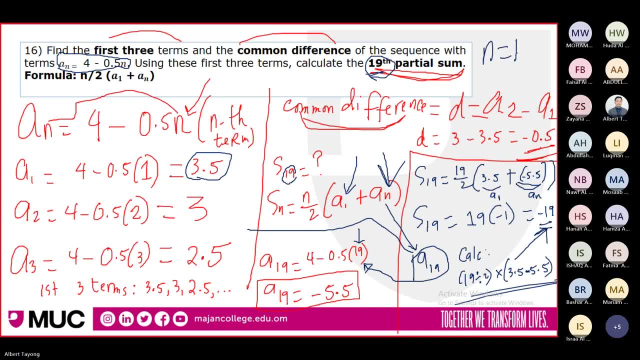 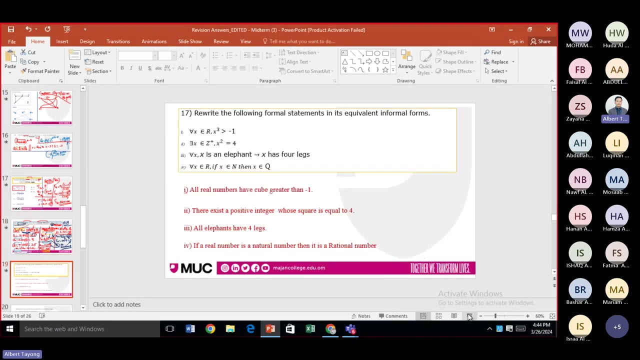 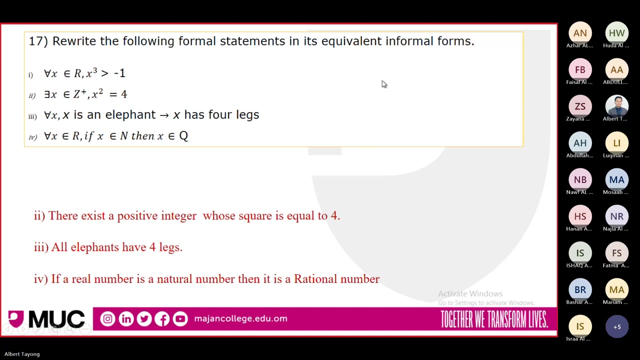 partial sum. so n is 19.. so you have to find a sub 19 using the given nth term: 4 minus 0.5 n, whatever is given. okay, let's have number 17 for number 17. i will discuss this again during the support class on thursday. 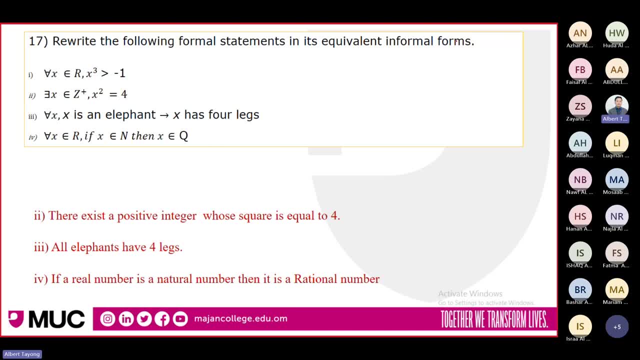 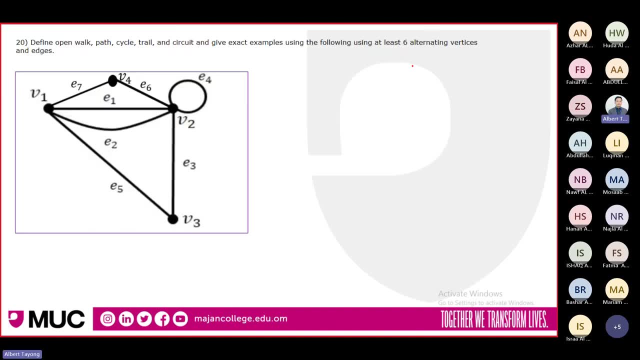 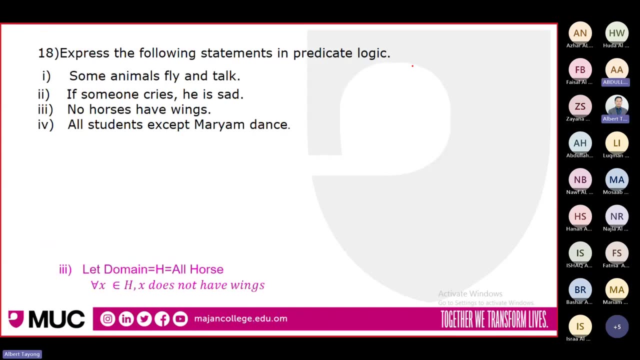 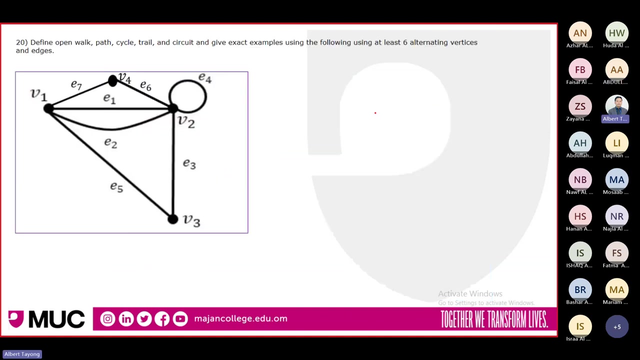 okay, we are almost done. 17 and 18. this will be part of the support class on thursday: number 19: deductive inductive. already we know this. 20 is what is? what is the support class on thursday? number 19: deductive inductive. already we know this. 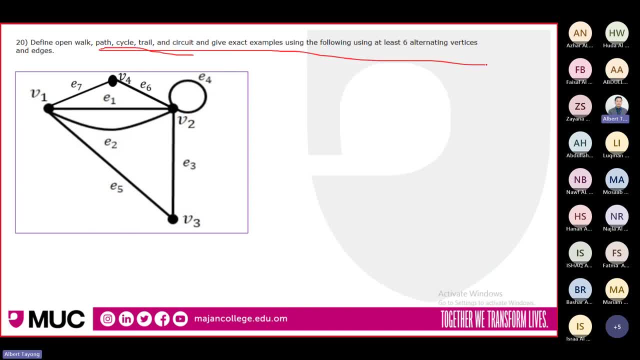 open walk path cycle. we have a lot of open walk path cycle. we have a lot of open walk path cycle. we have a lot of examples of this. examples of this, examples of this- last time, so i will discuss that later. last time, so i will discuss that later. 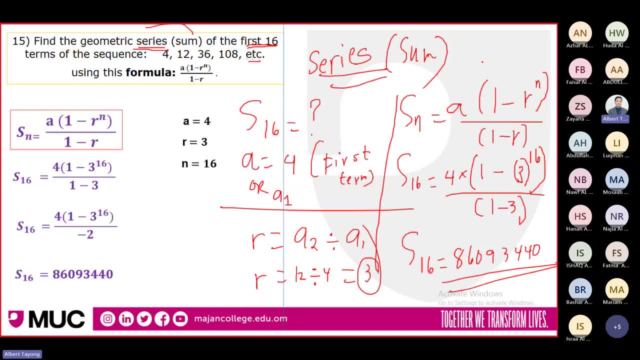 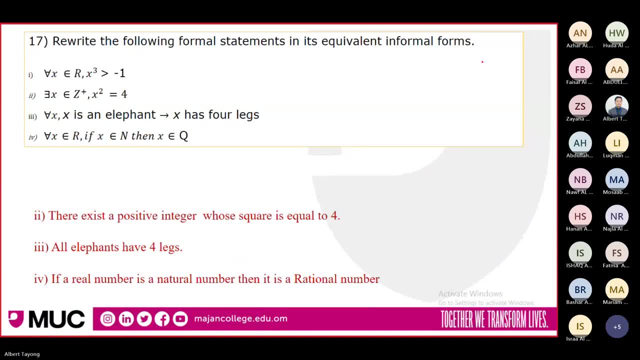 last time, so i will discuss that later. okay, let's have number 17. anyway. i will give more examples on anyway. i will give more examples on anyway. i will give more examples on thursday for thursday for thursday for number 17 and 18.. 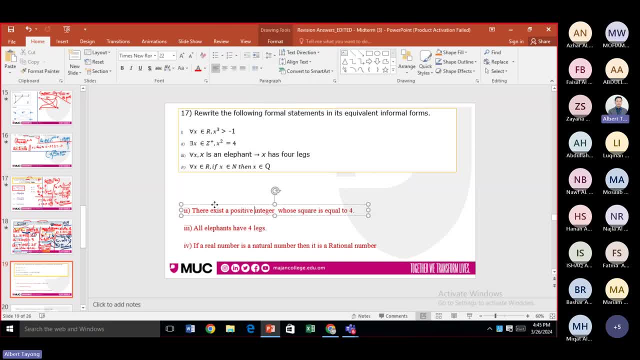 so please attend the support class. so please attend the support class. so please attend the support class. we had a lot of support class this. we had a lot of support class this. we had a lot of support class this semester semester. we had a lot of support class this semester. 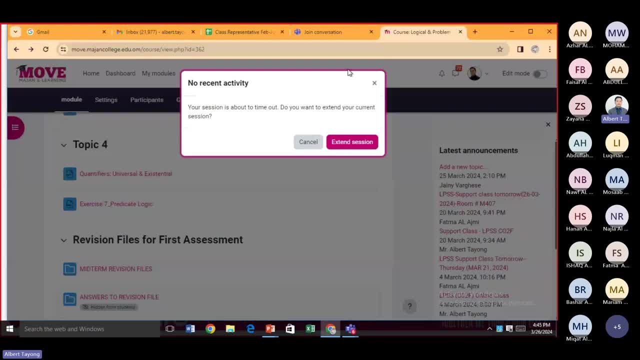 okay for thursday, we will be talking. okay for thursday, we will be talking. okay for thursday, we will be talking about this. topic four, although i sent you the video. topic four, although i sent you the video. topic four, although i sent you the video already. 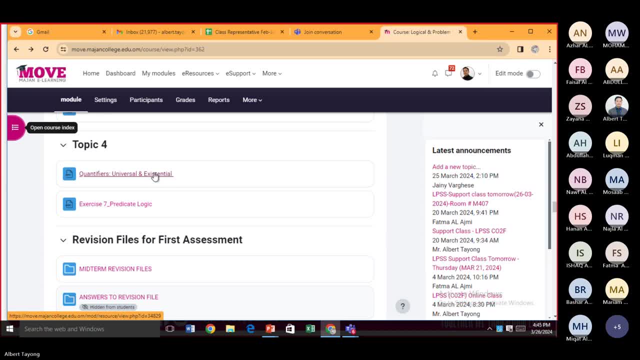 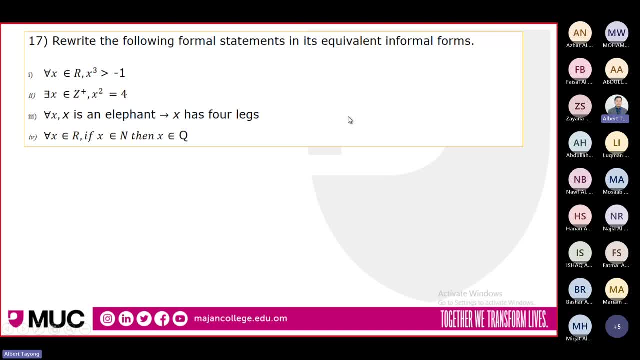 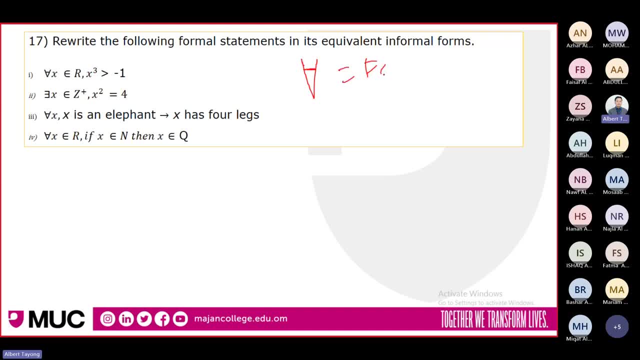 all right. so whenever you see this symbol, it's like a inverted, it's like a inverted, it's like a inverted. it means for all. it means for all. it means for all. this is this is this is what we called as universal. what we called as universal. 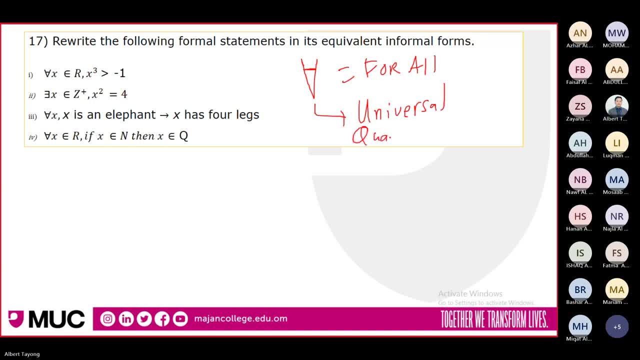 what we called as universal quantifier. universal quantifier means universal quantifier means. universal quantifier means we include all the elements universal. we include all the elements universal. we include all the elements universal. so the keywords are so, the keywords are so, the keywords are all all. 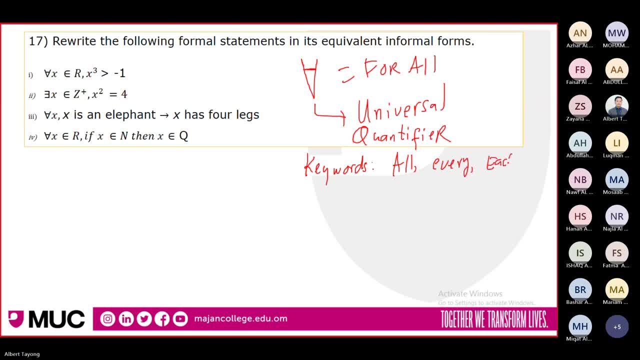 all, every, every, every, each, each, each, any, any, any, anything, anything, anything, everything. but the most common are these two: all. but the most common are these two: all. but the most common are these two, all, every, every, every, every. so it means you include all the elements when. 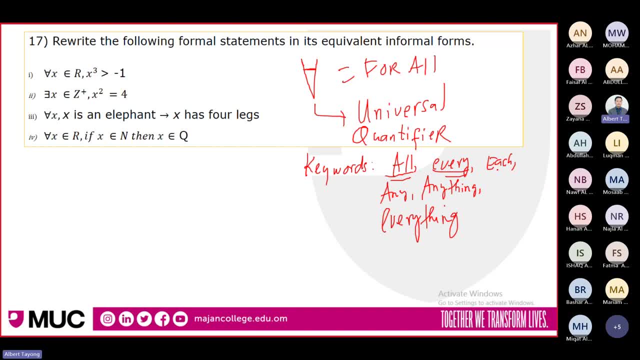 so it means you include all the elements. when- so it means you include all the elements. when you say every student, you say every student, you say every student. that means all students, that means all students, that means all students, universal, universal, universal. but it depends on the problem you're. 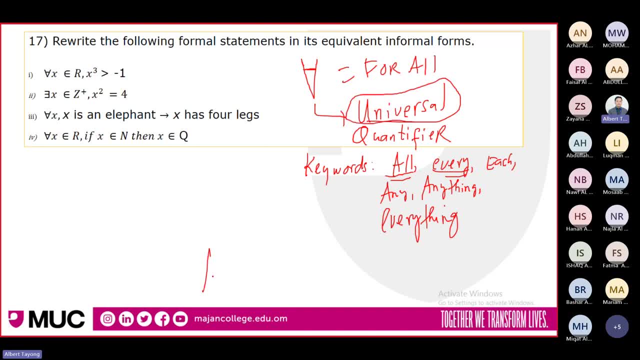 but it depends on the problem you're. but it depends on the problem you're talking about talking about. talking about when you say all students, when you say all students, when you say all students, if you don't mention where, if you don't mention where, if you don't mention where, it means all students in the world. 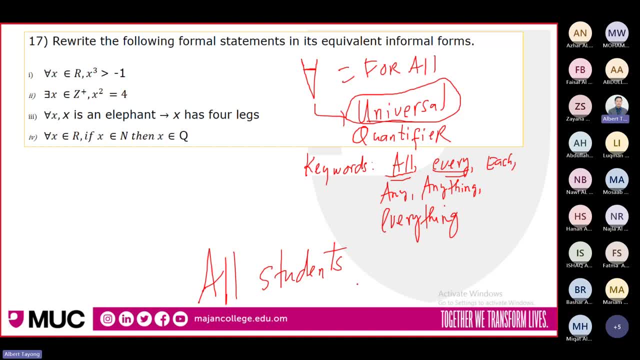 it means all students in the world. it means all students in the world, but you can also say all students at. you can also say all students at. you can also say all students at muc, muc, muc. this one is also universal. this one is also universal. this one is also universal, but only. 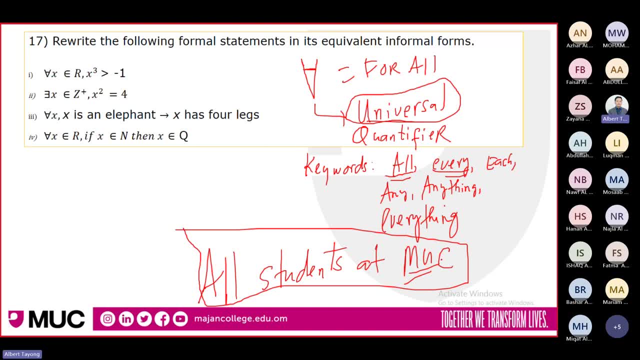 but only, but only here. okay, excuse me, okay, excuse me, okay, excuse me now, please take note of these letters. now, please take note of these letters. now, please take note of these letters. r means real numbers. r means real numbers. r means real numbers. memorize them, memorize them. 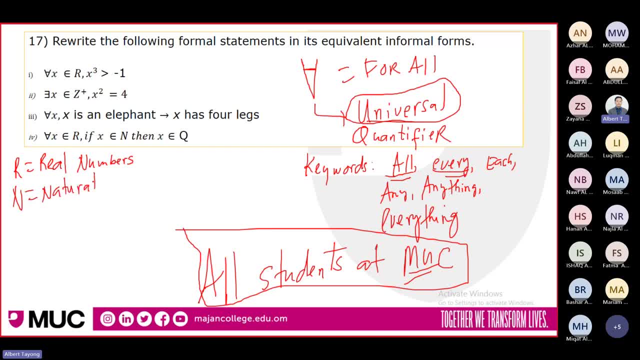 memorize them. n is natural numbers because you're n is natural numbers because you're n is natural numbers, because you're going to use this, in going to use this, in going to use this in the exam. natural numbers, also called as counting. natural numbers, also called as counting. 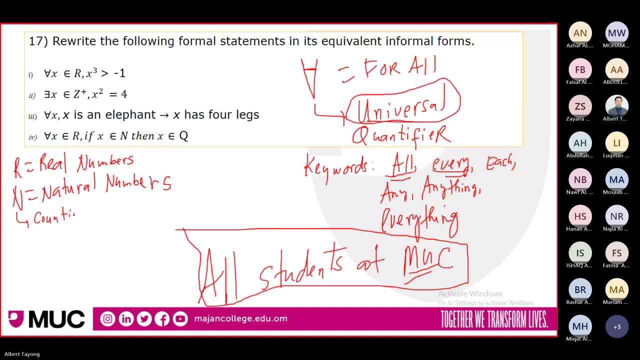 natural numbers, also called as counting numbers: z plus positive integers, z minus negative integers, z minus negative integers, z minus negative integers, of course z integers okay, w whole numbers: q, rational numbers, q rational numbers, q rational numbers. these are the common symbols in. these are the common symbols in. 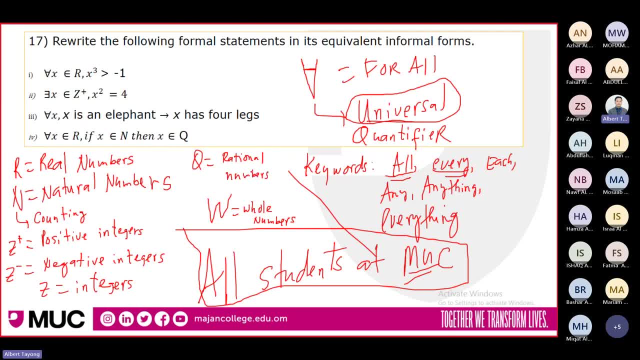 these are the common symbols in mathematics, mathematics, mathematics. in your foundation. all of these are discussed in your foundation. all of these are discussed in your foundation. all of these are discussed. i'm just repeating it here. i'm just repeating it here. i'm just repeating it here. okay, so q rational numbers w. 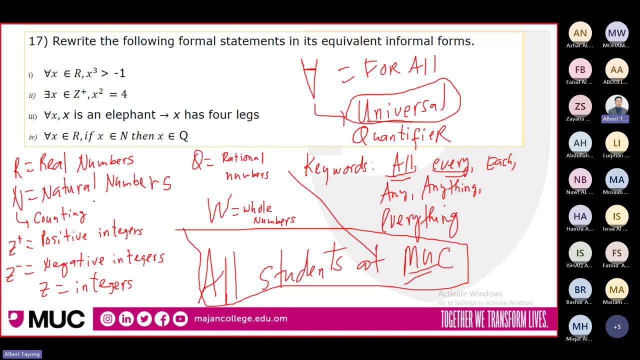 okay, so q rational numbers w. okay, so q rational numbers w whole numbers, whole numbers. whole numbers n counting or natural numbers. n counting or natural numbers n counting or natural numbers. positive integers z plus positive integers z plus positive integers z plus negative integers. negative integers z plus negative integers. 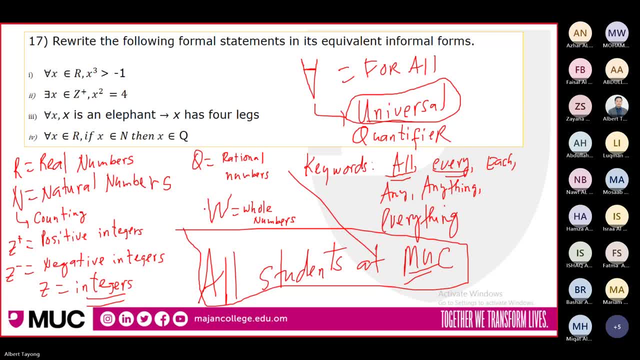 negative integers z plus negative integers z minus z integers, z minus z integers, z minus z integers. okay, the first one. okay, the first one. okay, the first one. we are changing from formal statements. we are changing from formal statements. we are changing from formal statements to informal, to informal. 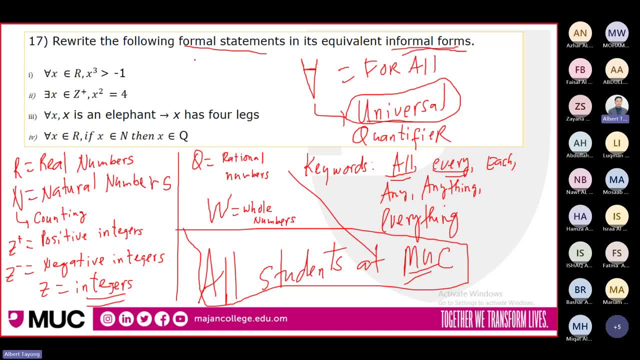 to informal statements. same logic: formal statements are statements. same logic: formal statements are statements. same logic: formal statements are the: the: the symbolic, symbolic, symbolic, the predicate form. the symbolic form is the formal. the symbolic form is the formal. the symbolic form is the formal. the informal forms are the. 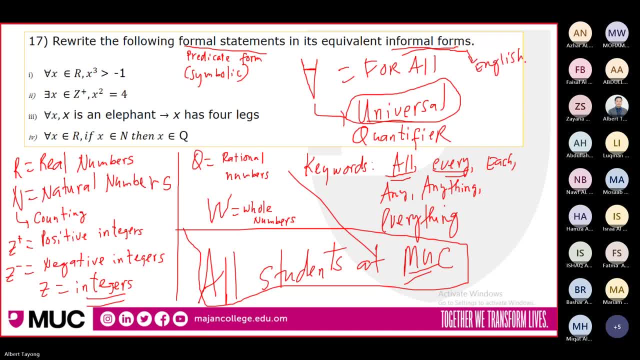 the formal forms are the formal forms. are the? the formal forms are the formal forms. are the english sentence or statements: okay, so, please take note of that. okay so, please take note of that. okay so, please take note of that. when you ask, when you're asked to rewrite. 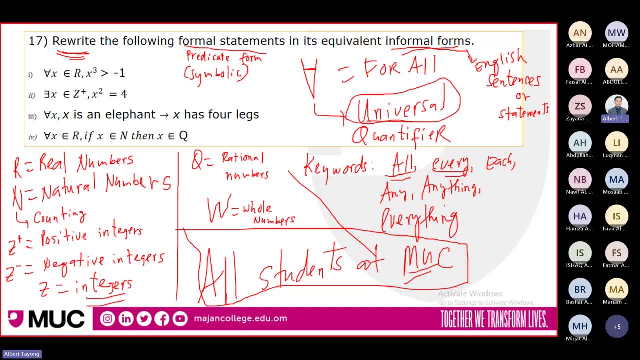 when you ask, when you're asked to rewrite, when you ask when you're asked to rewrite, when you're asked to rewrite, from when you're asked to rewrite, from when you're asked to rewrite from formal formal. formal to informal. it means from symbolic to informal. it means from symbolic. 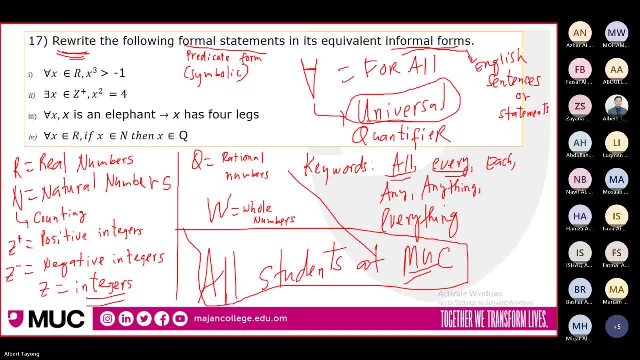 to informal. it means from symbolic to english sentence, to english sentence to english sentence. so this one is symbolic, so this one is symbolic, so this one is symbolic for all x in r, for all x in r, for all x in r. e here is element of, e here is element of. 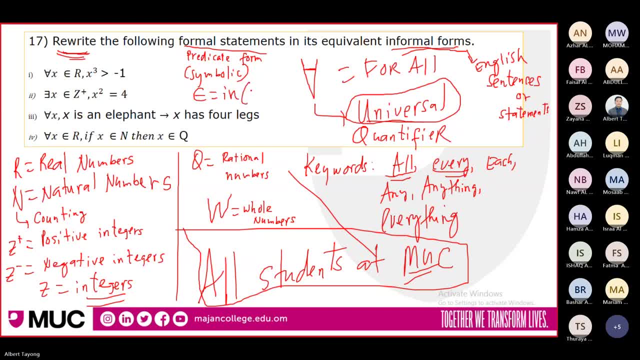 e here is element of, but we just say in, but we just say in, but we just say in: element of, element of, element of. it means it means it means it's part of that set, it's part of that set. it's part of that set, okay. 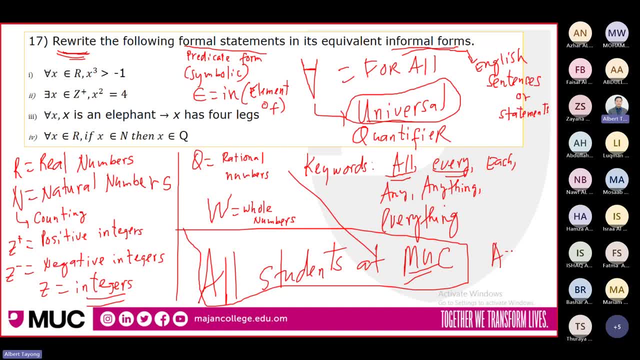 it's inside, it's inside, it's inside. and we have, for example, a equals five, and we have, for example, a equals five, and we have, for example, a equals five, six, seven, six, seven, six, seven. five is an element of a. six is element of a. five is an element of a six is element of a. 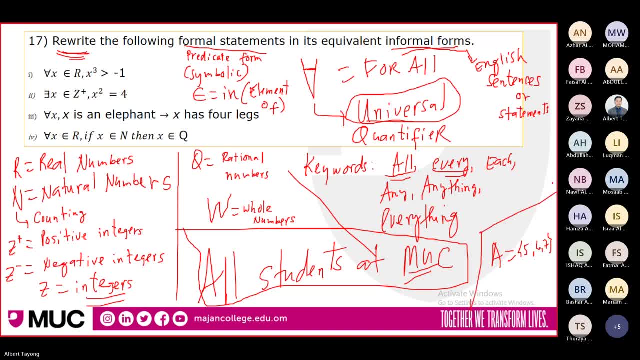 five is an element of a, six is element of a. seven is an element of a, is inside. seven is an element of a, is inside. seven is an element of a, is inside. so we usually use in, so we usually use in, so we usually use in. so for all: x in r comma, x, cube greater. 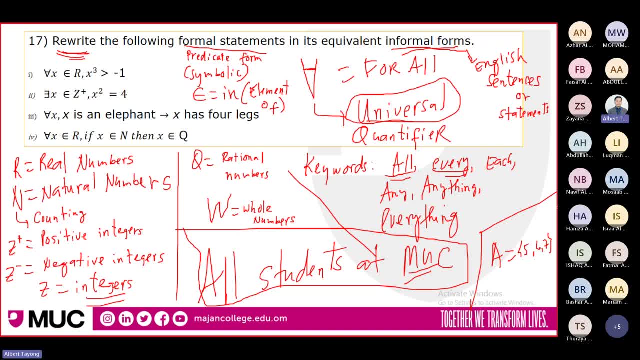 so for all x in r comma x cube greater. so for all x in r comma x cube greater than negative one, than negative one, than negative one. so how do we change this? so how do we change this? so how do we change this from left to right? 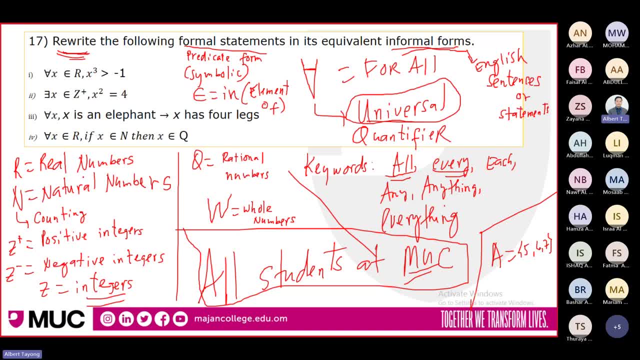 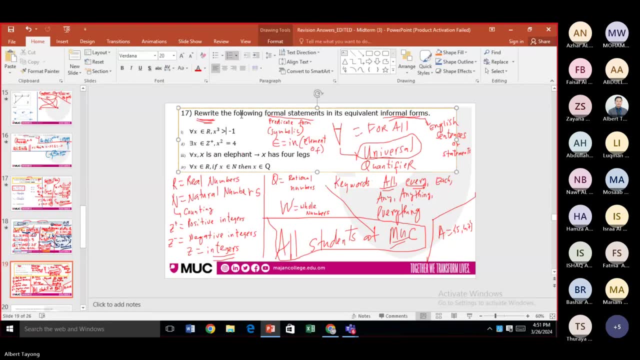 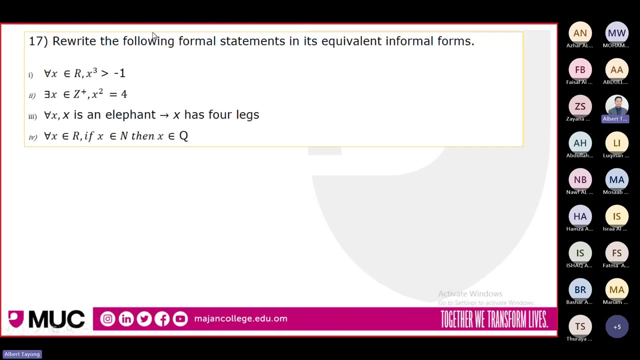 from left to right, from left to right, using the words here, using the words here, using the words here: r n z plus r n z plus r n z plus z minus z q w. okay, so let's answer that letter or number one. you say all letter or number one, you say all. 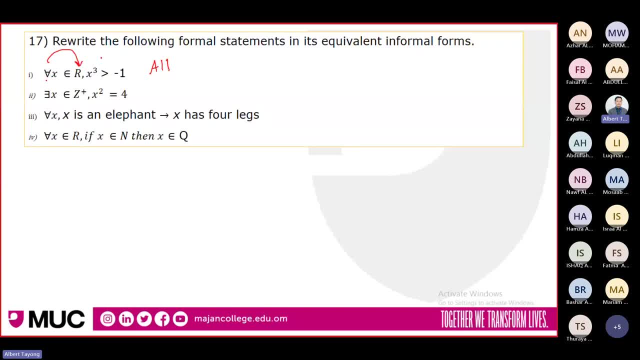 letter or number one. you say all because of this symbol left to right, because of this symbol left to right, because of this symbol left to right, then proceed here, then proceed here, then proceed here, all real numbers, then have, then have, then have, cubes, cubes, cubes. tub s greater than negative one. 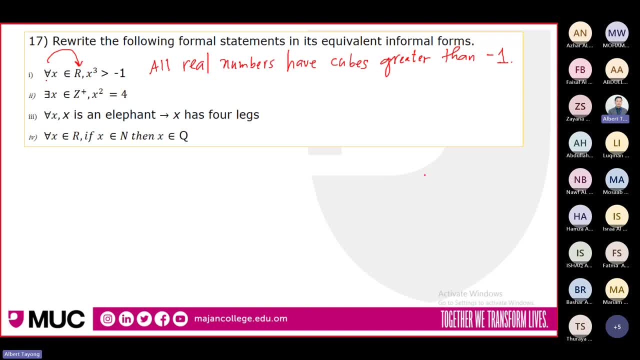 okay, okay, okay. so if you have x cube, so if you have x cube, so if you have x cube, say cubes, say cubes. x squared, say squares. of course. if you have four until infinity, use powers of four. if it is ten, you say powers of ten. it's usually only three and two have names because these are the most common ones. 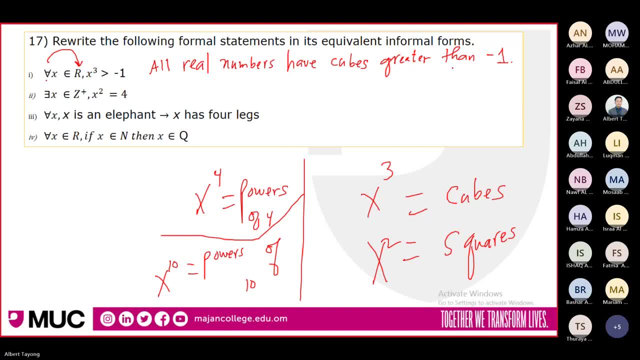 so all real numbers have cubes greater than negative one. you can also make it singular in your exam is up to you. this one is plural. okay, you can make it singular. how are you going to make this singular? this is plural singular. you will say every real number. 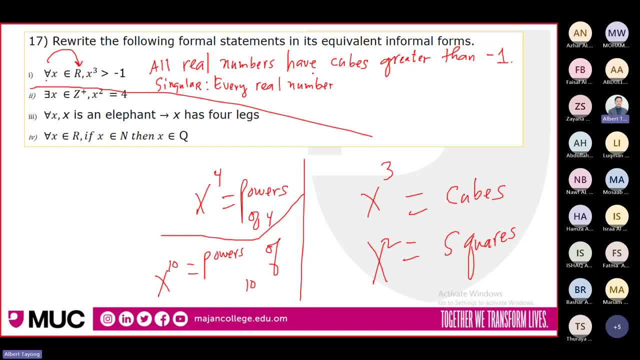 so numbers will become number, have will become has. cubes will become a cube greater than negative one. so this is also correct in your exam. it's up to you which one you're going to use. if you want to use the plural, you can use the plural. if you want to use singular, you can use singular. so all you can say. 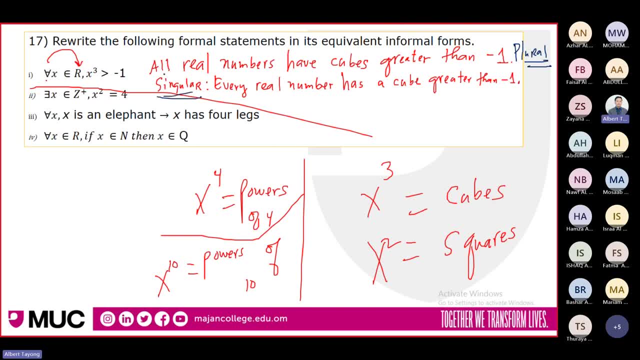 every real number. have will become has cubes will become a cube greater than negative one. okay, but it's easier to use the plural. all right, let's have now a little bit of a look at the real numbers. okay, let's have a look at the real numbers. 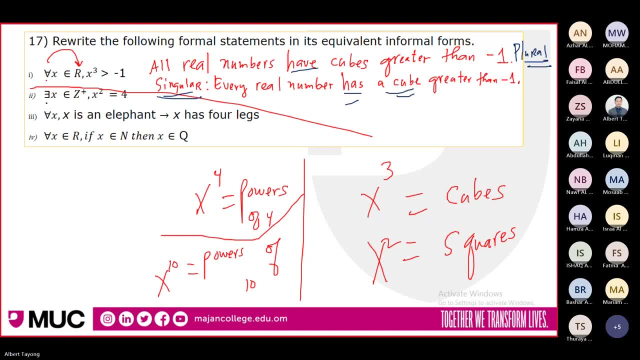 okay, let's have a look at the real numbers. number two: p p family family family. family family family is: is it is become become of, not the of it Quantifier. The keywords are some: There is a, There exists. There is at least one, There is at least one. 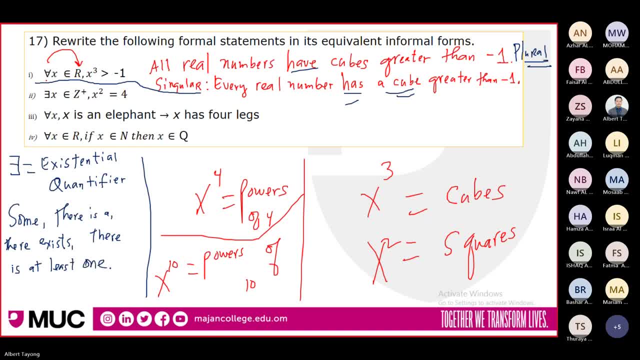 These are the keywords. It means at least one, But not all. Okay, for example, when you say some students, it means one or more, but not all In this. all real numbers, all Universal, Universal, We don't Exclude anything, Okay. so that's the difference. That's why it is called as existential, because at least one, but not all. 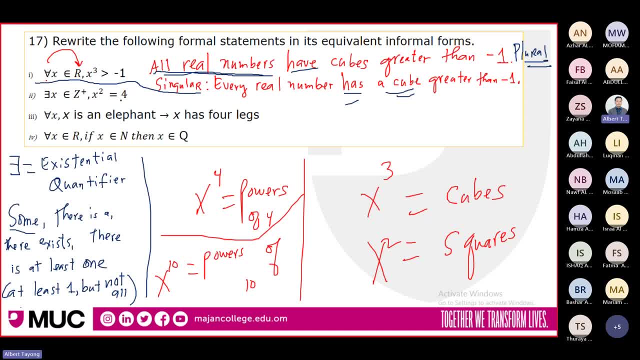 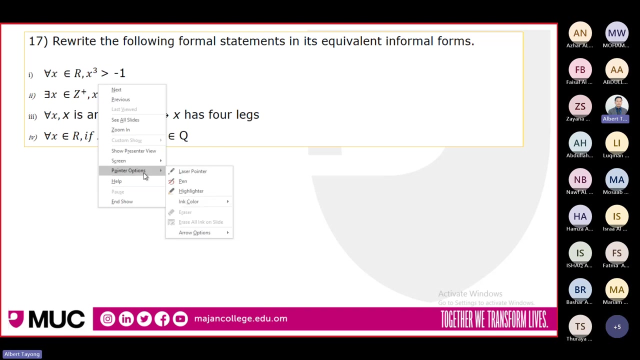 So let's answer number two. There exists x in z plus Comma x, squared equals four. So what does this mean? So you can use the plural, Or number two, you can use the plural if you want. Okay, so you can say some. Okay, so you can say some. 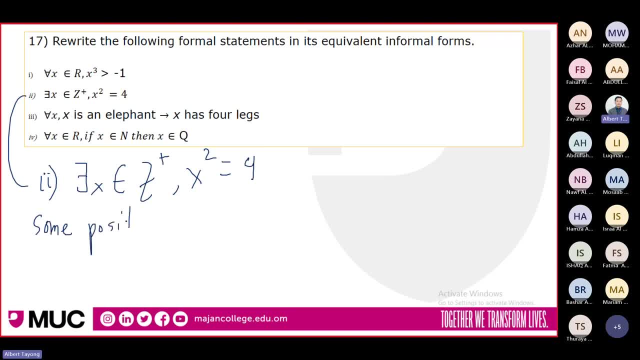 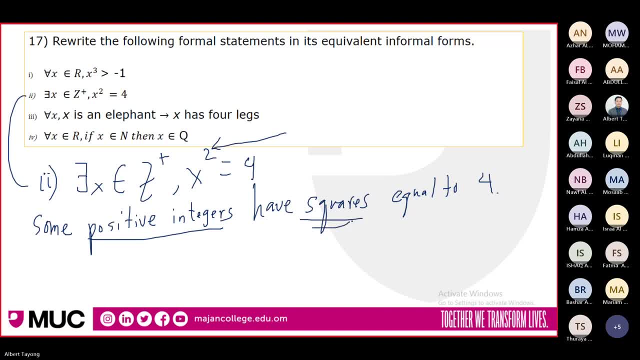 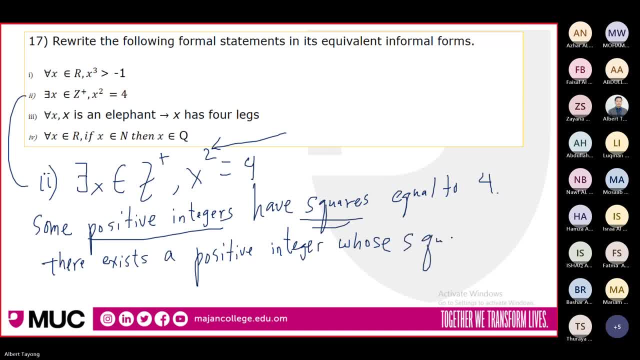 Half will become whose Whose square? Whose square Is equal to four. You see the difference. There exists a positive integer, Instead of saying positive integers. Half becomes whose Square is equal to four. Half becomes whose Square is equal to four. Okay, so any question here. 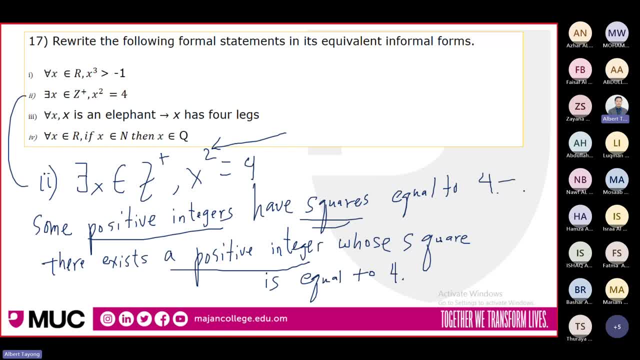 Guys, it's up to you Whether you want to answer Using the plural form Or You want to use the singular. Plural is. Plural is p-l-u-r-a-l. But don't waste your time In the test. Select only one, Whichever is more comfortable for you. 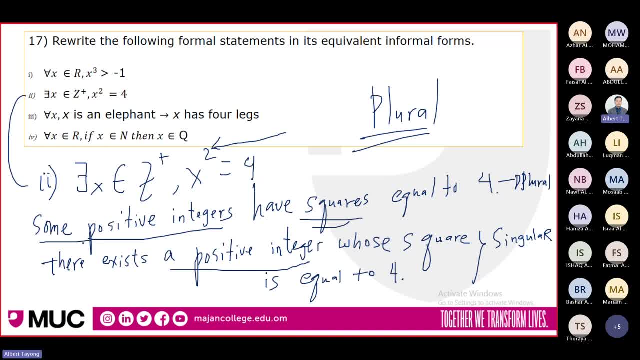 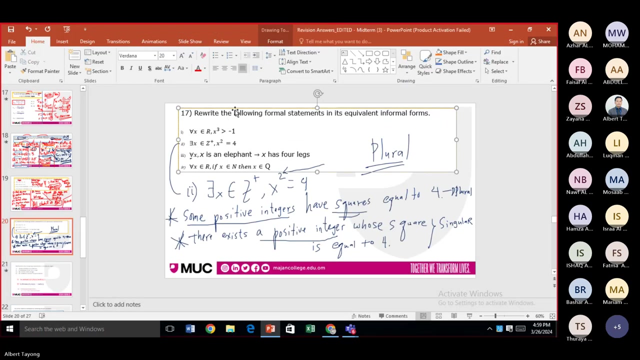 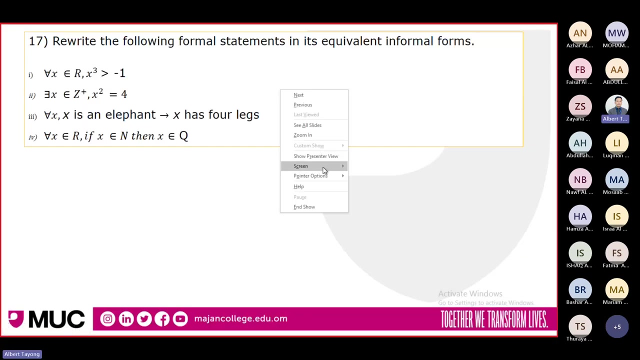 But, as I said, The plural is easier Compared to the singular, So let's have number three. Number three, The first symbol there is for all. So start with all, Or you can use every Okay, Okay, Number three. You can say All elephants. 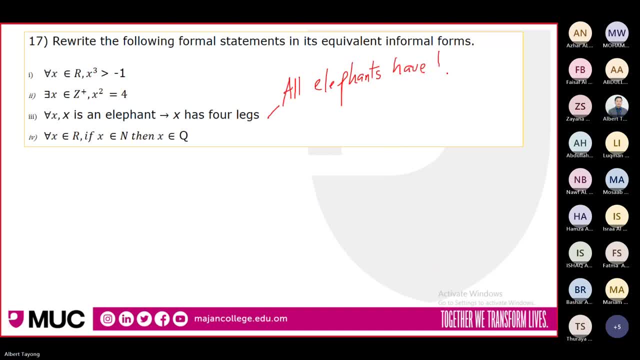 Have four legs. Or you can say: Every Elephant Has Four legs, Singular. Or, since we have this symbol, This symbol means If then. So you can use An if then statement. You can say: If It is an elephant. 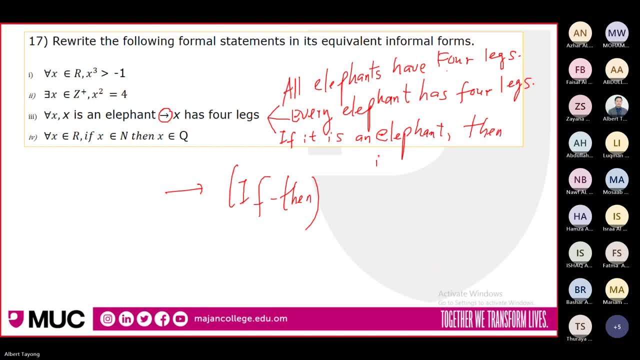 Then It has Four Legs, So this one is also correct Because of this symbol. As I said, the easiest one is the plural: All elephants have four legs, Or every elephant has four legs, So have Becomes has. 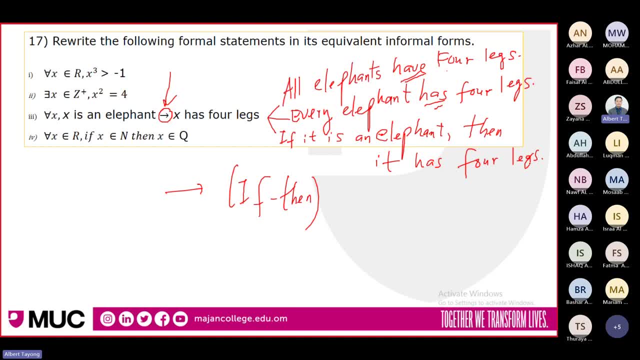 Or we say: if it is an elephant, Then It has four legs. So whenever you use If statement, It will become universal. Okay, When you say If a student, When you say if a student, It means every student. 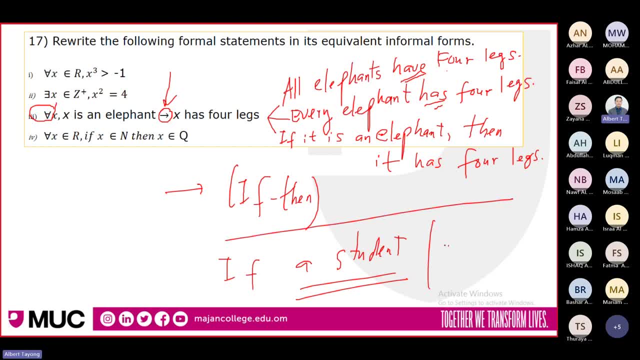 All students. Okay, This means all students, Because you are assuming You are using the if here Conditional And then Are here It's like every Or each student. So if Will change the statement to Universal If. 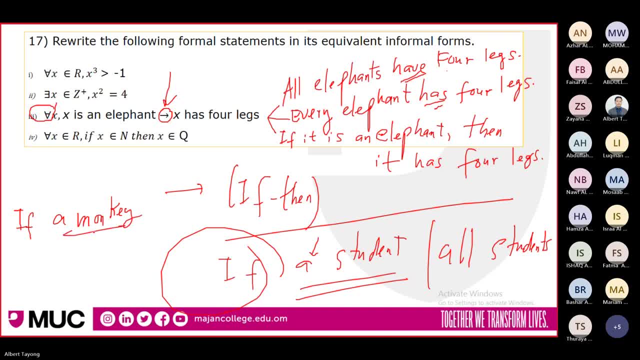 A monkey. This is not only one monkey, Although I hear means one Because of if, It includes all monkeys in the world. If a monkey means Every monkey Because of if. If you're going to remove, If a monkey has only one monkey, 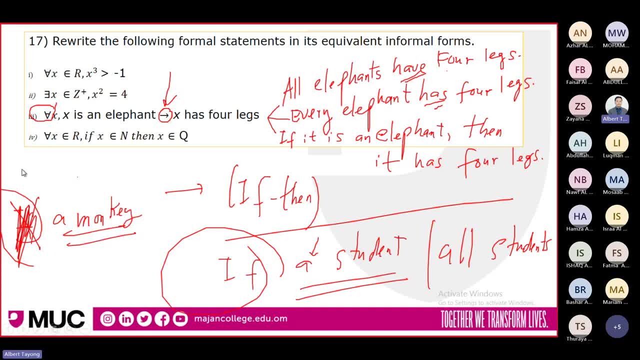 Okay, So if we'll change the statement, You say: if, If a man, So it includes every man Because of the if So here, if it is an elephant, then it has four legs. It includes all the elephants Because two of them are independent animals. 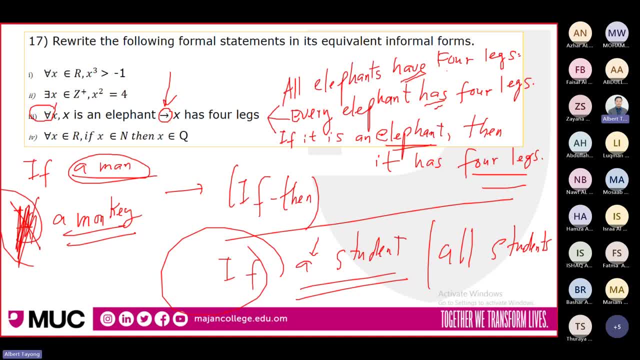 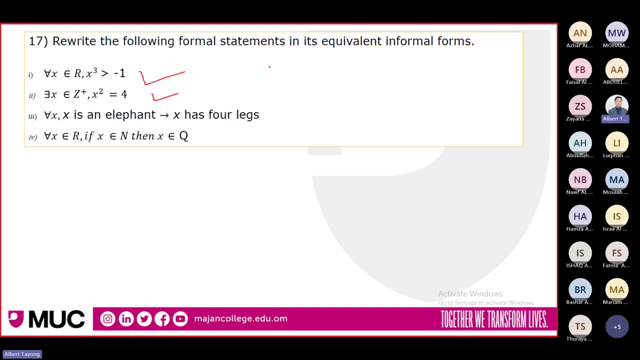 So it includes all the animals in the planet. And if you want to see A, So One, Two, One, Four, One. are you still there? yes, yes, did you understand? one, two, three, yes, yes, okay, here the if is inside. we have three variables. we have the R, N and Q. we have 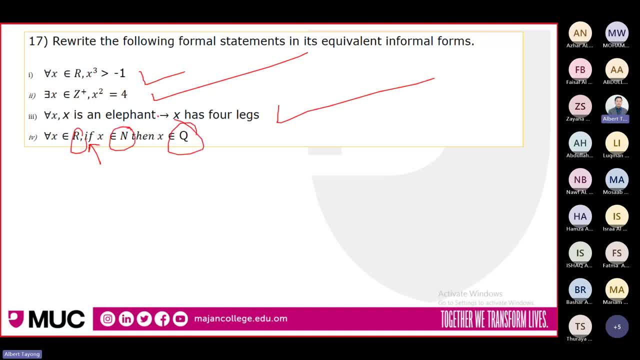 our N and Q. so if we are talking about three things like here, we have our N, Q and we have if in the middle, we have to start with the if comma, here X. so there are three variables here. R and Q start with F always, so you start with F. 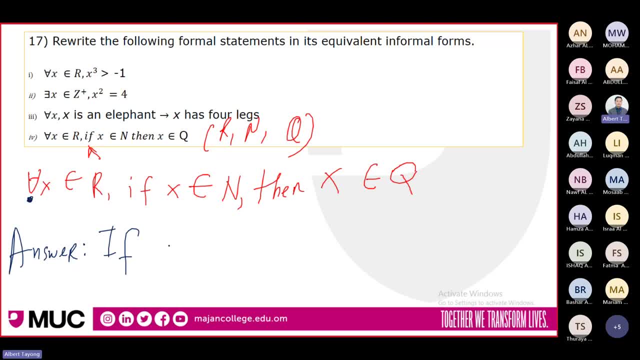 then this one. as I said, when you use if, ah, it will be all. if a real number, so go to the left. so start from here, then go to the left, then go to the right. so if a real number is a number, natural number, that's the end. 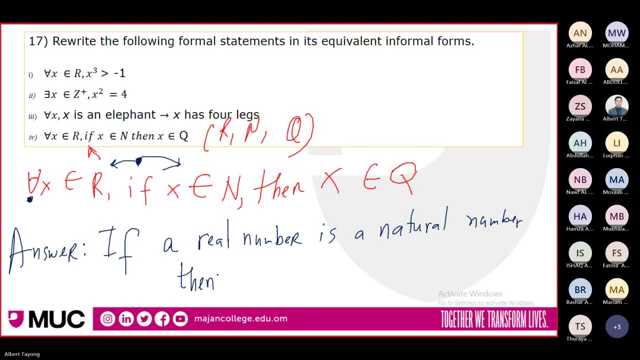 then it is a rational number. Rational number is the Q. okay, this is RA. so this is the answer: rational number, real number, natural number is for the N, this is for the Q, this is for the R. so again we have to start. 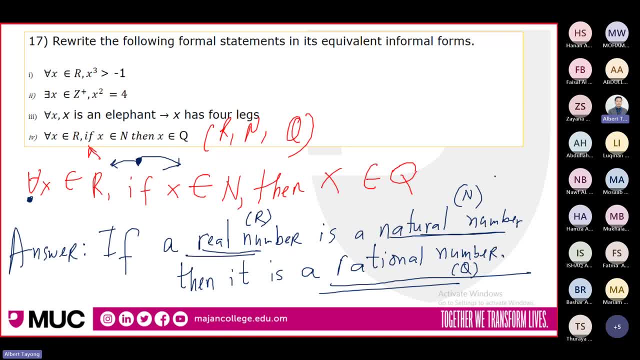 from: if go to the left, then go to the right. so if a real number is a natural number, then it is a rational number, the Q, Okay, Okay. so this is how to change from symbolic to English sentence. informal, as I said, is English. 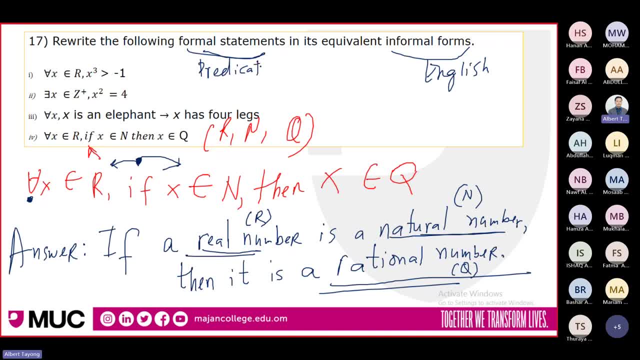 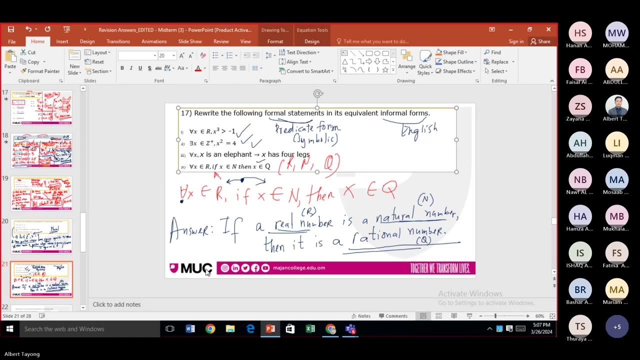 formal is the predicate form, the symbolic form. okay, these are symbolic. Okay, so this is how to change from symbolic to English sentence. informal, as I said, is English. it changes to English statements. Okay, is this clear? 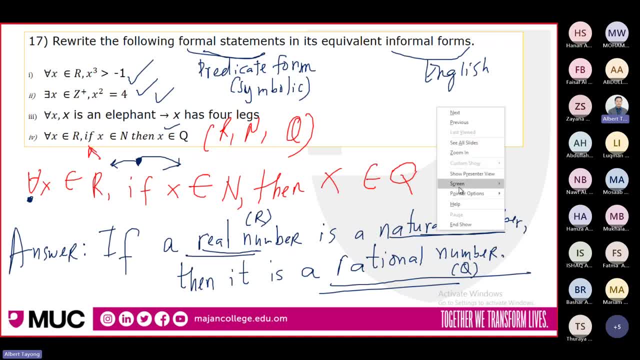 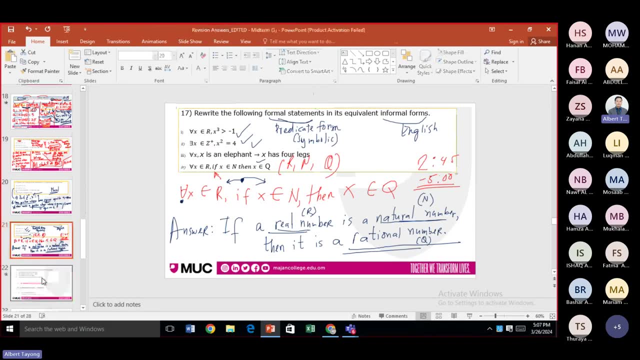 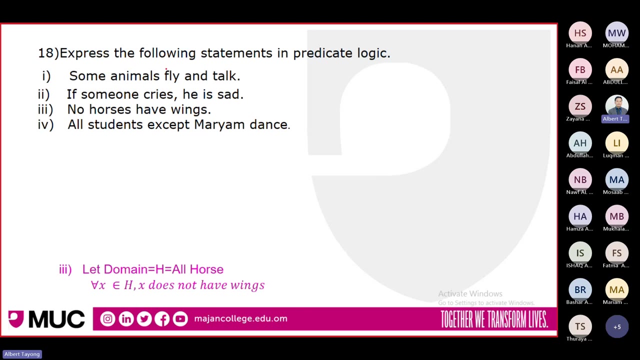 We'll have more examples of this during the support class on Thursday, 2.45 to 5, after tomorrow. now the 18 is the opposite. opposite. this is, we change the statements to predicate logic, to symbolic, whenever you see the word predicate logic, predicate form, symbolic. 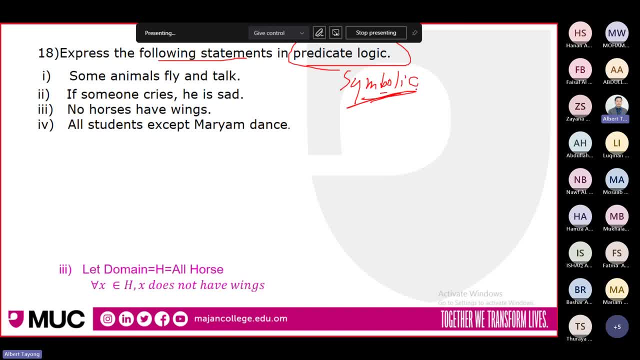 so whenever you see the word some, somebody, someone there exists, you're going to use this symbol automatically. okay, it means at least one, but not all like here's somebody. some animals fly and talk: it means at least one, but not all animals. not all animals fly and talk. in fact, i discovered only one. 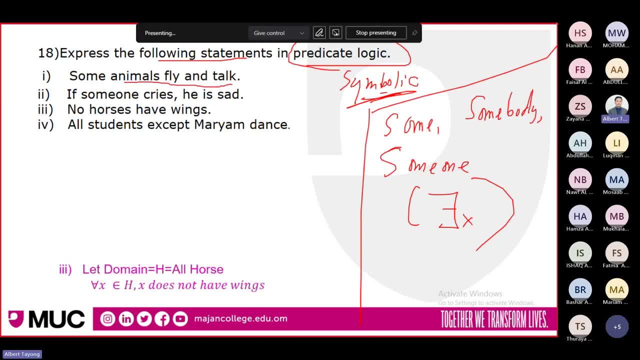 maybe there are some, but i know only one animal that fly and talk. what is it? what is that animal? the parrot's right. so first you have to identify the domain. every time you change from english english to symbolic, find the domain. first domain is the subject, what we are talking about. 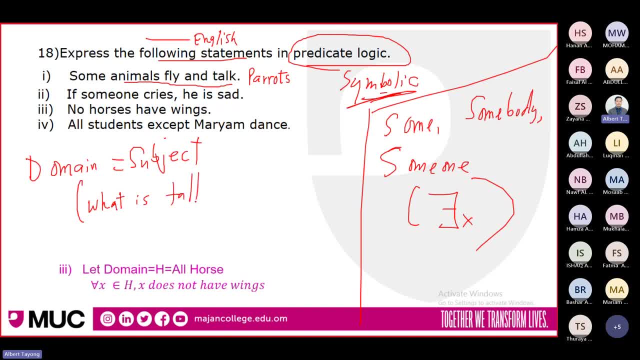 okay, what is talked about. so what are we talking about here? we talk about animals. that is your domain. okay, we say: all students, students are the domain, so you have to know what is the subject, what we talked about. we call it as the domain, so so that means your domain will be. 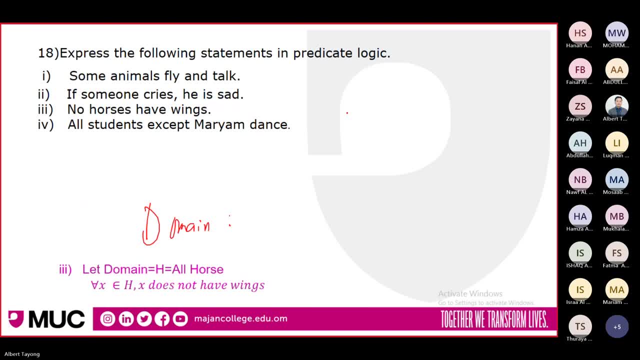 x is an animal like this: when you specify your domain, you start from the inside, go to the left. it's like how you write in arabic: from right to left. x- here is any animal. you can use any letter, but the most common is x. but, as i said, this is any letter here. 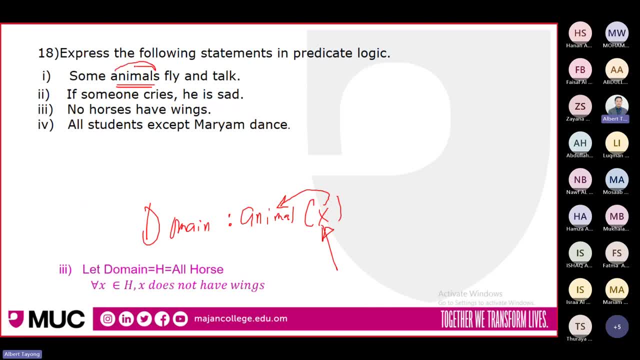 because we don't know what animals are. this it's not mentioned in the problem. we say some. this is the quantifier. it tells us how many. quantifier means it gives us like the count: is it all, or at least one? that's the meaning of quantifier from the word quantity. 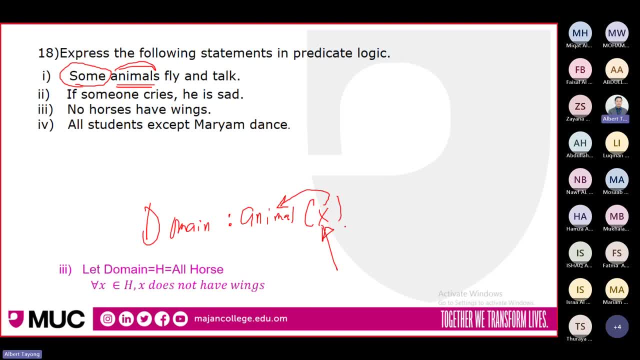 sum, so at least one, so x. here is any any element, part of the domain. so our answer will be like this: x is any animal. and then here we are going to put our domain x is an animal. as i said, we start from here and then we are going to nerves. sorry for this. 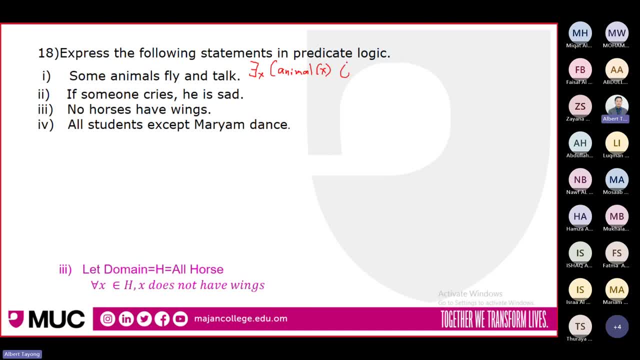 ablation, but here go to the left. then we connect using the and symbol because we have here our predicate. the last part is the predicate some animals. that's our subject. this is what we are talking about. our domain is animals, so fly and talk is part of the predicate. that is after. 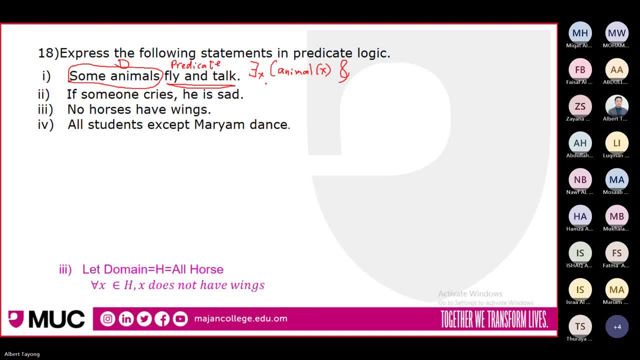 and so it means some animals, or there exists an animal such that this animal fly and talk. okay, so there exists, so this there exists. or some animals fly, so x is animal, x flies. you start reading from inside, go to the left, then x talks. but we use the base form of the verb. 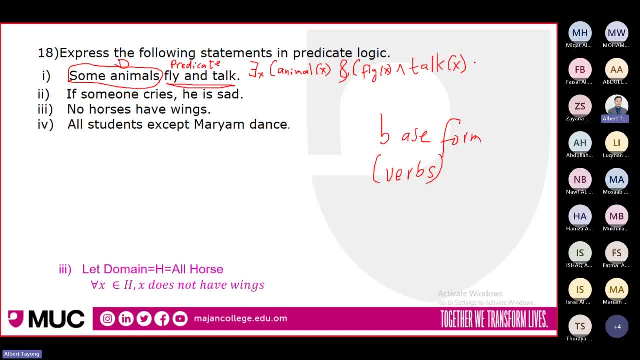 what's the meaning of base form, the original form of the verbs base form. okay, and here we have to close this. so we have to close it here and here. and the first also we have to close this one we have open here before fly, so we have to close towards the end. 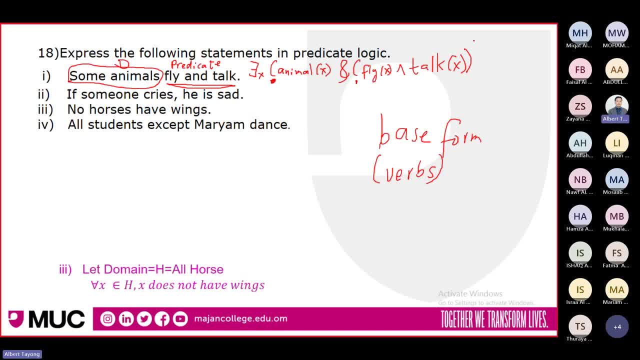 and we have here open before animal, you have to close towards the end. so every parentheses that you open you have to close it towards the end. this first close parenthesis is for x, Second one is for this And the third one is for the first one. 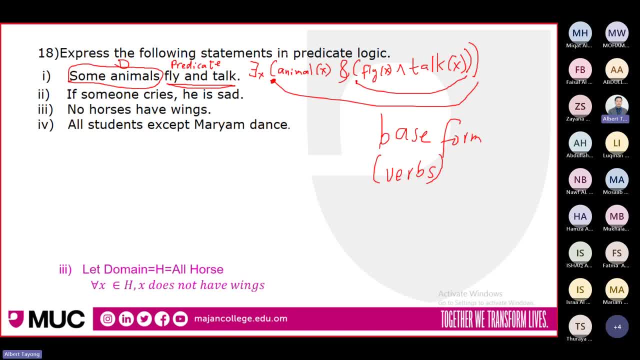 So if you're going to read from left to right, some animals fly and talk. So that is the answer. Please try to answer number two. If someone cries, he is sad Guys, we don't care whether it is true or false. 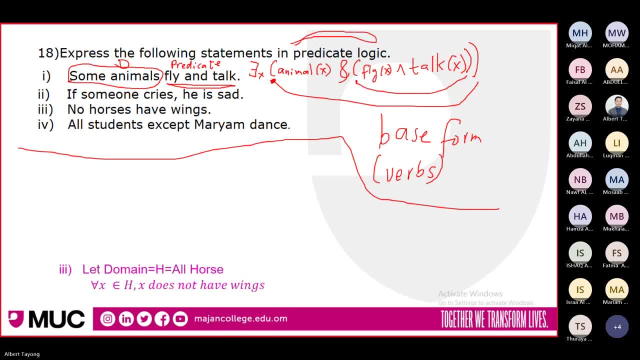 We are only changing the symbolic form. Yeah, so we don't care whether this is true. If someone cries, he is sad. Some people, they cry, but they are not sad. Okay, so number two: If someone cries, he is sad. 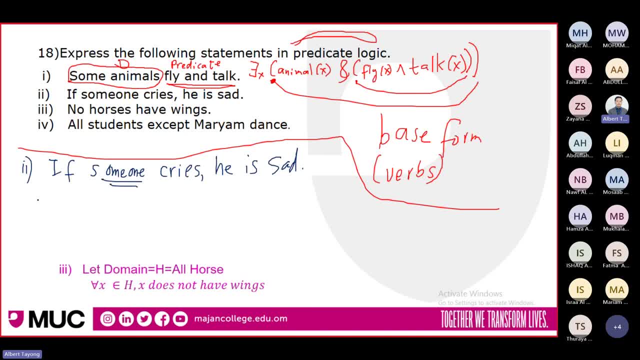 So, as I said, someone, some, you will use this symbol immediately. Okay, and there is, if here, So someone, you have to define that X is a person, Because in logic, someone could be anything. Okay, don't forget, someone here means: 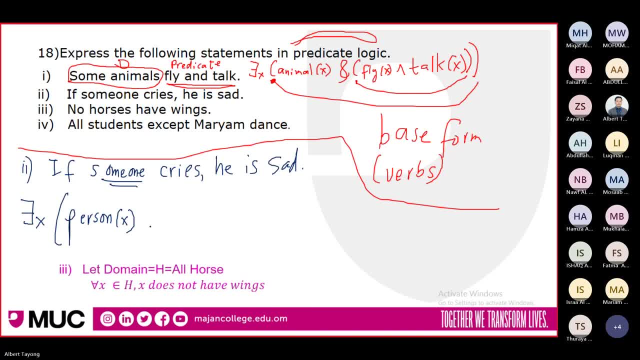 the domain is a person And we have cry. Okay, so we don't use cries. You have to use the base form of the verb. Cries comes from the word cry. The comma here has the word then. So then He is sad. 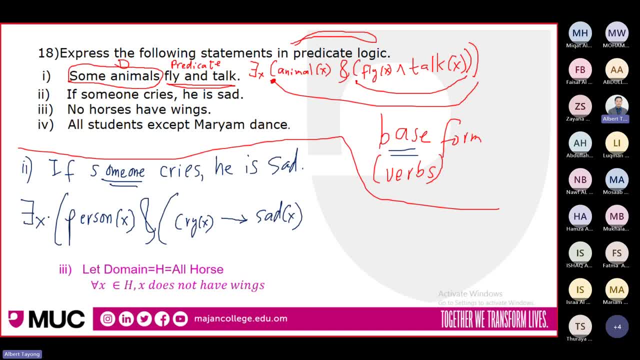 X is sad. So X here is any person, This one after E, X. As I said, this X can be any variable. You can use M, you can use N, any letter, So the X here is a person. So that person if he cries, then he is sad. 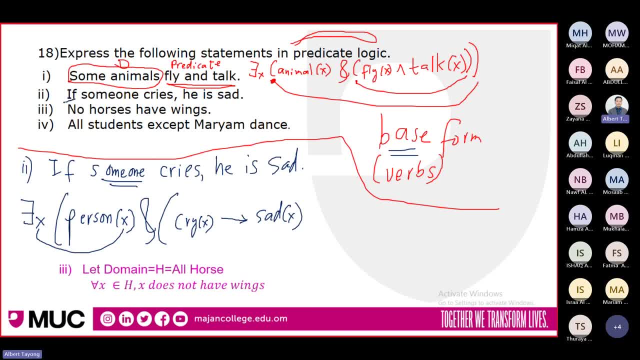 So we have to use M. And now, if we have a letter, we will use this symbol And we will use it to describe the person. So we will use it to describe the person. So we have to use this symbol in the first. 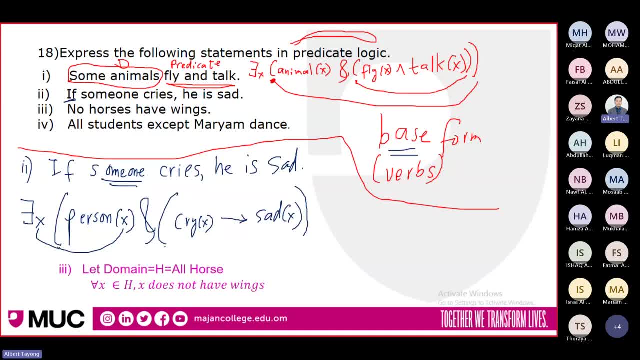 So we have 2,, 3,, 4,, 5,, 6,, 7,, 8,, 9,, 10,, 11,, 12,, 13,, 14,, 15,, 16,, 17,, 18,, 19,, 20,, 21,, 22,, 23,, 24,, 25,, 26,, 27,, 28,, 29,, 28,, 30,, 31,, 32,, 33,, 32,, 33,, 32,, 34,, 34,, 35,, 36,, 37,, 38,, 38,, 39,, 40,, 41,, 42. 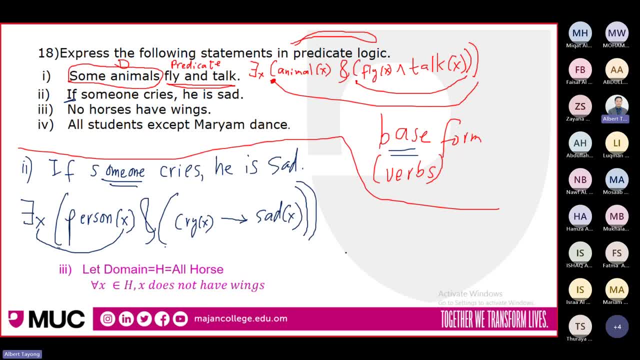 So you have three close parenthesis towards the end. We will just answer number 3 and 4, then we will go. We'll extend a little bit for five minutes. It's time already. Number 3 and 4, I'm going to answer for five minutes. 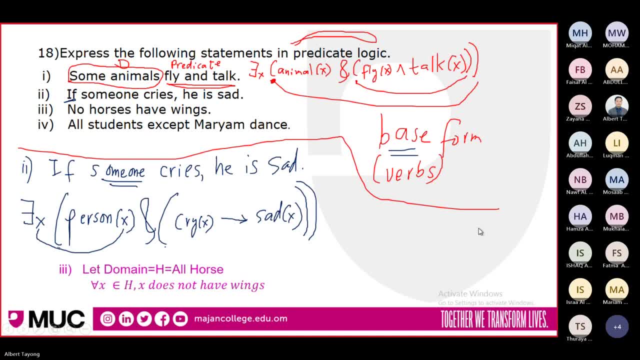 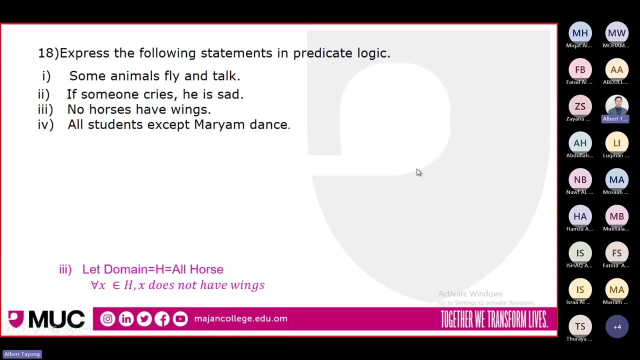 Guys, do you have any question here? Any question? No, Okay, Let's have number 3.. No horses have wings. What's the meaning of no horses have wings? Let's say no horses have wings, It means all horses does not have wings. 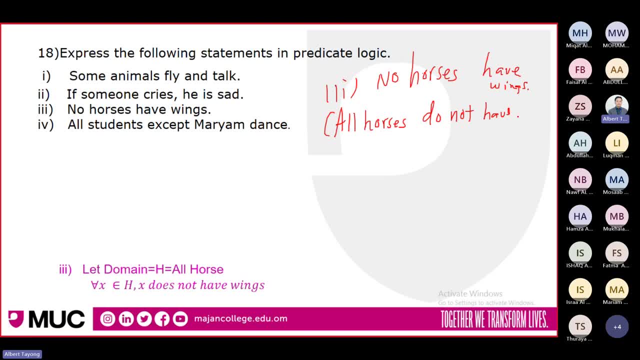 Do not have wings. So in the exam the first step is to change to all Okay. Whenever you the word no, first step is change to all okay. and then you define let h equals set of all horses. so you have to define the domain. this is the domain, what we talk about: horses. 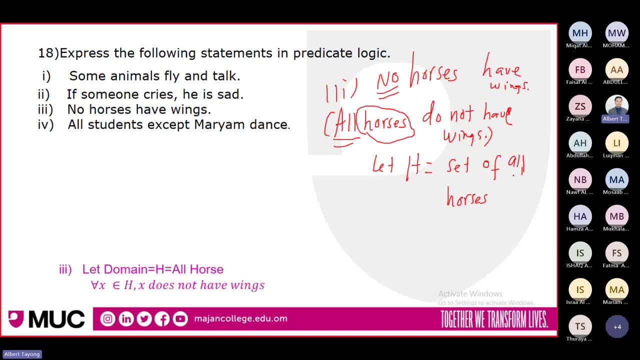 so set of all horses is h. you use the first letter or you can use your own letters. okay, so the answer will be all here. so we have this symbol, small x here. below is any horse. please take note that the x here is part of the domain this. 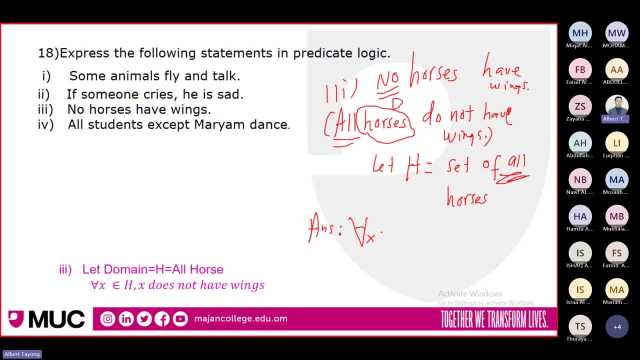 is our domain. x is any horse in h. okay, for all. x in h, that means all horses. comma. then use this letter here: x does not have wings, okay, do not have wings, becomes does not have wings because x. x here is like every. every horse does not have wings, okay, so always. this is singular here after x. 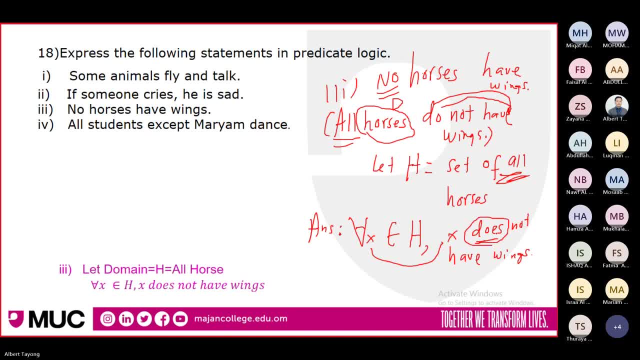 so this is the answer. so this is the answer. so this is the answer. okay, so for all x in because all horses. so for all x in h comma. x does not have wings. that's the predicate. the predicate is: do not have wings. the last one: all students except mariam. i want you to answer this homework. 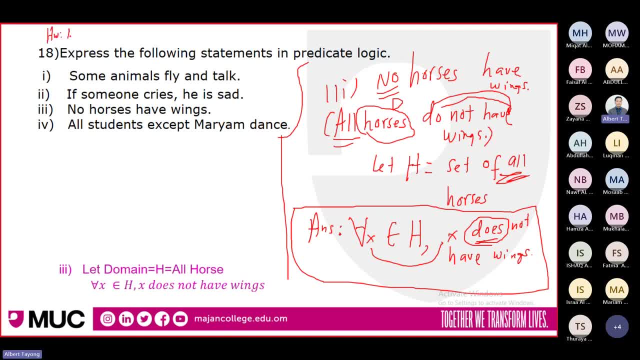 no students fail in this homework. no students fail in this homework. no students fail in this homework. no students failed in lpss. no students failed in lpss. so try this as your homework. first step is to change to all. first step is to change to all. no students failed in. what's the meaning?